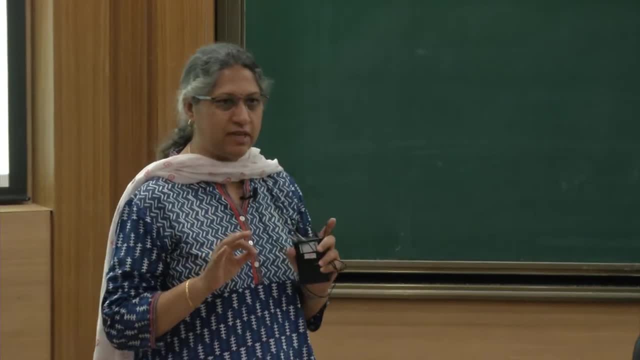 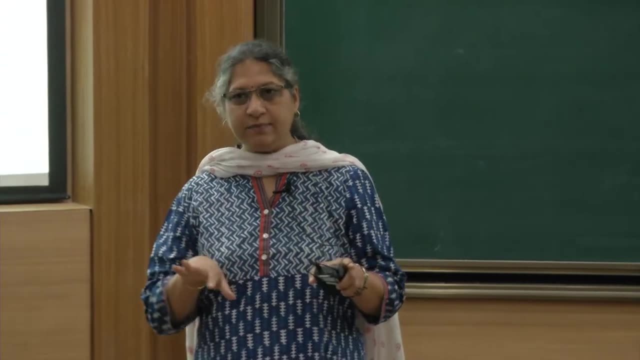 But anyway, the net result of any observation is that you have a lot of data that you need to analyse and get science out of it right. So to do that, there are certain steps that you need to do to get some meaningful results out of your data. 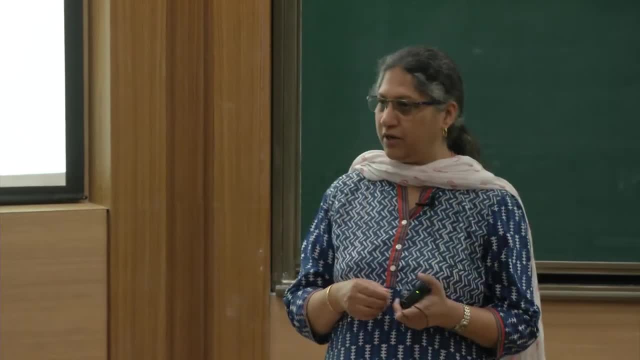 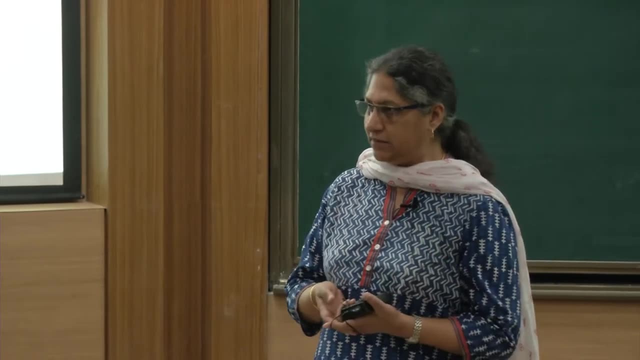 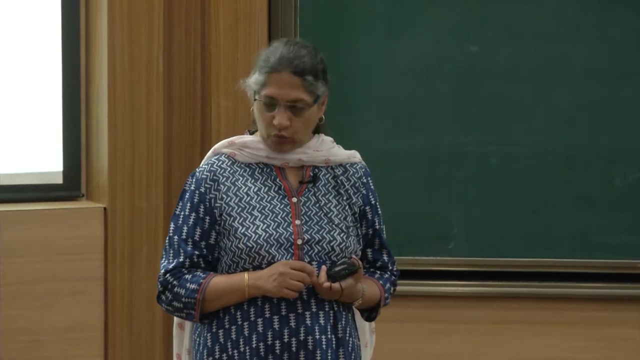 And today, much of our- you know today's sessions are all connected with what you do with the data and how you would ultimately get some meaningful results out of your data. Let me start the first steps that we have to do with any data. 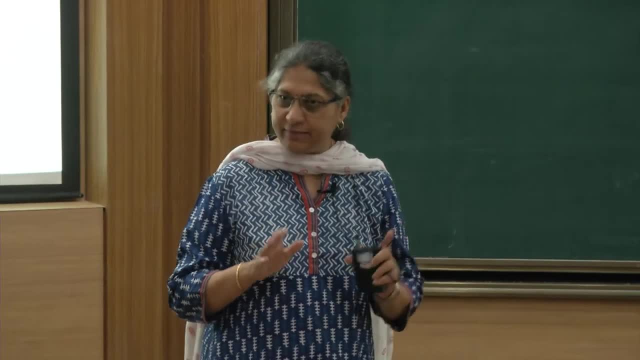 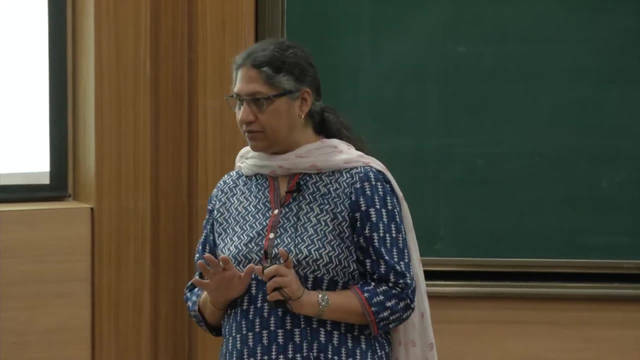 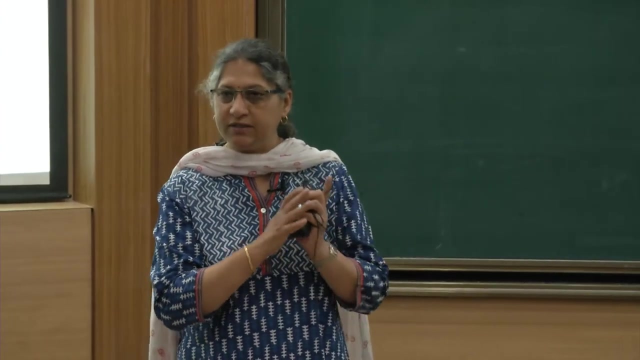 And I'm going to concentrate on the image data. that is essentially what we do for the use for photometry. I'm not going to talk about spectroscopic data right now, But much of what we do for this image, image data- is also something that we do in spectroscopy. okay, 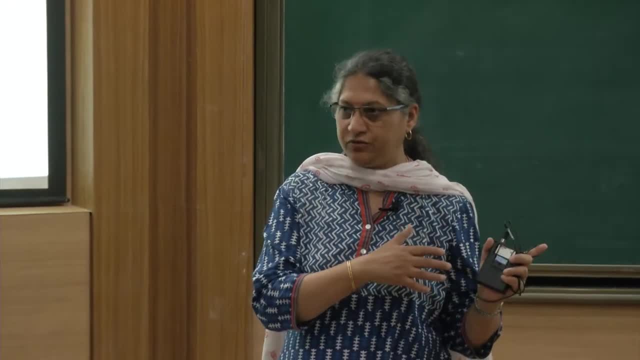 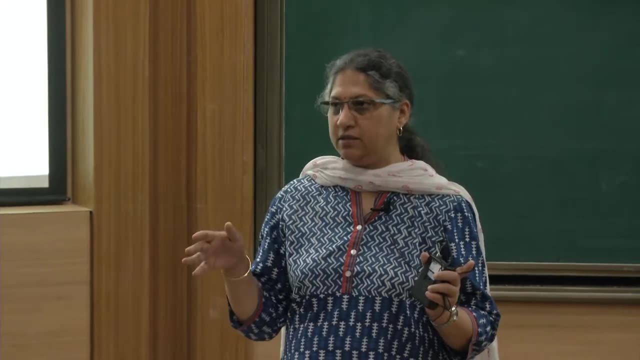 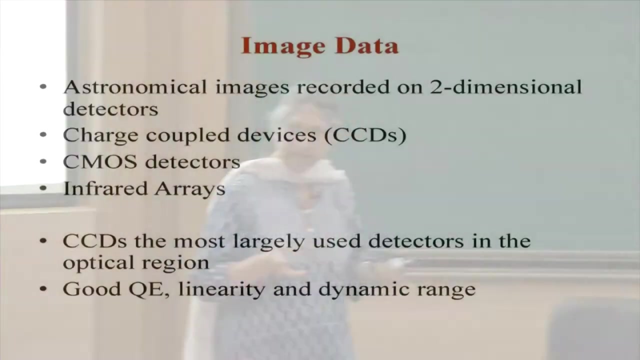 So, whatever I'm going to tell you now, a good fraction of it, majority of the steps are what you'd initially do, even for the spectroscopic data, before you go to actually analysing the spectrum. okay, So what is image data? It is essentially the astronomical images. 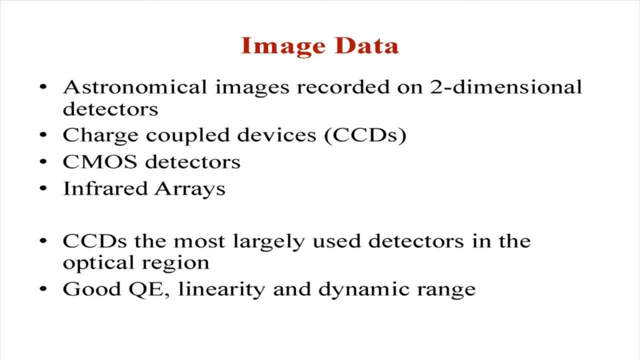 It is a portion of the sky which is recorded on your detector. There is a two-dimensional detectors And some of the most commonly used detectors are the charge coupled devices, the CMOS detectors and the infrared arrays to observe in the infrared region. CCDs are, you know, by far the most largely used detectors in astronomy. 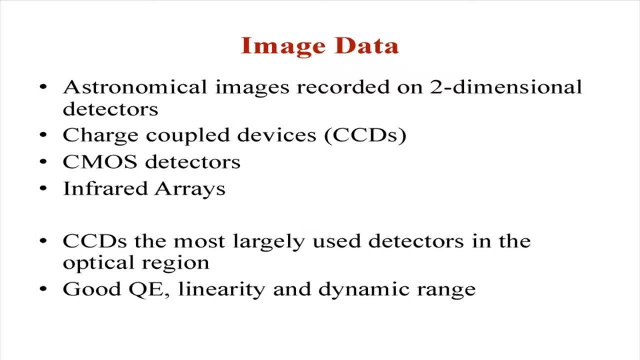 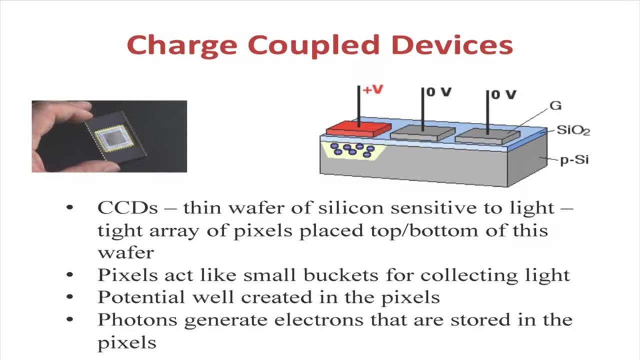 And some of the main advantages of using CCDs are that it has a good quantum efficiency, good linearity and a good dynamic range, all of which we want in any astronomical instrument. Okay, So just a few slides on what charge coupled devices are. 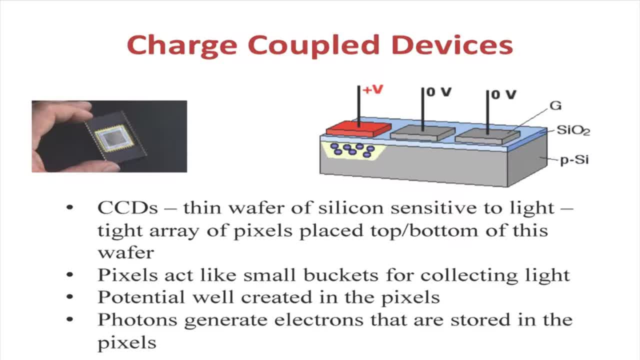 for people who don't know, these- You, you know, have the CMOS detectors are what, by and large, are used in the digital cameras and in your mobile phones to a certain extent, But what we use, by and large in astronomy are the charge coupled devices. 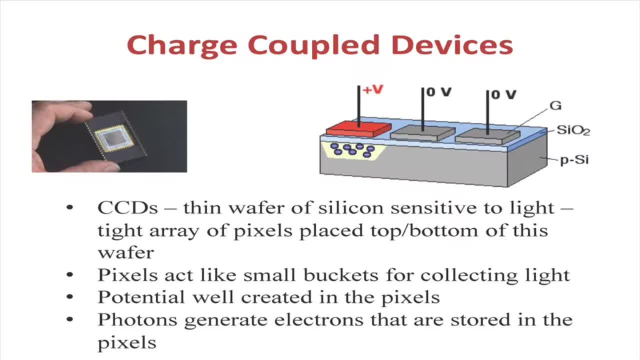 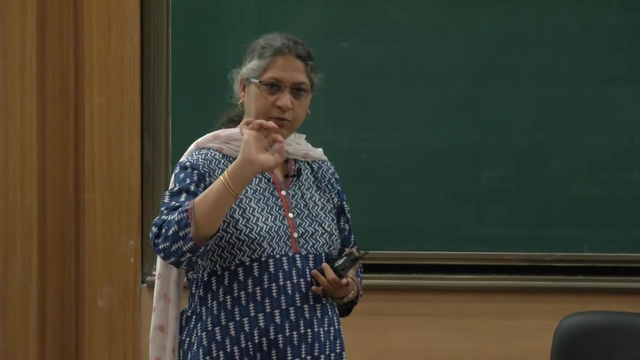 So these are, you know, nothing but silicon, silicon based arrays, where you have these pixels, or the pixel that is a light collecting element in the CCD, which acts like buckets, small buckets of you know light collecting buckets, basically Okay, So what happens is that in these pixels there is a potential well, which is created. 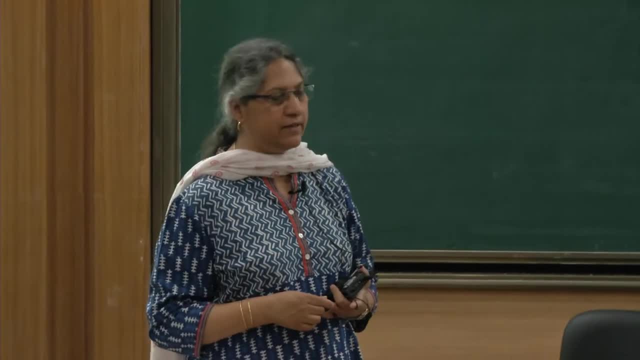 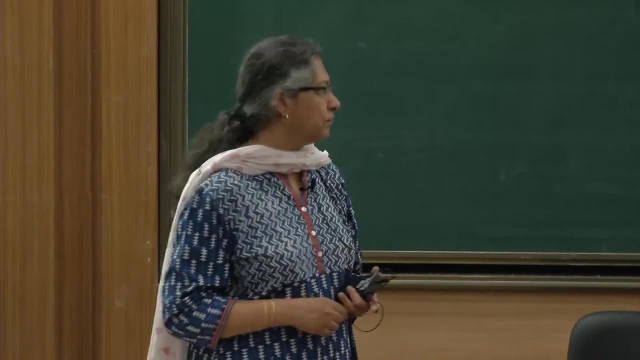 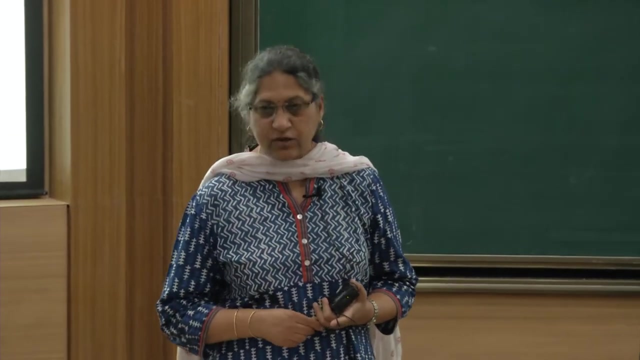 where the electrons are stored And these electrons are generated. when a photon strikes, Okay, Where the photoelectric effect, which all of you know. So this is how the electrons are generated and these are stored in the pixel. So, having been stored in the pixel, you need to read out these electrons. 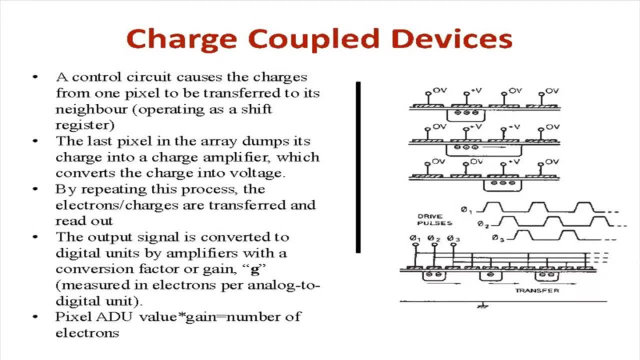 Right. So what is done is that you you have a circuit which essentially allows in reading out the electrons. So when you have this potential, well created the, the region of the pixel which has the most positive voltage, that is where the electrons are stored. 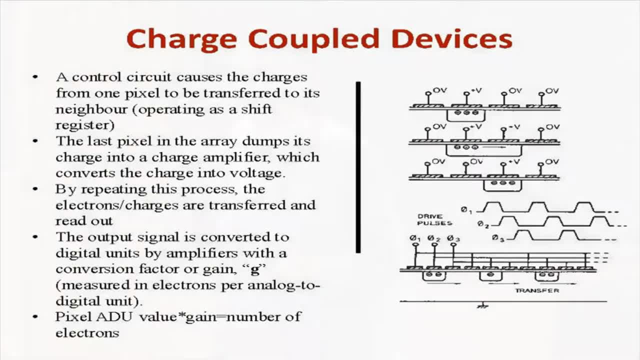 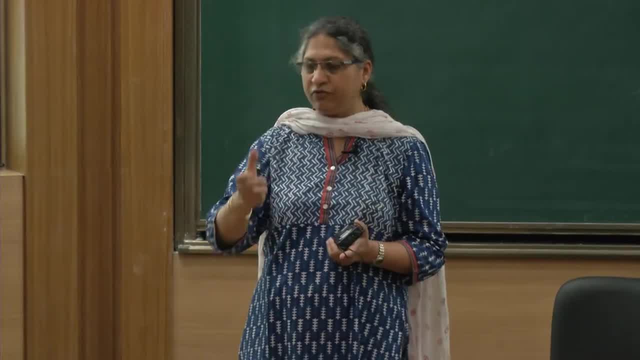 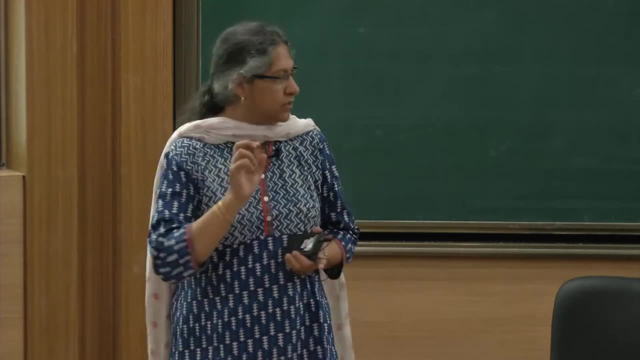 Then you have to read off. So this is done by a clocking sequence where the adjacent pixel, you make that more positive, So the electrons move from where it is collected to the more positive region. So you keep doing it sequentially. Okay, So the CCD has. it is a two dimensional detector. 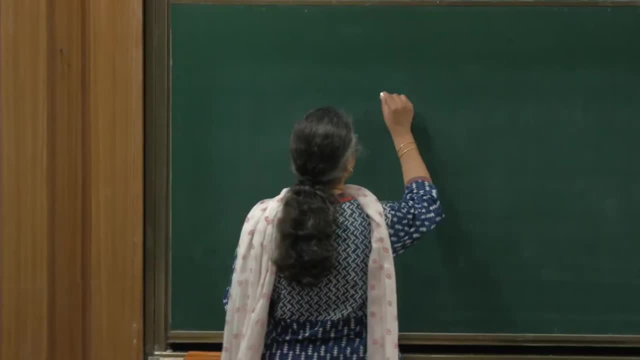 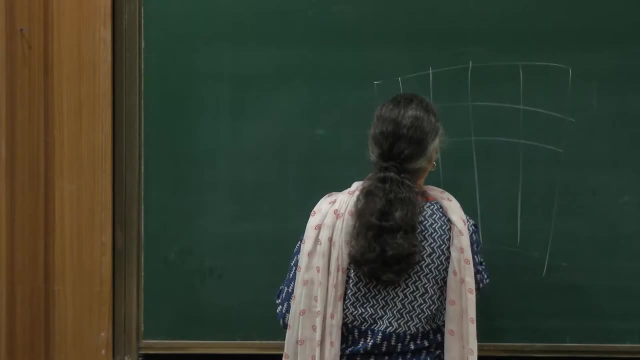 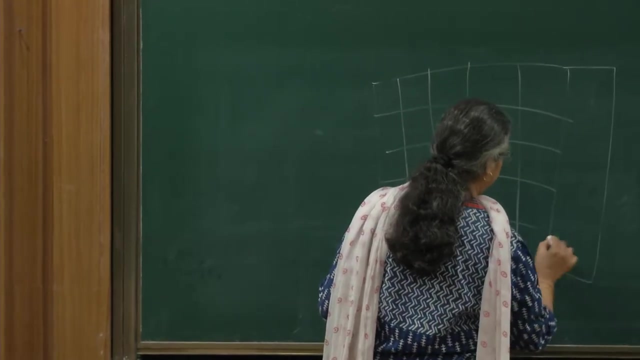 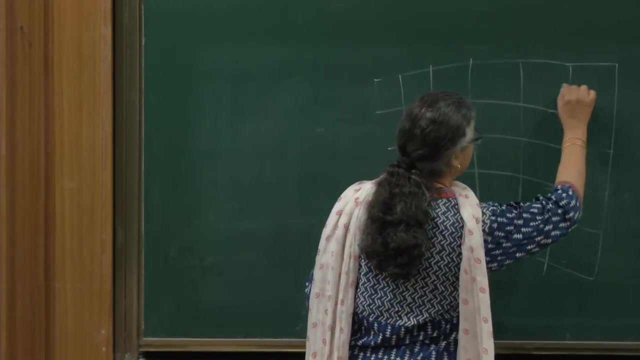 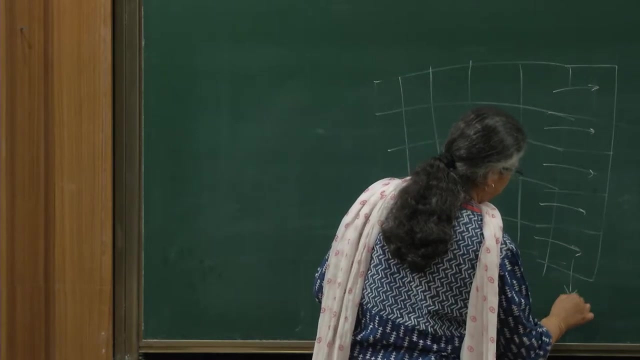 So you have these rows and columns, Okay, So basically, what you do is you have one column here, which is the readout column, So you read the rows. So, for example, along each row the charge is transferred here, Right, And the charge gets transferred sequentially this way: 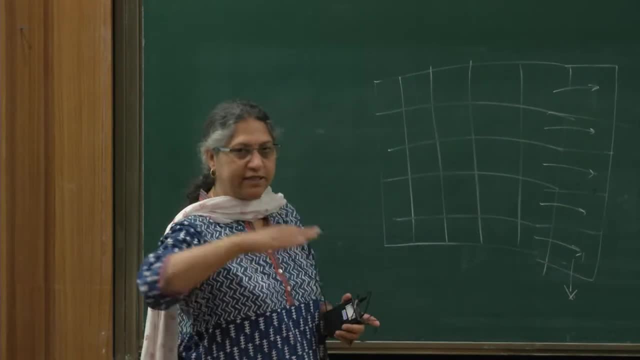 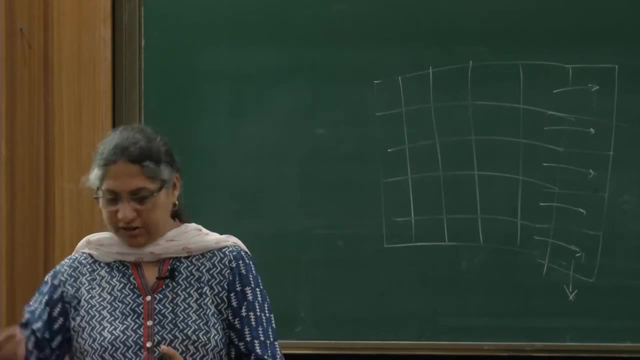 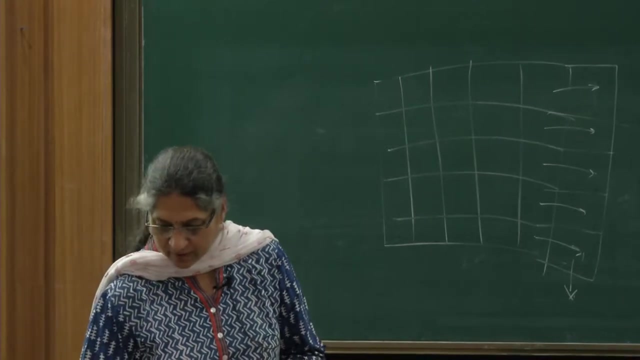 Okay, So you keep reading off each pixel. It keeps getting transferred from one pixel to the other, And that is why you are calling it as a charge coupled devices, Because it is not read off from each pixel but it is, you know, transferred to another pixel and it is read off. 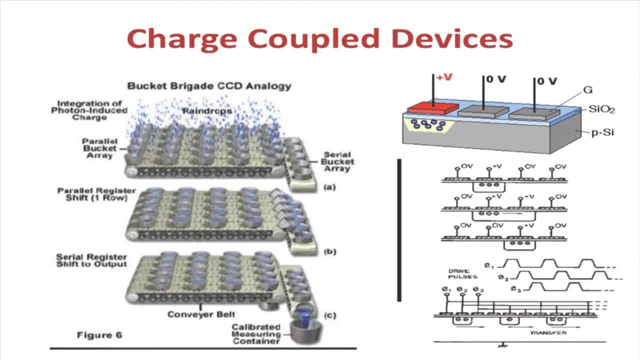 The most used analogy for you know how to understand how the pixels are read out is What is generally used, is the what is called, as you know, collecting the rain water in bucket. So you can look at each pixel as a bucket which is collecting water and then you know, essentially, tip off this bucket first. 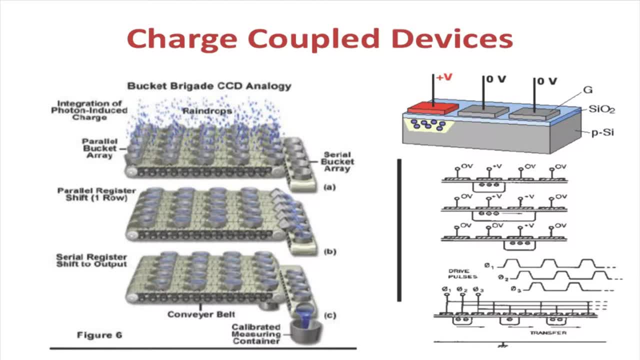 So this gets emptied. So to you know: initially these buckets are all empty, So what you do is you tip off this into this. You know it goes like that. Then you tip off this, Empty this into this, So you read this: 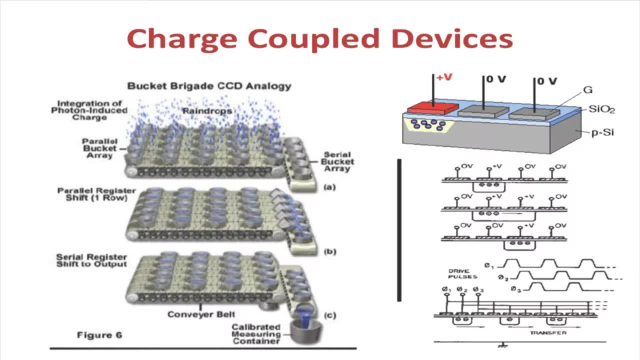 Okay, So you keep shifting. It is like a shift register- You keep shifting the charges and you read them off. So what you are reading of the charges is like you are reading of the voltage and that you need to convert into a digital form. 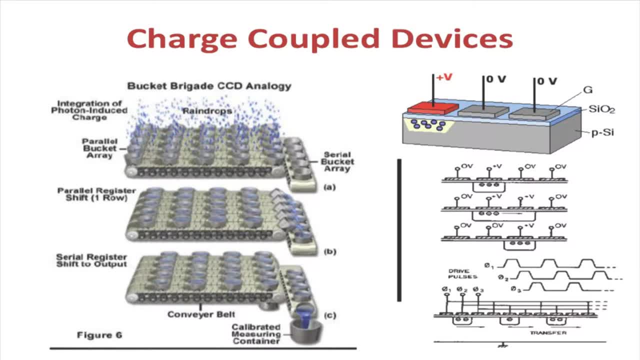 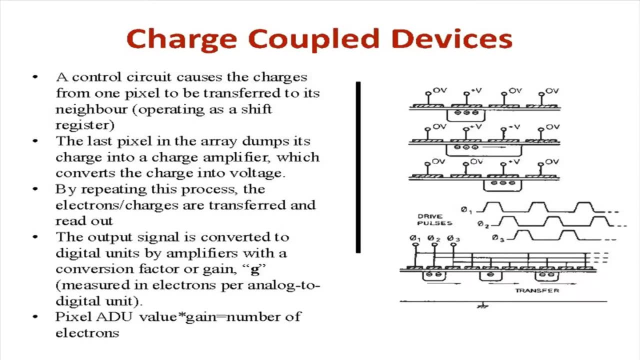 And that is what we call as the counts. So essentially there are these amplifiers which convert the readout. electronics Converts the voltage into the digital form And the amplifiers are there which, will you know kind of there is a gain given so that you have the voltage can be easily read off. 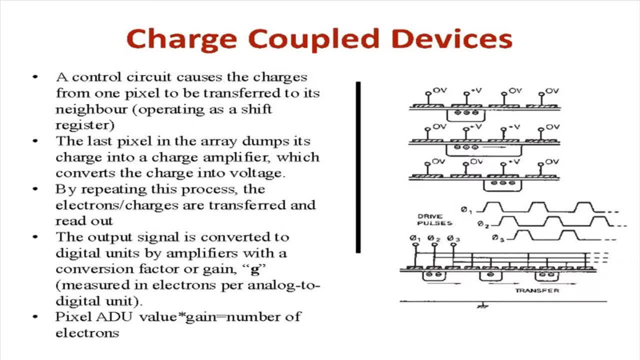 And what is of importance here is what we call as the analog to digital unit, So which is nothing but a reflection of the amount of electrons which are collected, Which, in turn, is a reflection of the photons or the flux that has been received from the astronomical source. 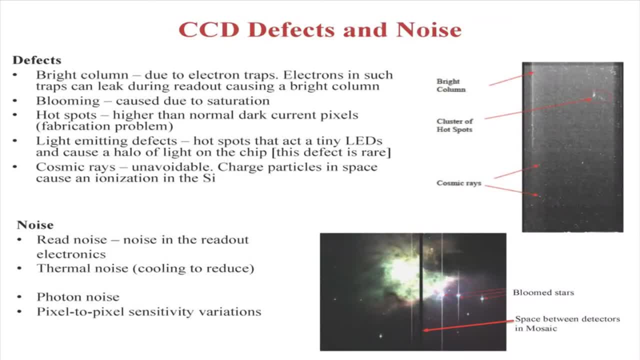 Okay, To use any detector. there are lot of things that we need to understand, certain characteristics about the detector, And it is extremely important to know what are the defects that you can expect in such a detector. Okay, So there are various defects that you can expect. 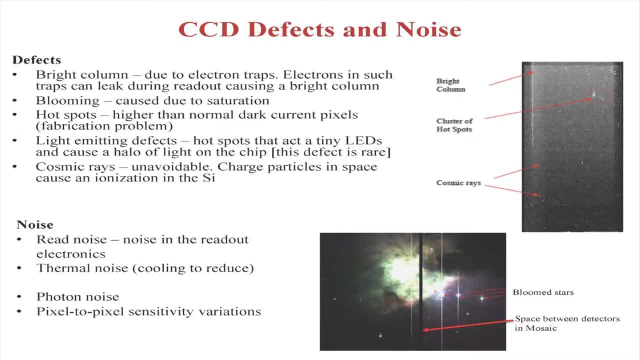 Okay, That you can expect in a in a CCD One is: you find there are some bright columns or you know, bright row and bright spots in the CCD, Even without it having been exposed to any astronomical source, And some of these like the bright columns. they are caused due to the electron traps, which is you know. 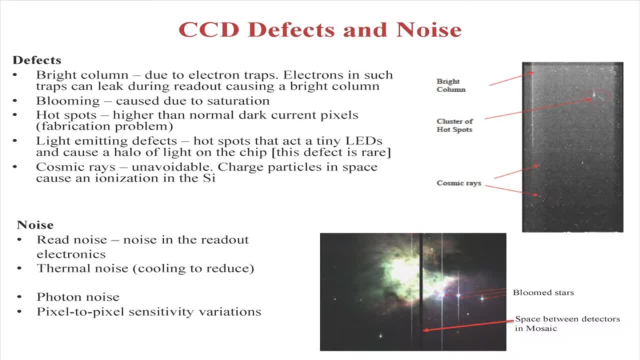 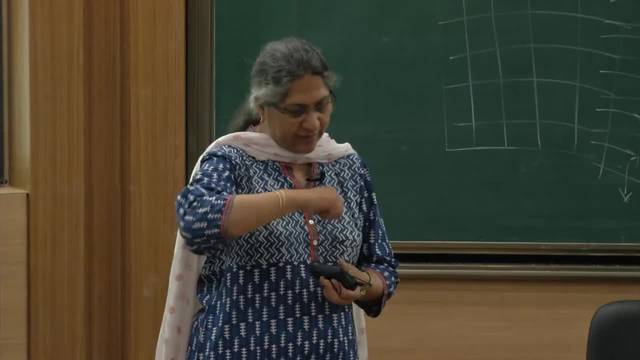 So when there are some electrons trapped in certain columns when you you know it can leak out when you are reading Reading the thing, and so it kind of it. it leaves a trail behind in the column. Okay, So these are called the bright columns. 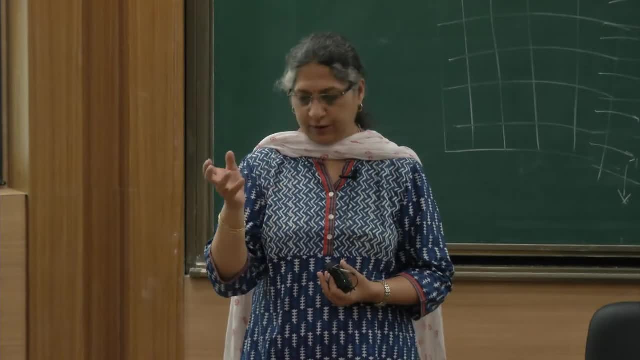 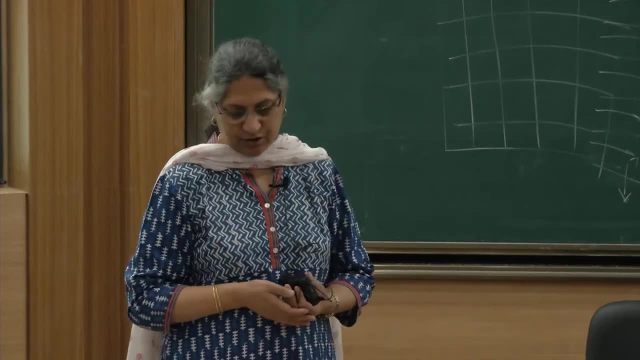 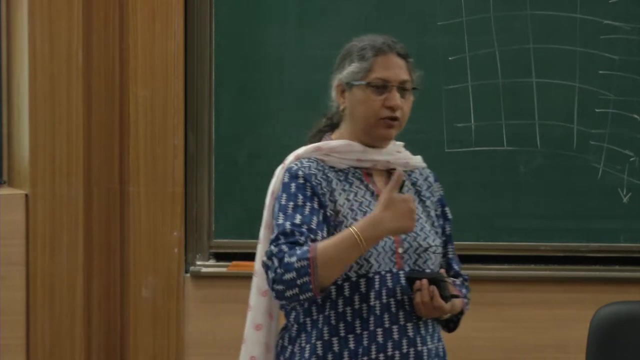 Then you can have hot spots, which is essentially the regions where you have a slightly larger dark current as compared to its adjacent pixels, And when the pixels saturate, that is, it reaches its full well capacity. When you read off, it again leaves a trail behind. 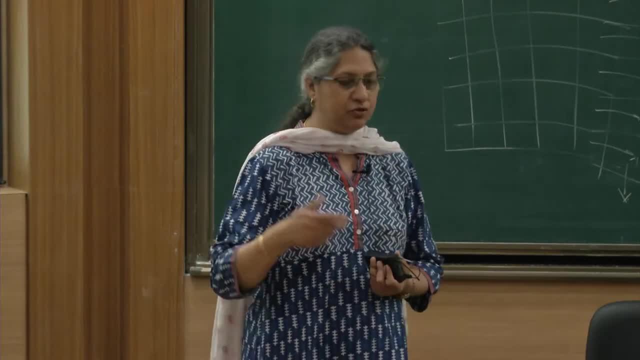 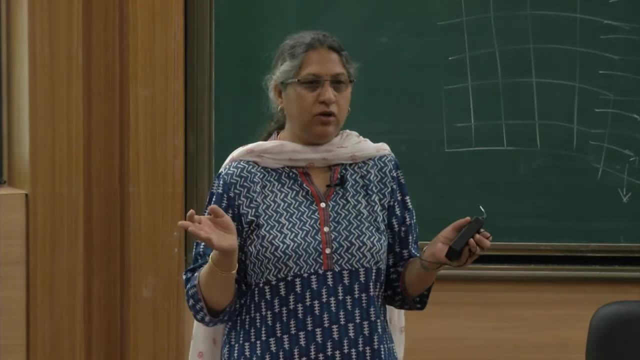 So this is called as blooming. And then if you, of course, you have something called the cosmic rays which Varun talked about yesterday, And this is which happens in all CCD. This is not a manufacturing or a fabrication defect per se in the CCD chip. 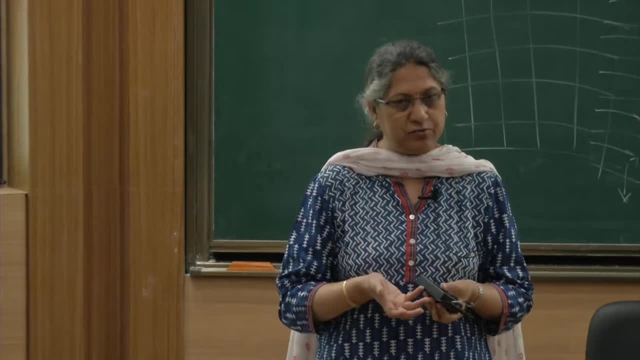 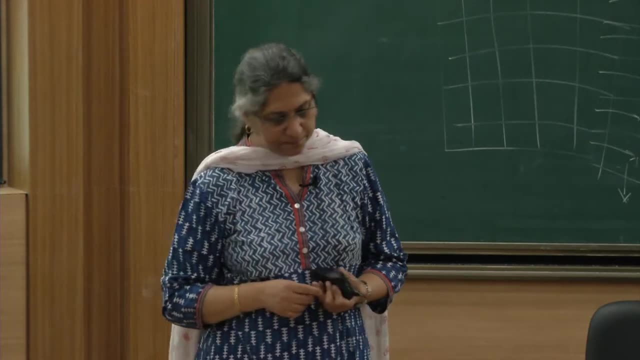 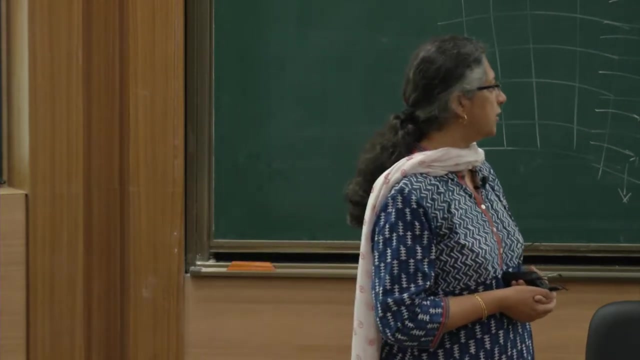 It is just that these, you know chips are sensitive to these cosmic rays which are there all over, And you can have a lot of these events which are affecting your images And then, as is the case in any detector, you have these noises. The read noise is essentially the noise due to the readout electronics. 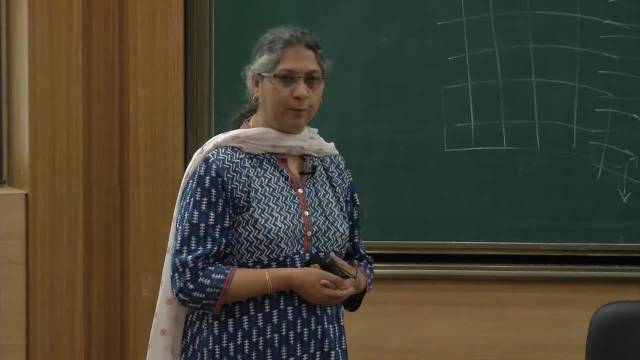 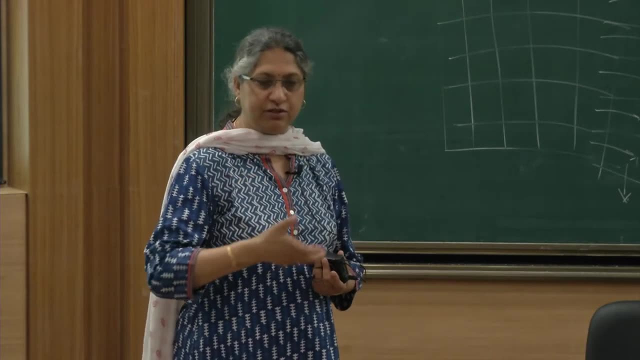 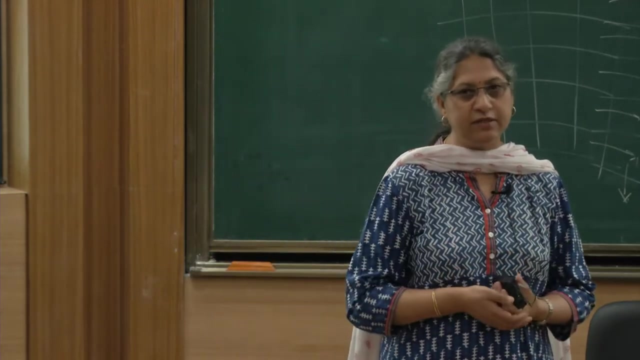 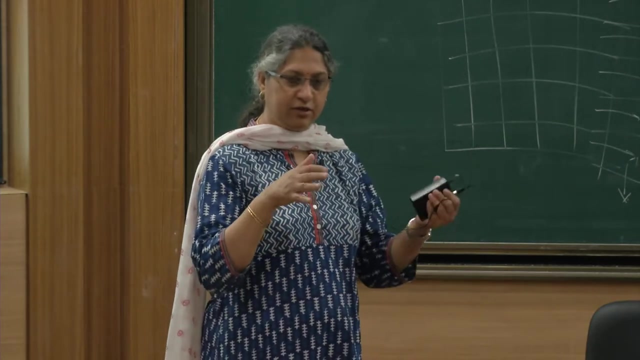 And then you have the thermal noise which is, you know, due to the. there are these electrons which are generated, you know, just because of the temperature, And much of the thermal noise can be reduced to practically negligible Limits by cooling the detectors. And typically all the CCDs are cool to you know, kept in a liquid nitrogen divar and it is cooled, or you have the peltier cooling systems. ok, 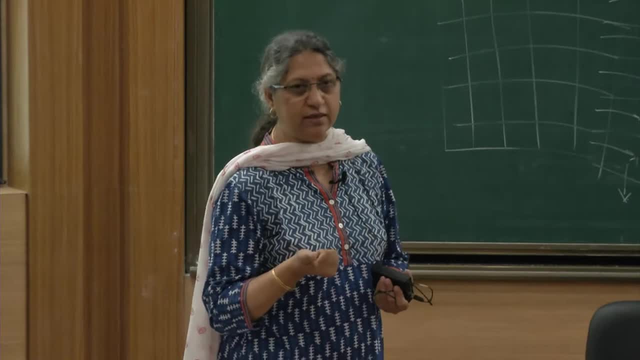 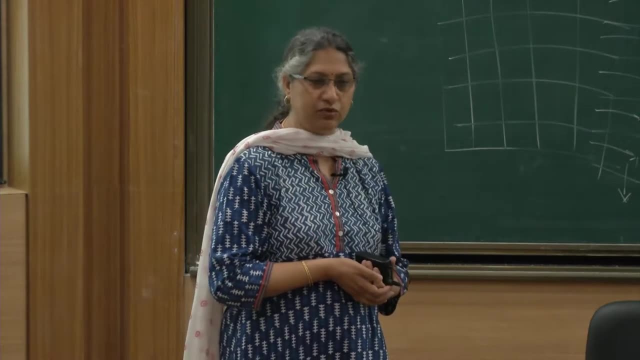 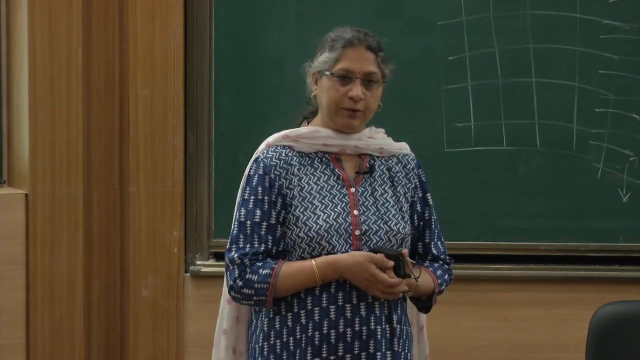 The growth telescope, the CCD camera which is used there is peltier cooled, Whereas on the HCT, and you know many of the other telescopes, the CCDs that are used are liquid nitrogen cooled. ok, And then you can also, And then you can also have, you know, a slight difference in the sensitivity from one pixel to another pixel. 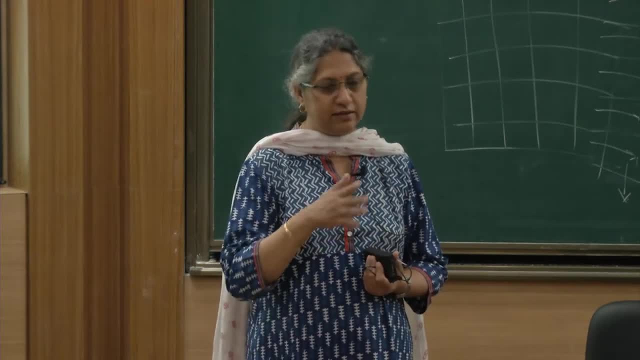 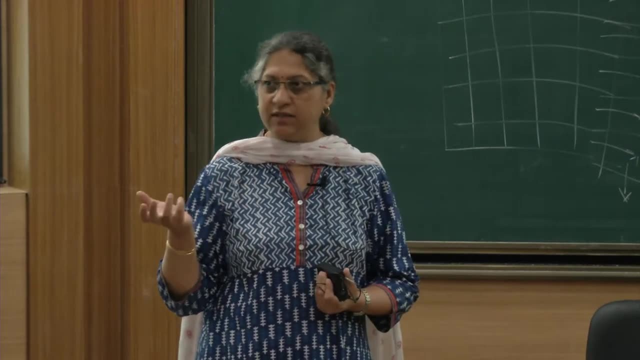 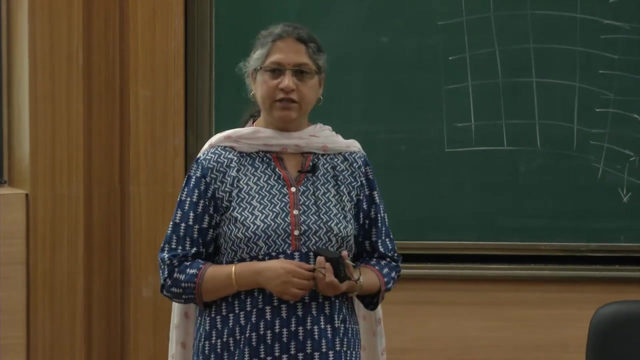 So this also causes some kind of noise level, And you need to have an understanding of what these variations are to be able to obtain the flux that you actually get from the astronomical source. So some of these we need to take care of when we are doing our image data analysis. 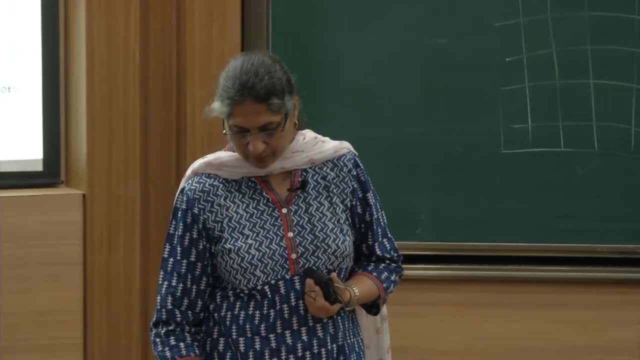 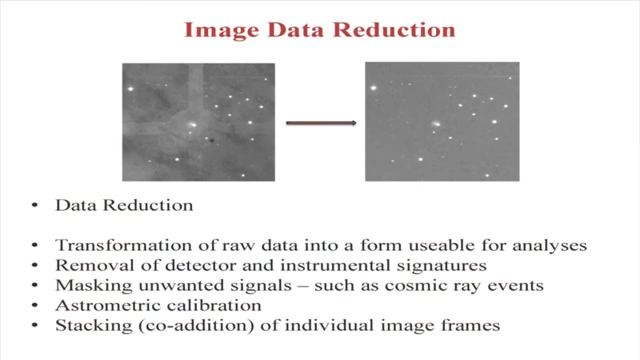 And I will go through the steps of what we need to do to take care of these defects. ok, So what is image data reduction? ok, It is nothing but transformation of the raw images that you get from the telescope, They from your detector- into something that is meaningful enough for you to do science out of it. ok, 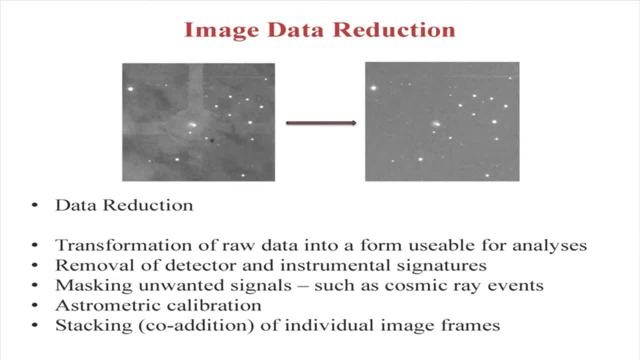 So what do you need to do? You need to remove the detector and the instrument signature from your images, And then you need to remove, And then you need to remove all unwanted signals, like the cosmic ray events, which has got nothing to do with the object of your interest. 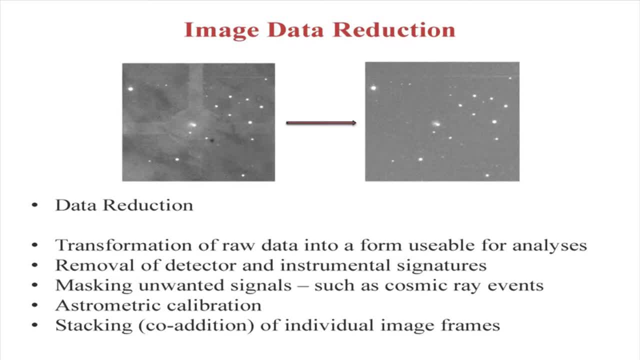 And then you do what is called as the astrometric calibration, What we were trying to do yesterday when we had this, you know, doubt of. did we observe the M77 supernova, right? I mean, we could not really identify the field. So what did Shubham do? 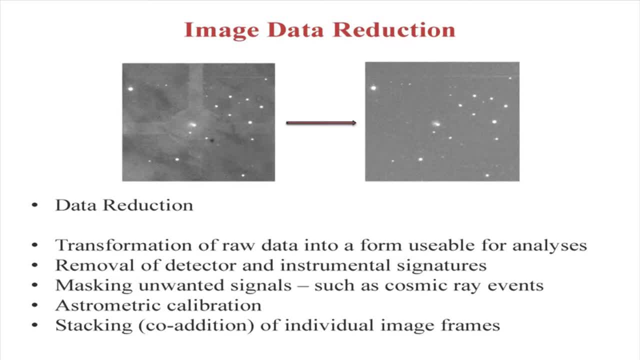 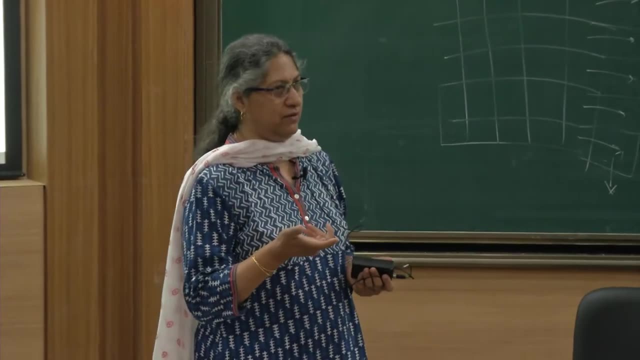 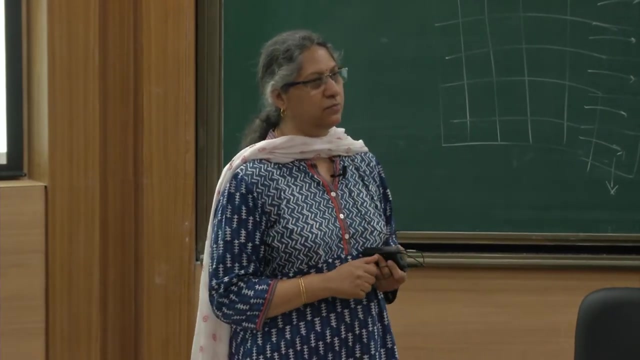 Can anyone tell me what was done If you had paid attention to all the discussions, All the discussion that was happening? Sorry That the contrast in the brightness was changed so that we could identify the supernova right. But then there was something else which Shubham did and based on which we said: yes, this is a region we observed. 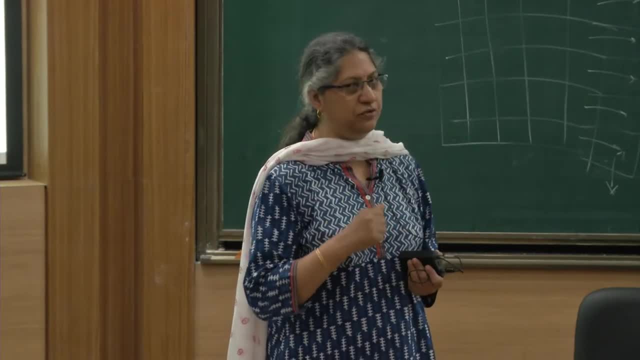 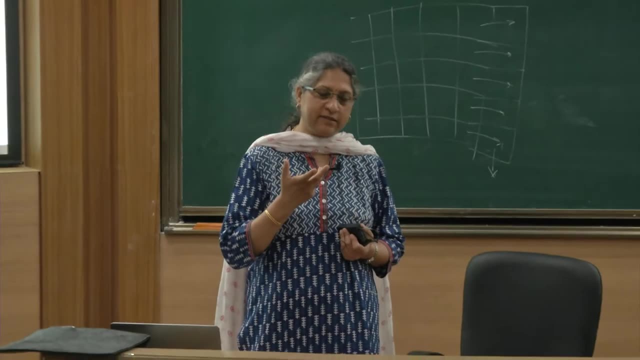 This is the M77 supernova region, which is what we wanted. How did we come to arrive at that? Yeah, we compared with the bright star, but we still we were doubtful right because we had a little bit of distortion in the image, So we had doubts. 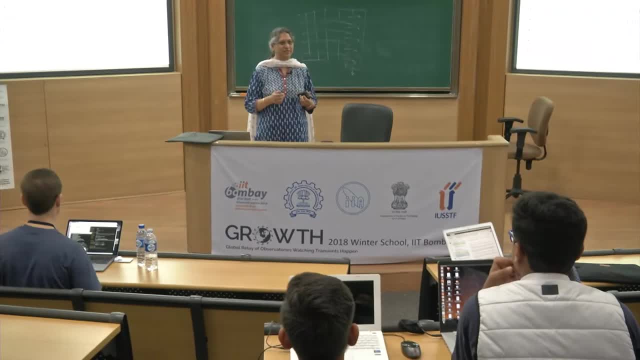 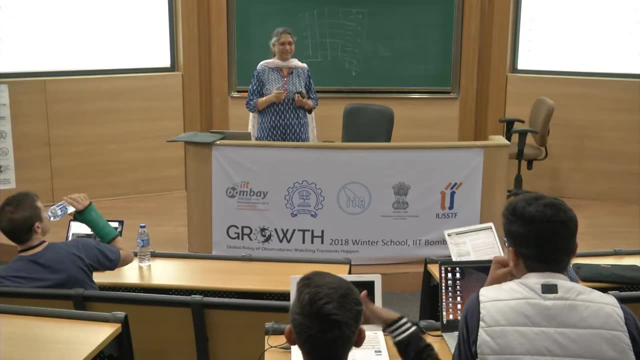 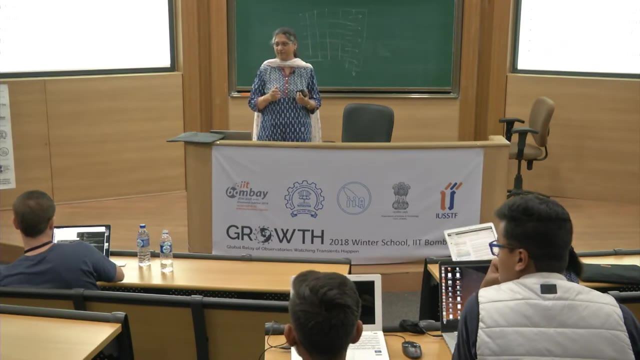 Yes. so what is meant by astrometry? What did we do? How did we confirm Yes, and So, essentially, we tried to see what waswhat were the coordinates of the field that we observed? 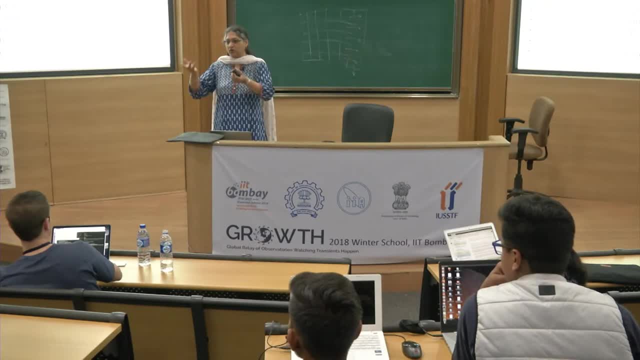 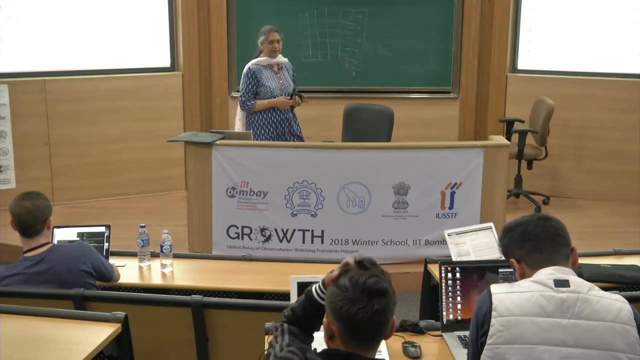 Yeah, and what are the coordinates of the supernova You match it with? The supernova was, of course, not in the centre, but nonetheless we knew that it was within the field of view of the detector Right. So that is what astrometric calibration is all about. 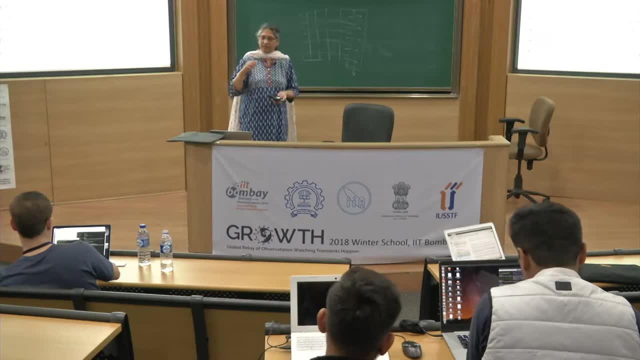 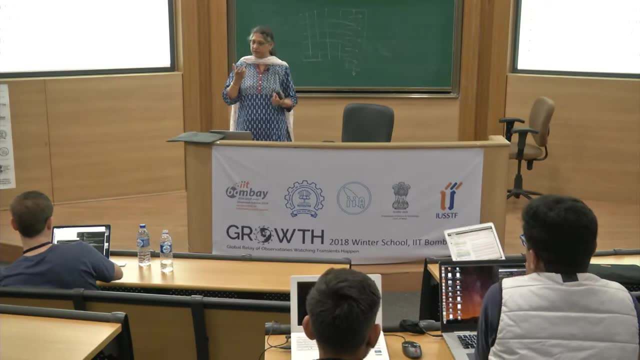 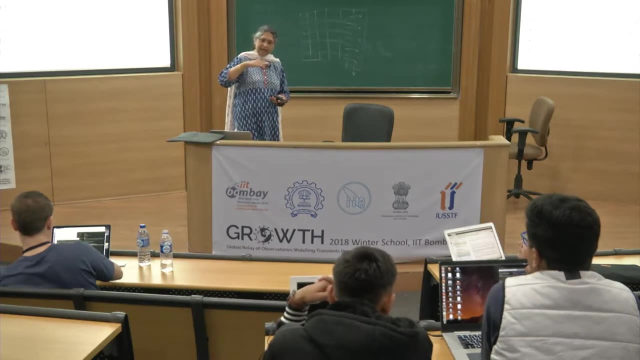 And then when you take multiple images of the same field field, which we normally do for various reasons, one is the one of the main reasons is to improve the signal, to noise, That is, you want to enhance the signal in your data. So when you do that, you stack these individual images or you combine them together. okay, 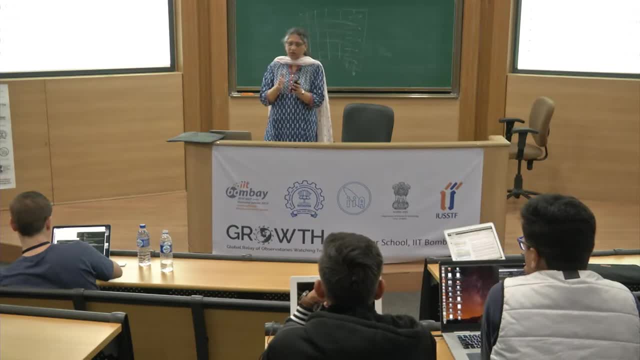 So when you combine them together, you have to ensure that all of them are perfectly aligned, So that it they don't introduce further distortion, So that you do astrometric calibration, and then you can stack them, Or you can stack them even without doing an astrometric calibration, by matching the pixels. 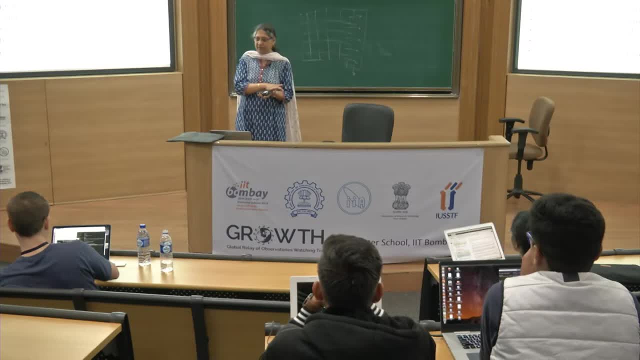 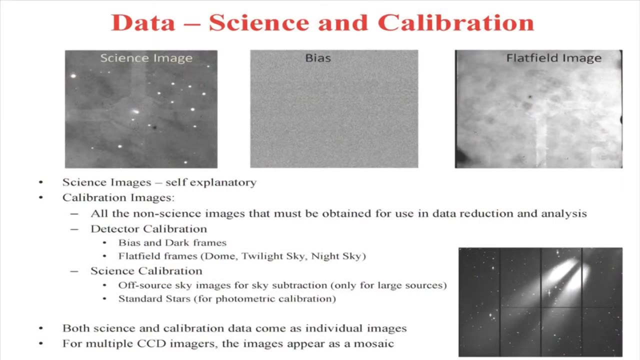 Very well, and then you can do the astrometric calibration. Okay, so you can do it either way, and or you can do calibration and stacking together. packages are available to do that. So let's go on with each of these individual steps now. So, as I've been saying, 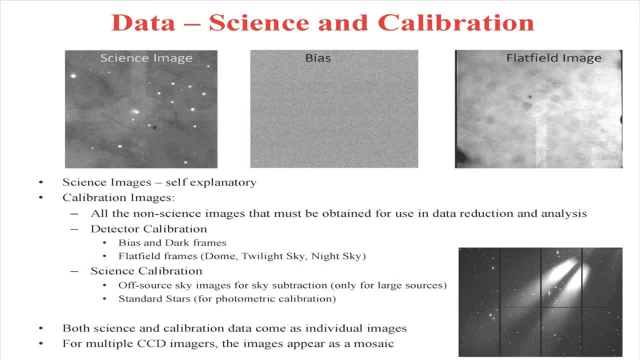 The data itself, I mean, contains your astronomical observations. what these are, I don't need to go into that, But what is important is that you need to take certain calibration images. Okay, So these are the, the non science Images that you need to take. okay to. 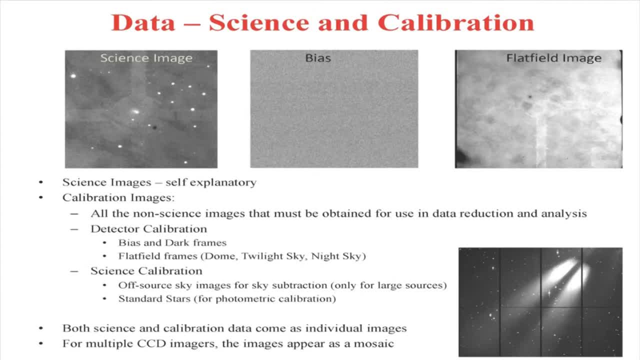 Help you in removing the detector and the instrumental characteristics from your data. So what are these detector calibration frames- These are what we call is the bias and the dark frames, and then the flat field frames and, for the science, calibration Itself. in certain cases you might need to take 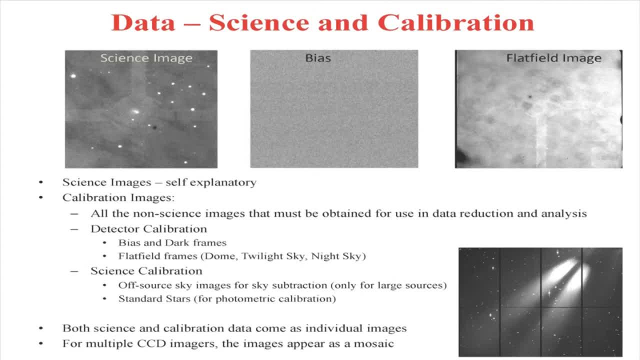 Images which are slightly off the actual source area, Where you have a slightly blanker, you know, fields. if this is in case, your Objects are extended objects and they more or less fill up the whole detector. So you do that because you also need to subtract the photons which are coming from the night sky. 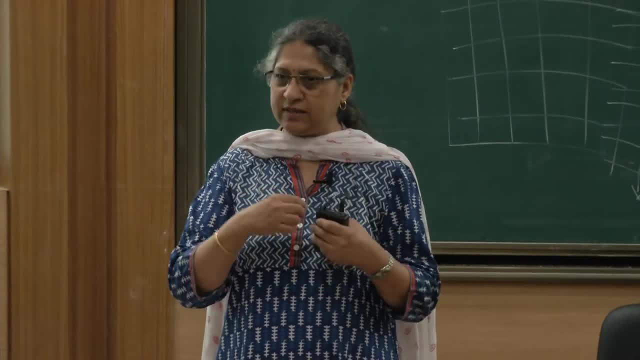 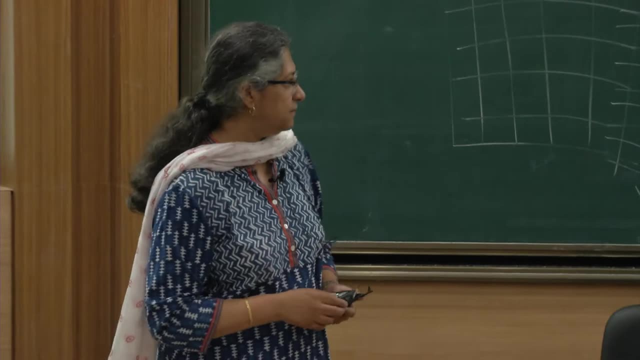 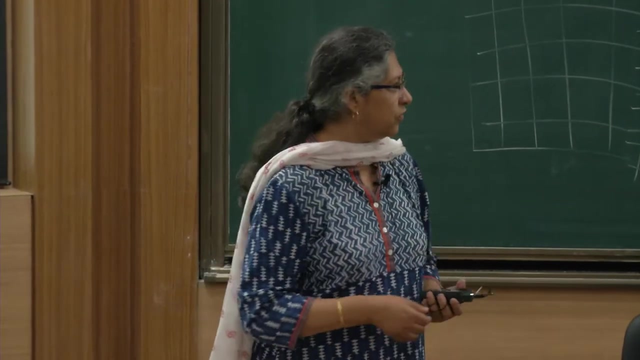 Okay, So the for that you do, for the, what we call as a sky subtraction, you would might want to take another image which is offset from the object of interest, and Then, of course, you have to have observed standard stars for Photometric calibration. What are these standard stuff? Yes, 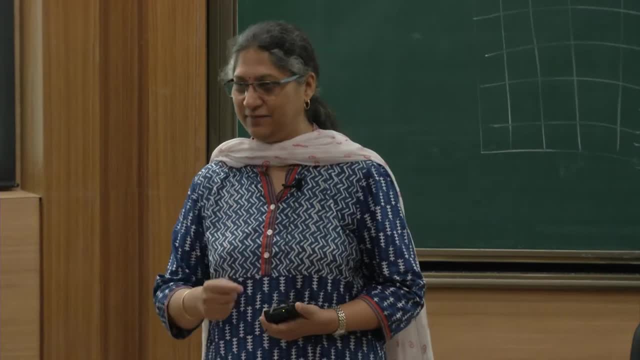 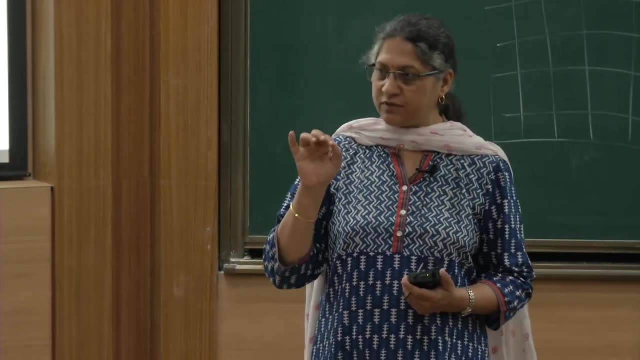 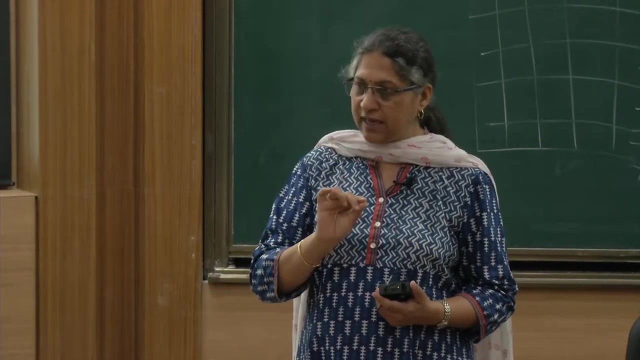 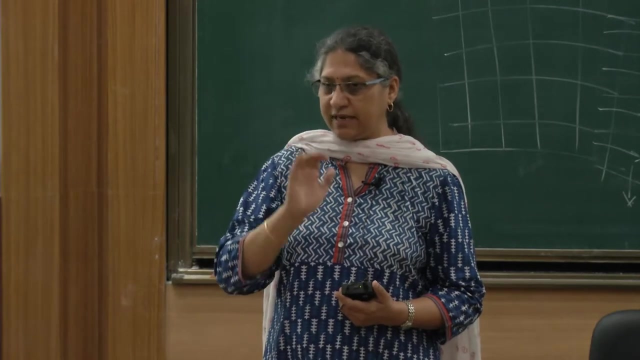 I'll come to that. So What are these photometric standard stars? these are regions of the sky where The stars have been very well studied and they're found to be Non variable. their fluxes are well understood and so these can be treated as Standards. the magnitudes are treated as standard. So, essentially, you will hear more about it in the next. 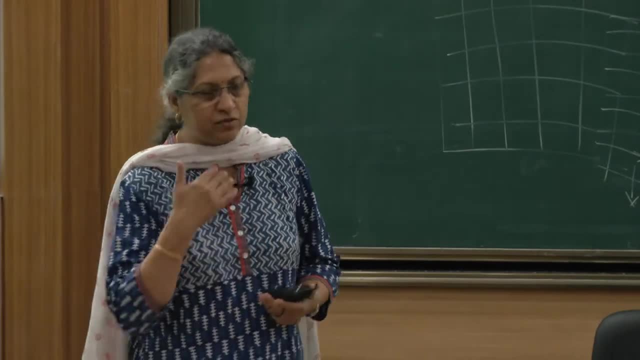 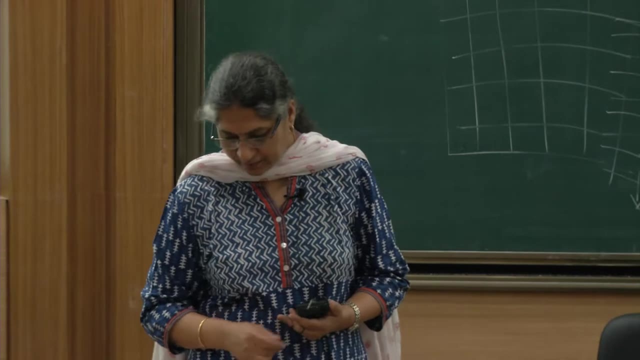 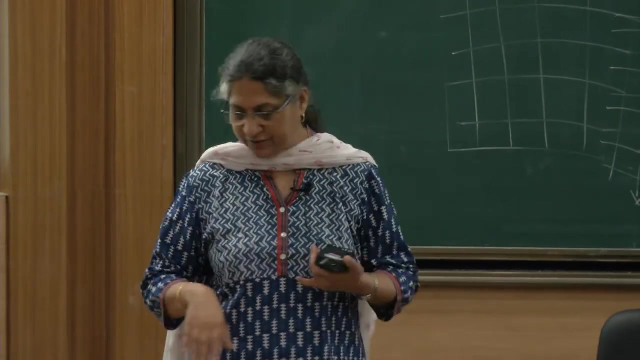 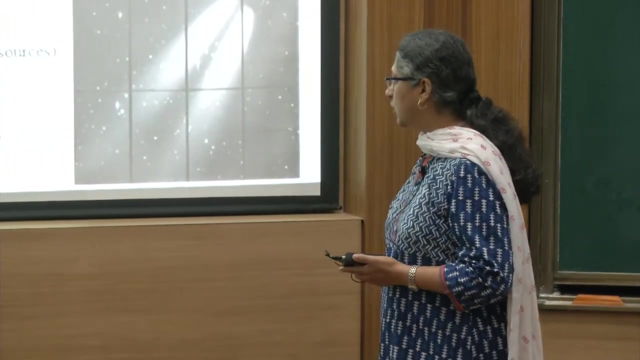 talk on how to do this photometric calibration, So you need to have observed these objects also. ok, So in the case you have CCD images with multiple CCDs, these appear like a mosaic, and what I have shown here is just an example of how such a mosaic CCD data would look. What you see here. 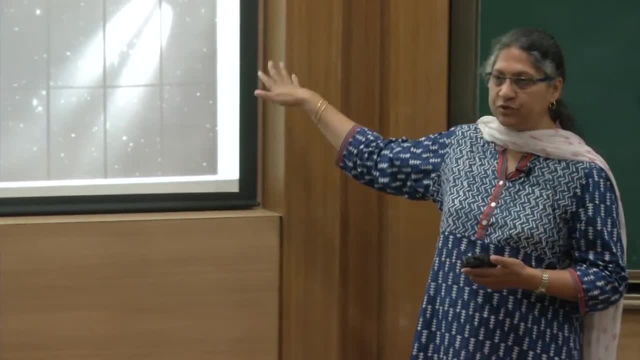 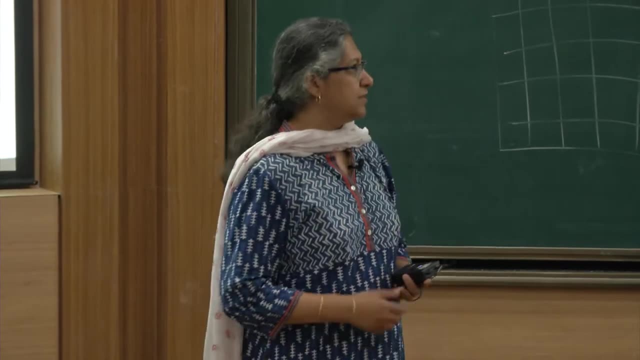 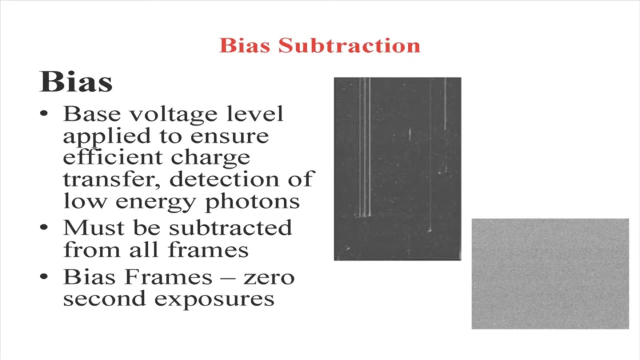 in between. these are the gaps between the CCDs which have been mosaic together. ok, What is bias? there is always a base voltage level that is applied to the CCD. one of the reasons for doing this is you try to keep the potential well to a certain level, so that 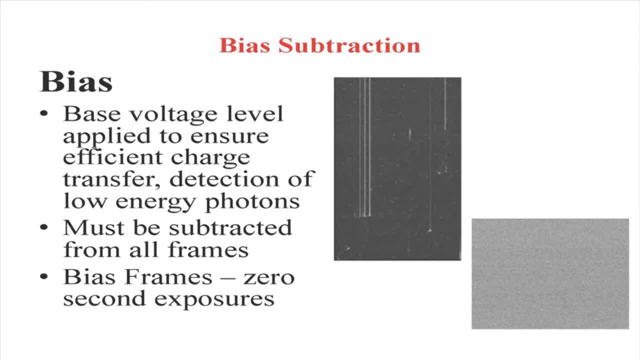 even a faint photon which is striking on to the detector can see the potential value, a certain level of potential. So if you want to do this for a certain level, in this case you need to keep the potential very low. So you try to keep the potential very low, because the ones which are 하니까 up to this level are the ones 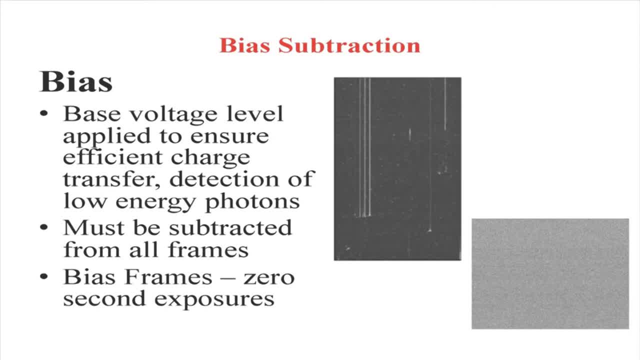 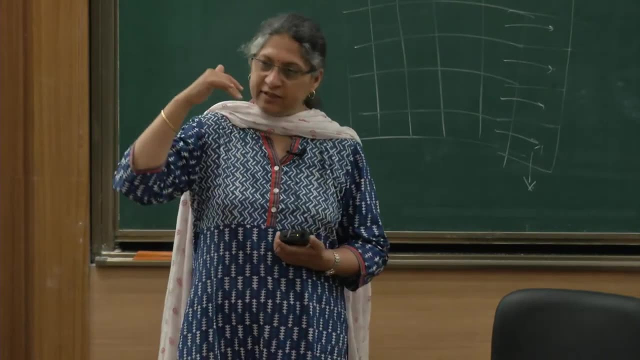 generate sufficient number of electrons for us to be able to read out. ok, But one needs to be very careful and actually the this is what the bias level is determined by the gain. ok, So you need to be very careful also that you do not have an extremely high gain if 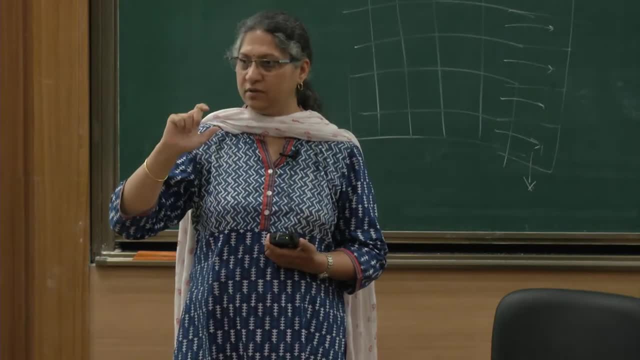 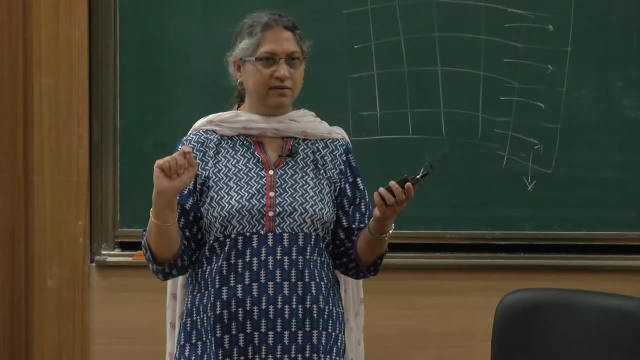 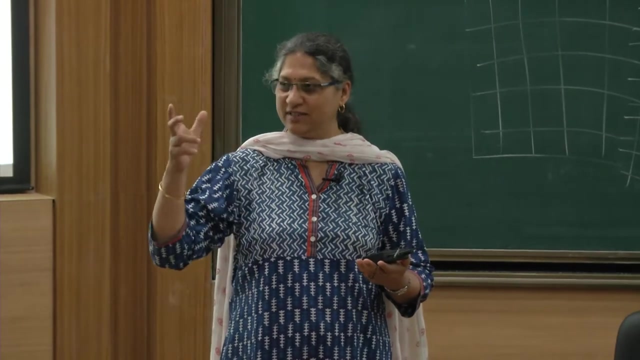 you do that, you will be reducing the dynamic range of the detector. What is meant by dynamic range? Anyone make a guess, Not you, I think you have experience. I want somebody else to tell me What is the term itself. what does it indicate to you? Yes, in a certain 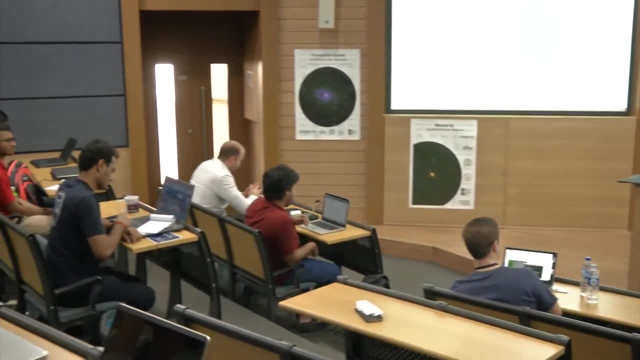 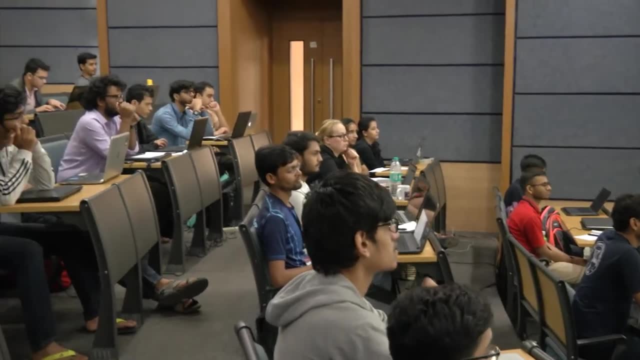 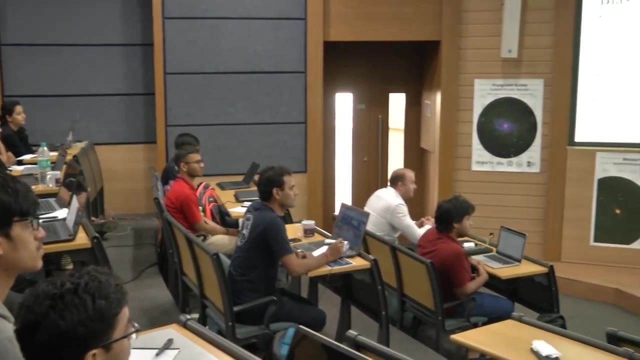 sense. yeah, yeah, yeah. So so what is important here is that we need a detector which can not only detect the fainter photons, but also the brighter ones. right, It does not always happen that, but we need to have a good range of fluxes that can be. 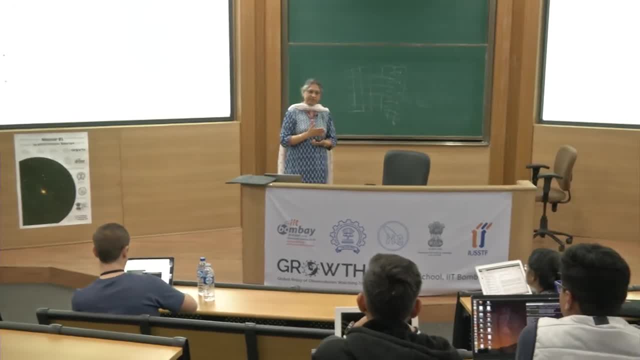 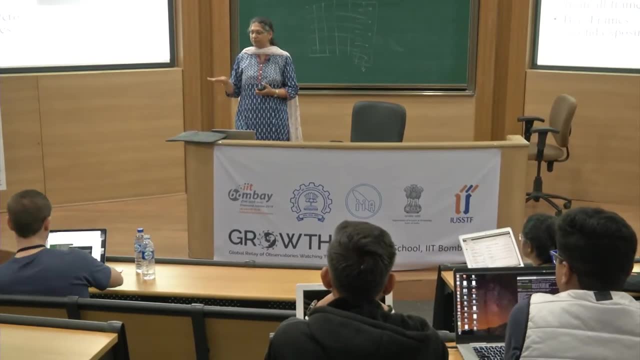 detected. ok, We do not want to have a detector which is tuned only to the faint objects, as a result of which we want to saturate all the bright sources in the field. ok, So you are not going to be able to get any information about the bright sources in the field. we? 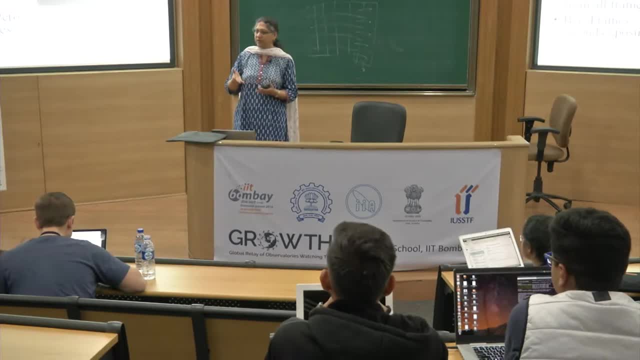 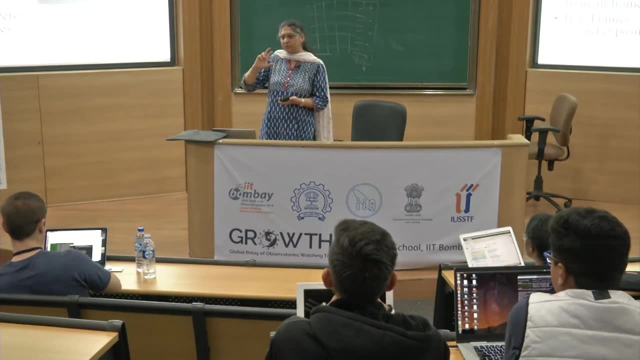 do not want to have such a situation. we do not want to have a detector which cannot observe bright sources, So you have to have some optimal range. ok, So this is the dynamic range. with that we taught The CCDs have a fairly good dynamic range and we keep the bias level at such a 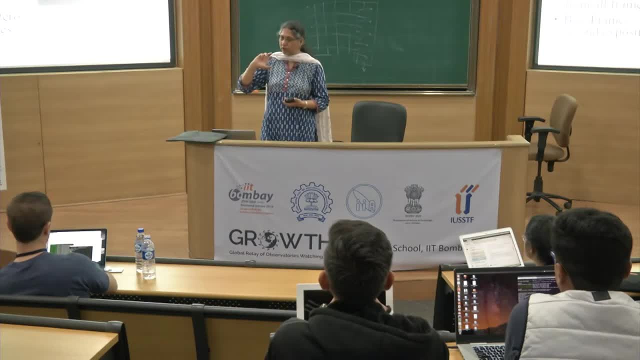 you know, at a level where we have a good enough dynamic range. ok, So it is determined based on you know what you want to do with your detector. So sometimes detector, the instrument, also have the option of changing the gain. So if you are observing a faint source, you 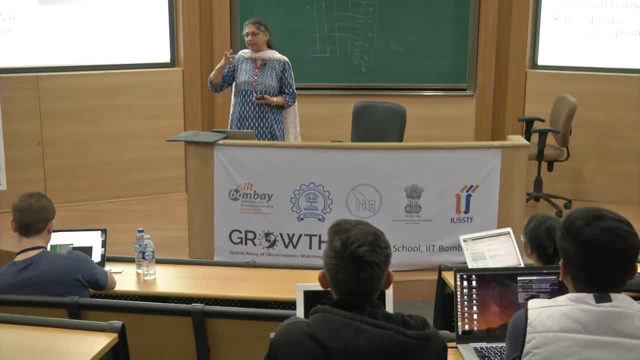 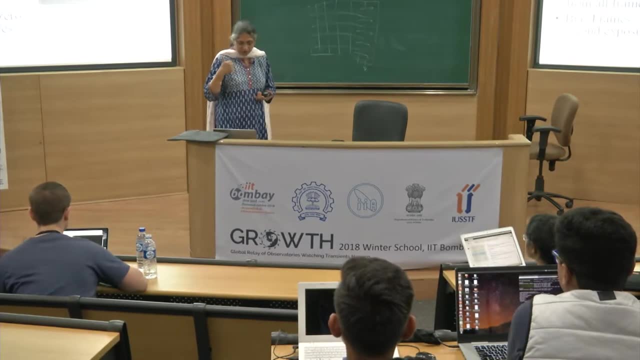 can, and you are not interested in the bright objects. you can have a slightly higher gain so that you can, you know, detect your source with the shorter exposure time. ok, So what are these bias frames? These are nothing but 0 second exposures. So what is happening? 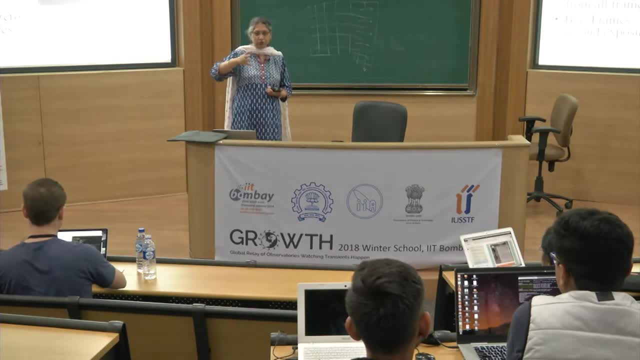 is, you are just reading out, ok. So when you do this, the base voltage that is existing all the time in the potential, well, Which is giving rise to certain electrons, that is read out. ok. So this is giving you the this level, which is of voltages, which is there in every pixel which you have to. 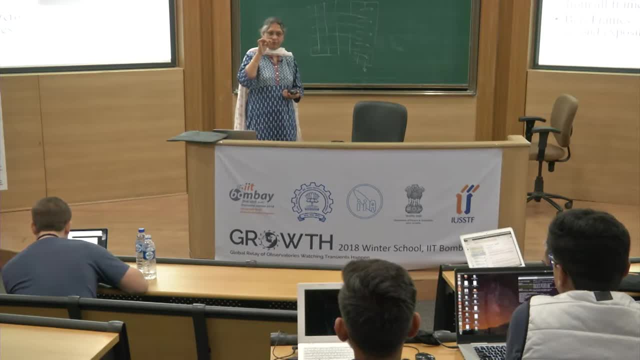 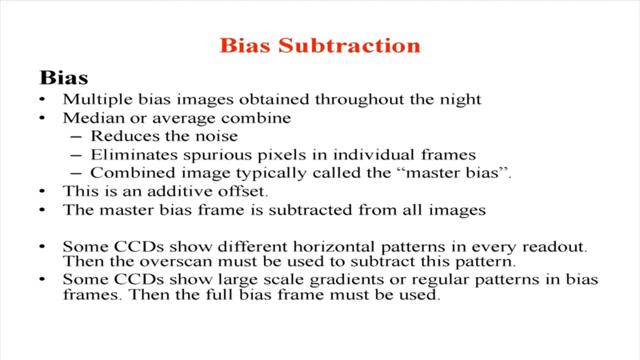 subtract out from the image. ok, So you need to ensure that these electrons are not treated as the electrons arising from your, from the photons of the astronomical object. ok, So they need to be subtracted out. So what you do is you obtain multiple images. 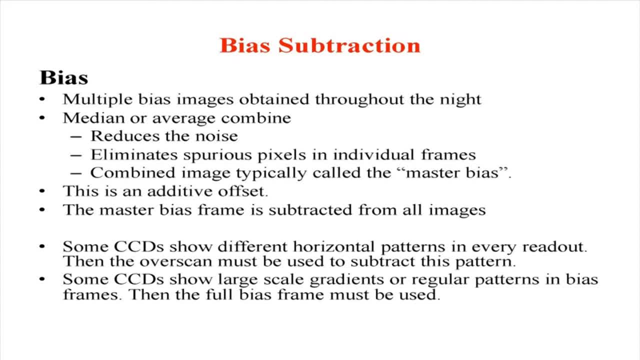 either in the beginning of the night and the end of the night or you obtain throughout the night. The advantage of obtaining bias frames throughout the night is that if there is some problem in electronics which is causing some kind of a drift in your gain which can 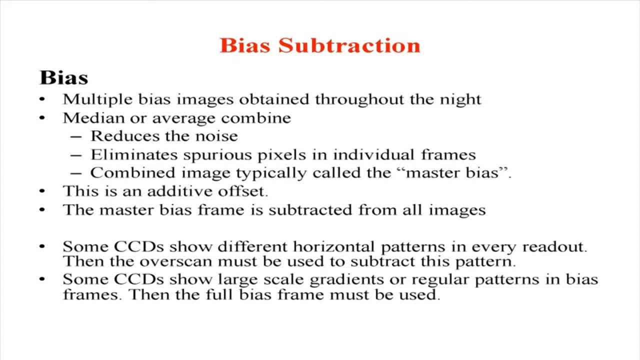 happen, then you find that your bias level is not the same throughout the night. ok, So you might want to doing. keep doing this. this is also giving you a a health check on your system, and it is also depends upon how accurately you want to get your photometry done, in which. 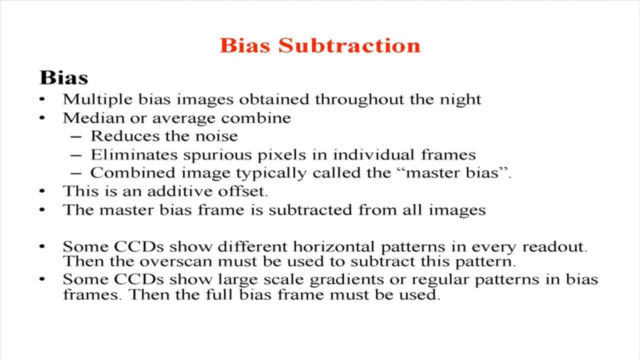 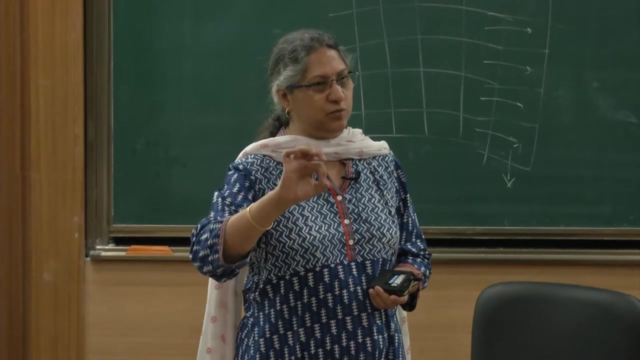 case, it is always better to use the bias values obtained as close as possible to your astronomical observations. ok, We just read it all: Dark, I will come to that. Dark, Dark, Dark, Dark. how it is different from dark. It means that you are not really giving any exposure time. ok, 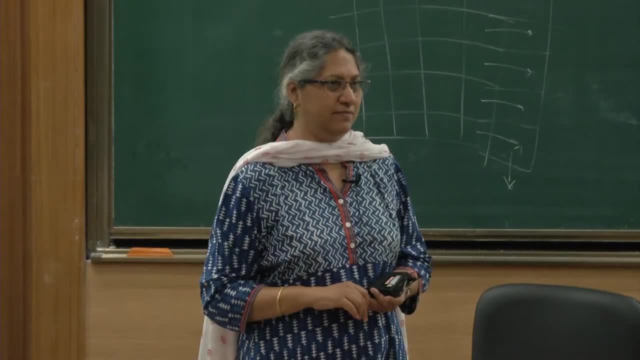 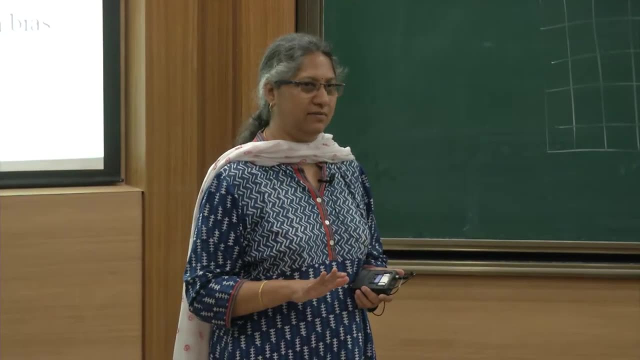 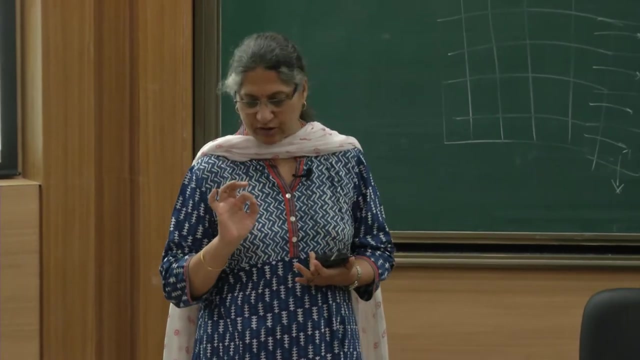 you are not integrating for a period of time. Your detector is on. yes, it is powered on. So you take this multiple bias images and then you combine them. you do a median or an average combining. So why do you do this? To reduce the noise which is essentially the read noise. 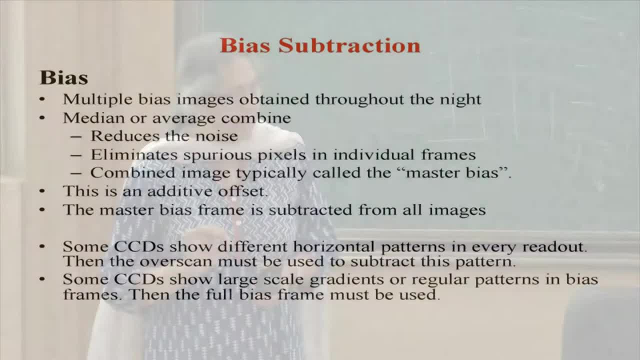 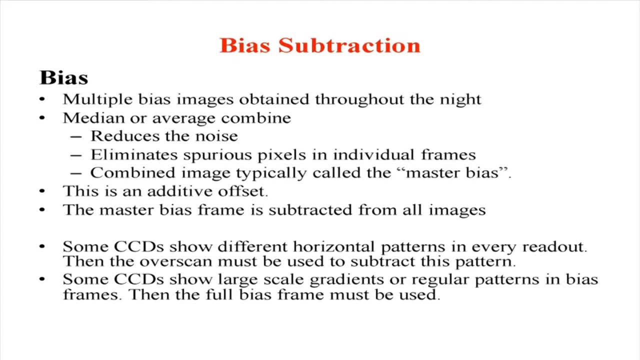 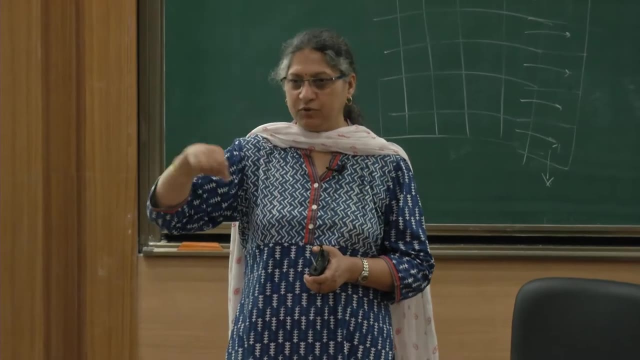 that you have, ok, You do that. and then if there are some spurious, you know events which are struck and some like, for example, there could be some cosmic ray hits. So when you do these median combining they are not going to be in the same position in all your frames, So they get removed. 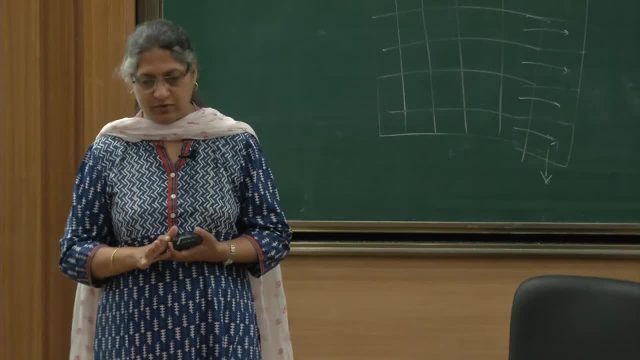 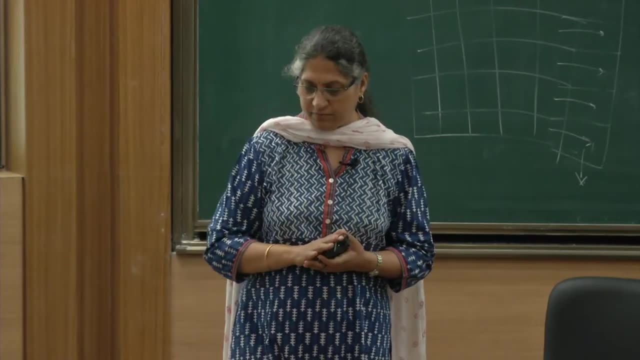 out from the final combined frame. So they get removed out from the final combined frame. So they get removed out from the final combined frame. So they get removed out from the final frame. ok, You create what is called as a master bias, which is median combined bias frame, and then 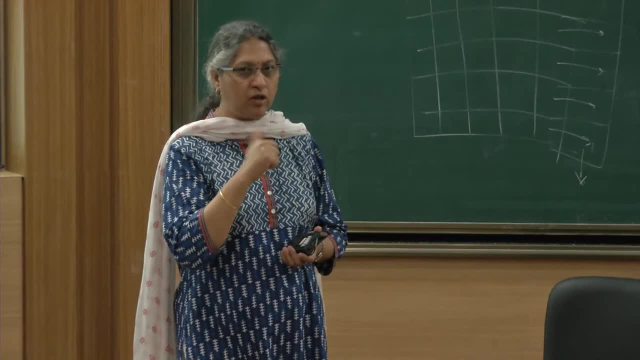 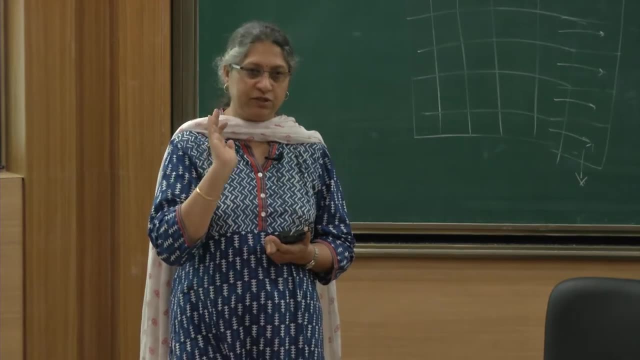 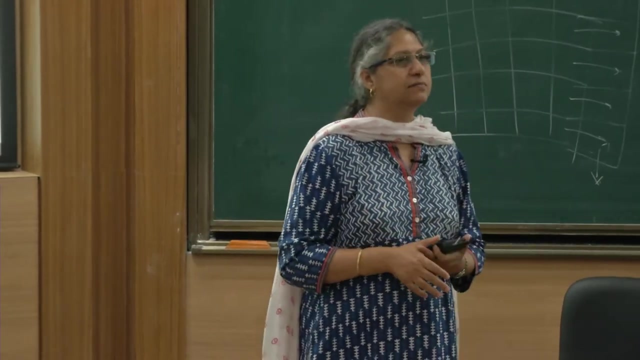 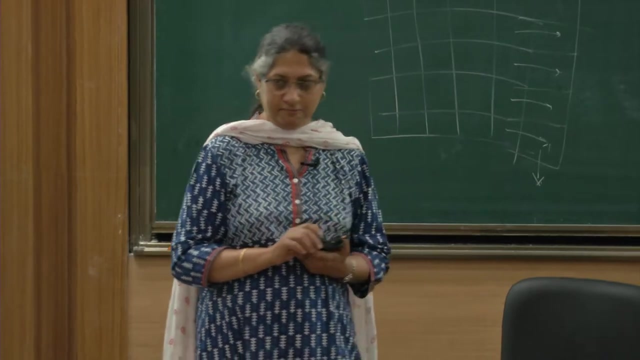 you subtract this bias frame from all the images. ok, So this way you have taken care of this. the 0 level voltage which is applied, the base level voltage that is applied. Sometimes CCDs can. yes, in principle it should not. if your system is stable, it should not. ok, Sometimes, you know they. 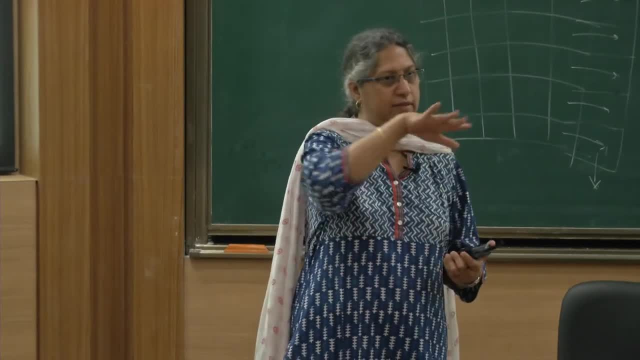 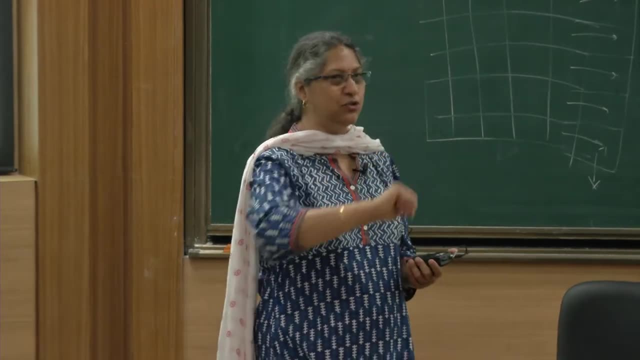 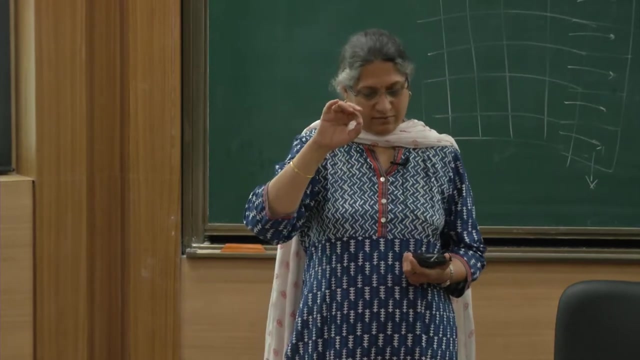 can. you can suddenly find that the CCD is showing some sort of a horizontal pattern, like, for example- which happens quite often in in India, for instance, if you have some issues with your earthing, ok, there can be some pickup, So you will find a pattern, and it can so happen this, this: 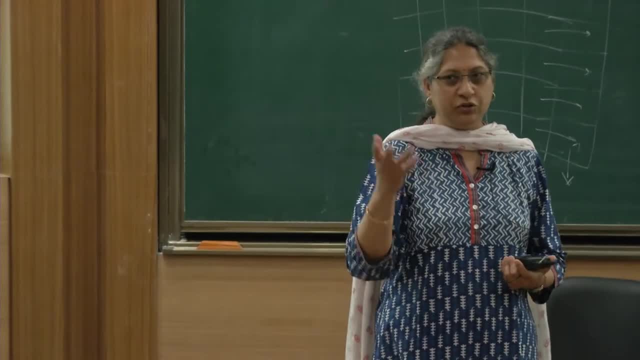 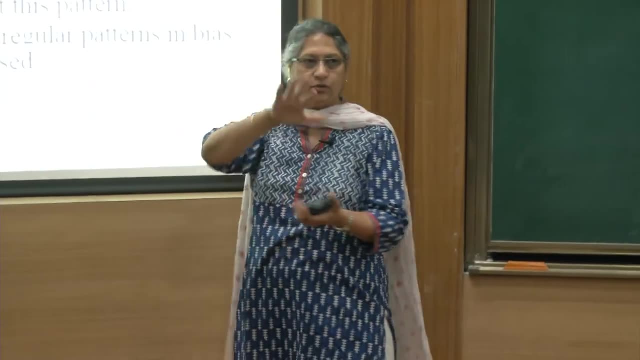 pattern does not even remain stable. ok, So what do you do under such circumstances? What I should told you in in this part: when you are doing the subtraction, you are doing a two dimensional subtraction, that is, pixel to pixel. you are matching and you are doing a two. 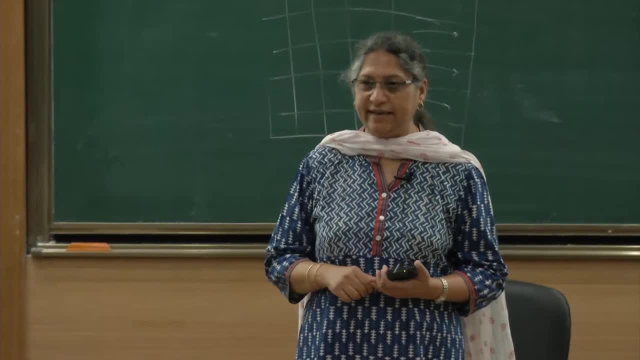 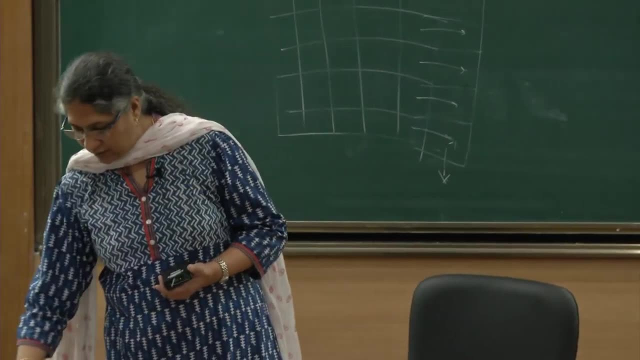 dimensional subtraction. ok. So what do you do when you have something like this? You can just take a median, you can take a constant value and subtract out. ok, So this is what you do in bias subtraction. There are various other things. you can have what is called an. 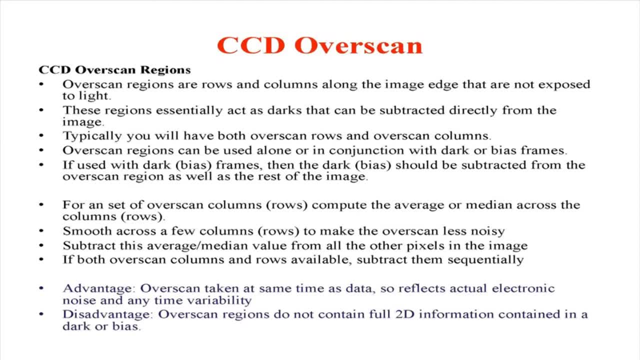 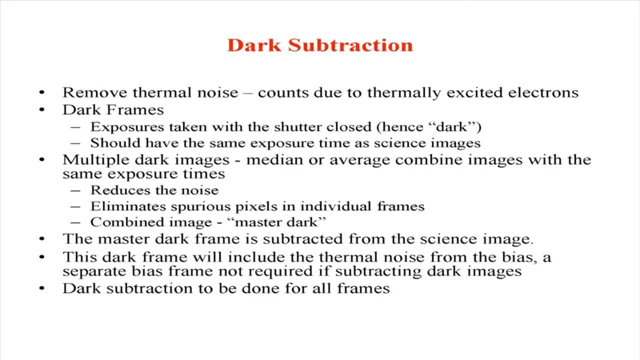 overscan region where you have some extra pixels which are just read out. that will again give you this bias value. you can use that to subtract and some of these things will be shown in the module. Dark is you. you know, do not expose the CCD to any light and then you obtain several images and this: 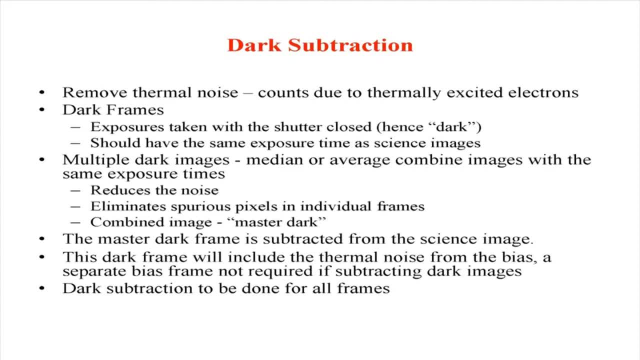 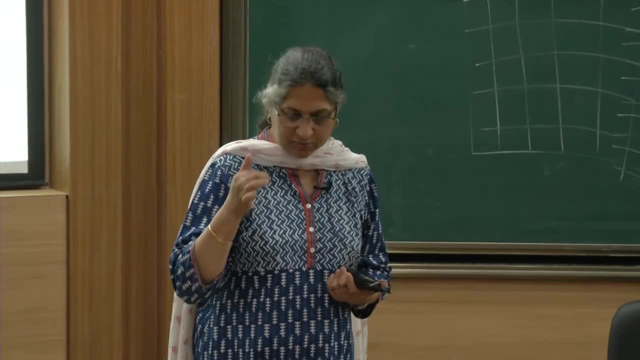 is what you I mean by and large. in very well cooled systems you do not have much thermal noise, but otherwise You have this thermal noise which is a function of the exposure time. ok, So you need to. if you are doing, if your detector has thermal noise, detectable thermal noise, then you need. 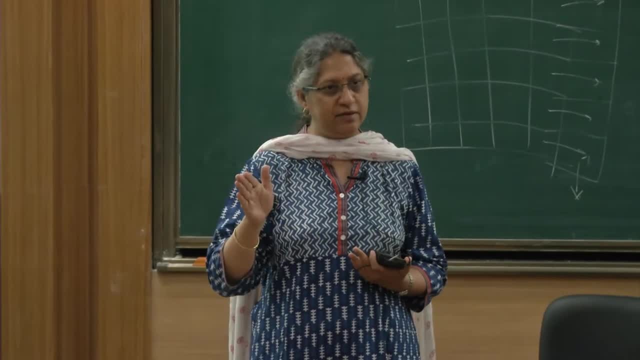 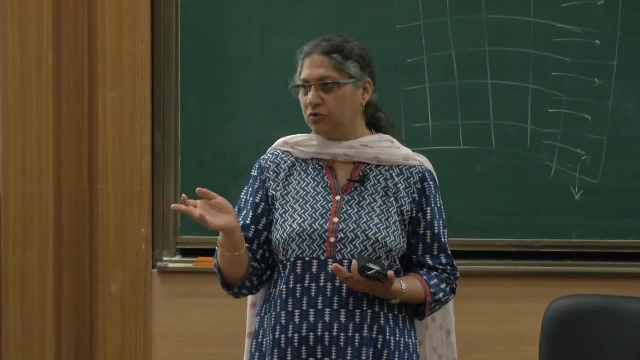 to take dark frames which are the same exposure time as your object frames and that you have to subtract out. Now, when you are subtracting the dark, it has bias, So you do not need to do a an independent bias subtraction. ok, The next thing is flat field correction. Why? 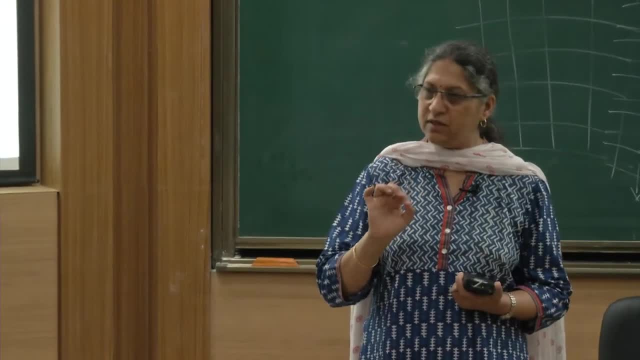 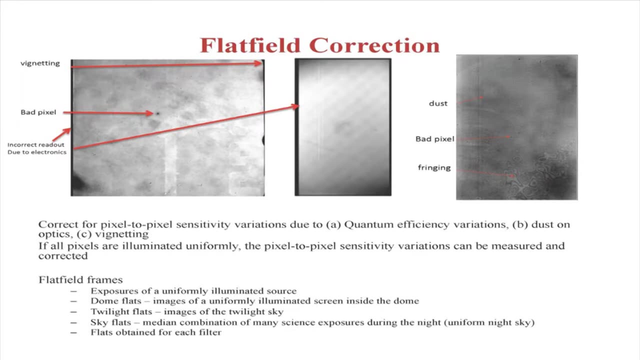 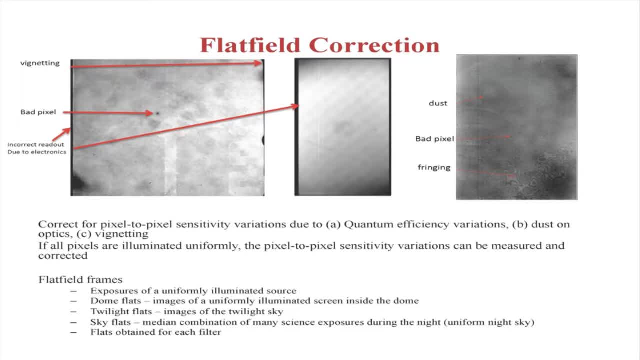 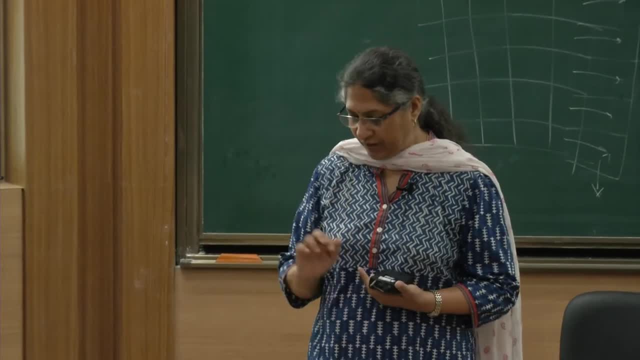 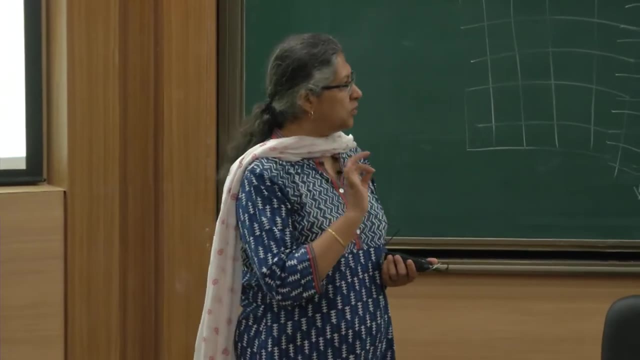 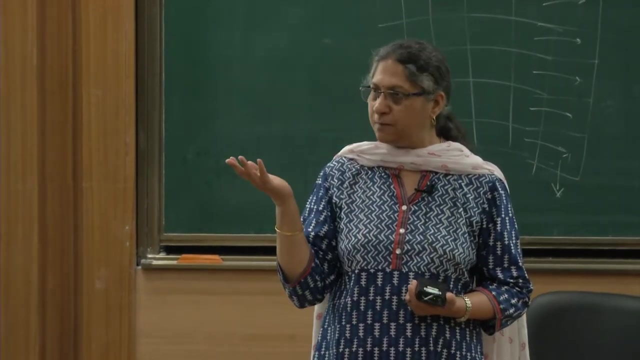 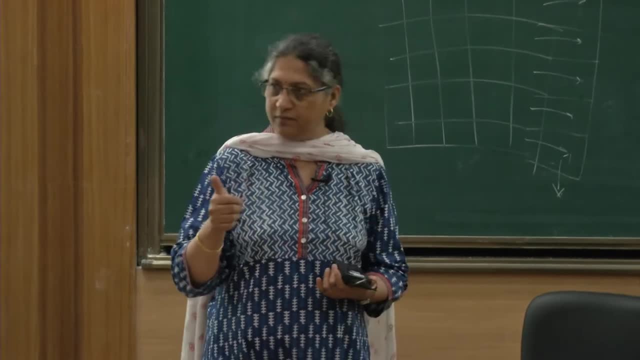 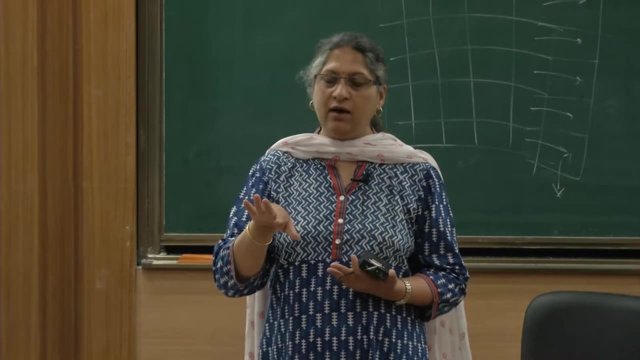 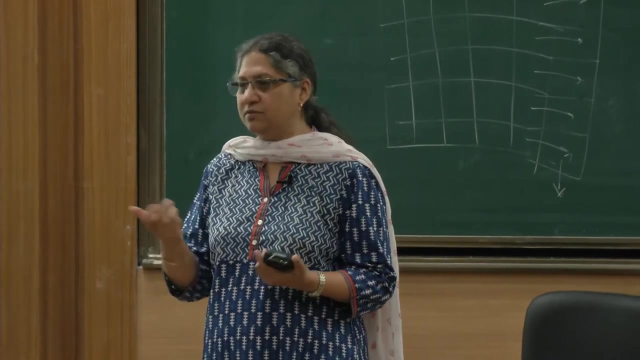 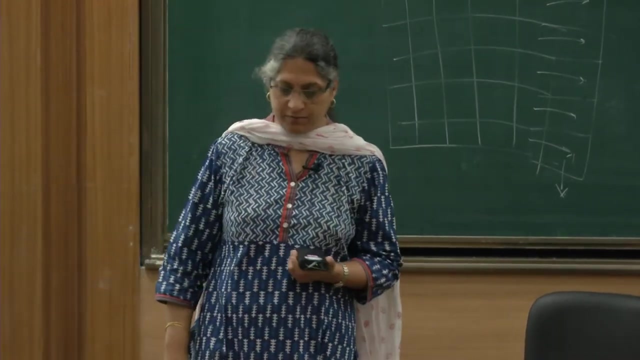 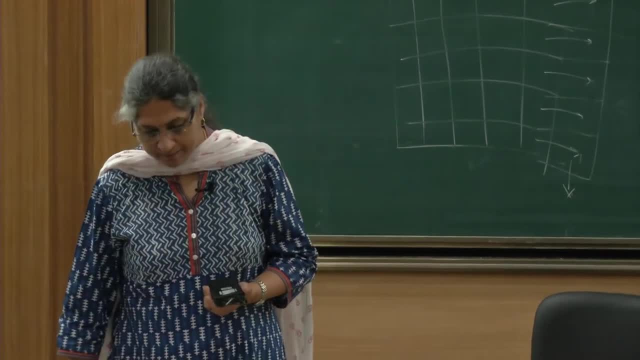 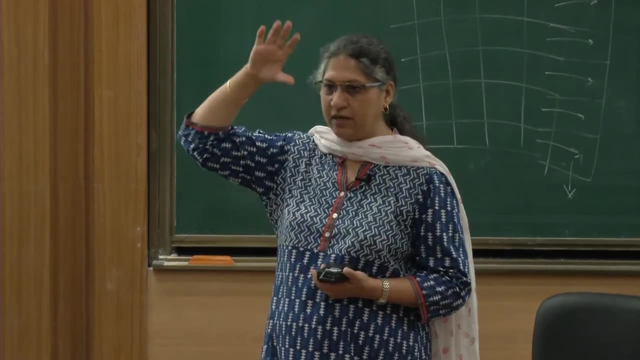 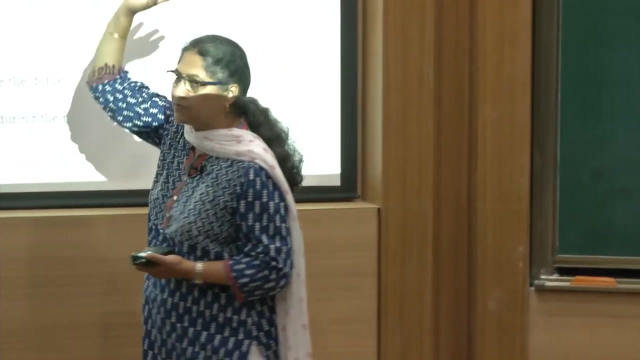 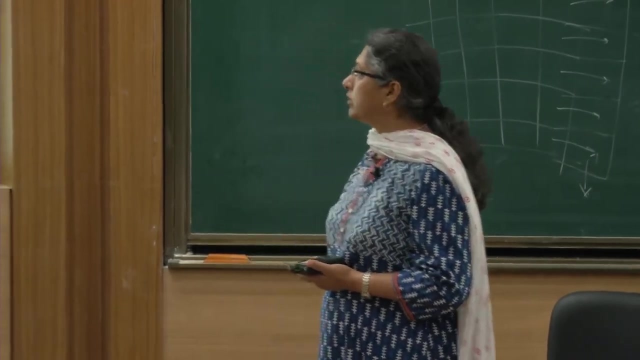 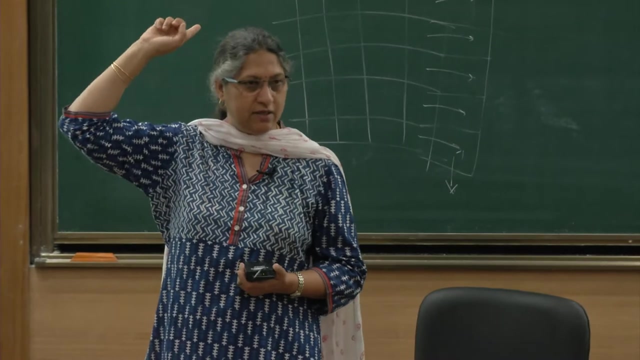 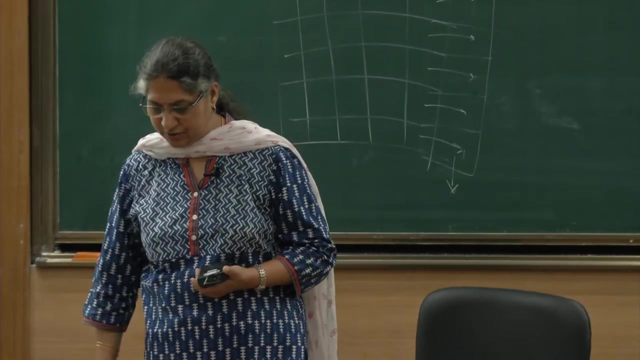 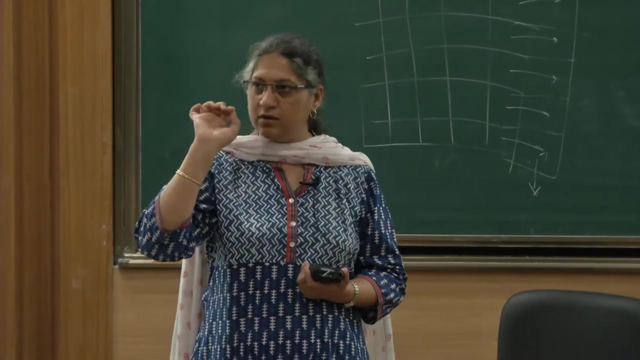 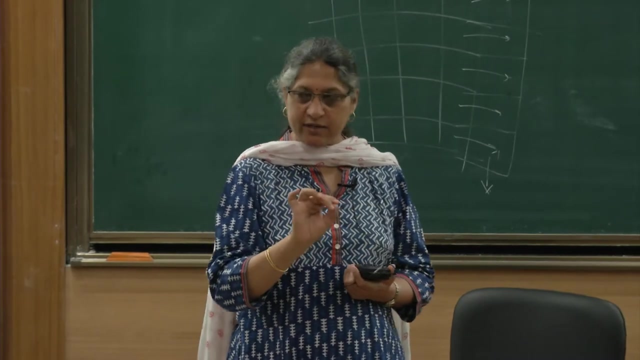 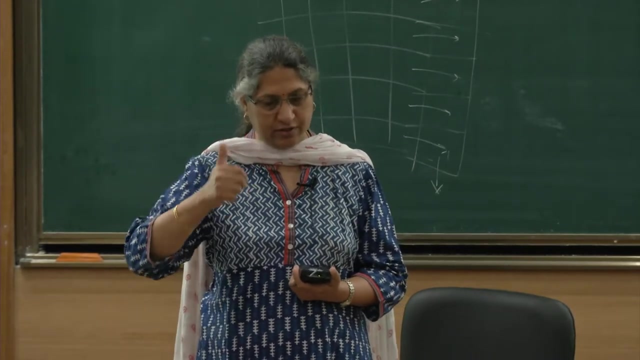 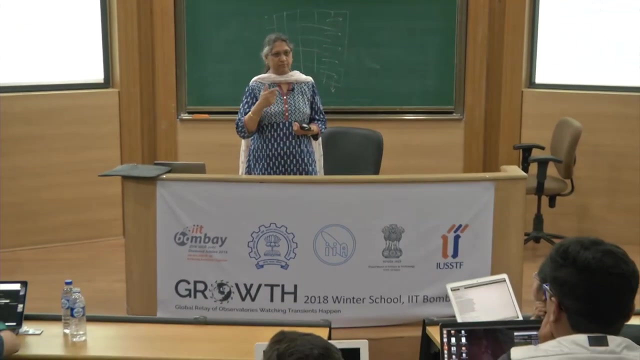 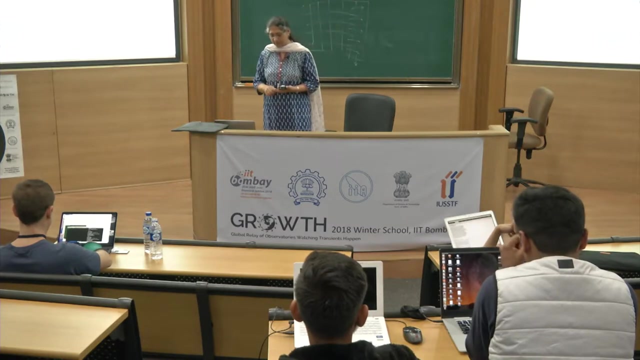 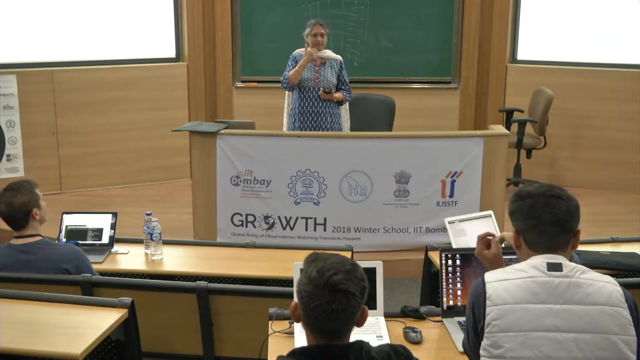 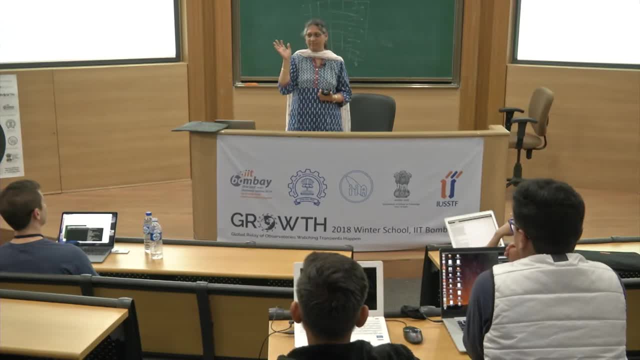 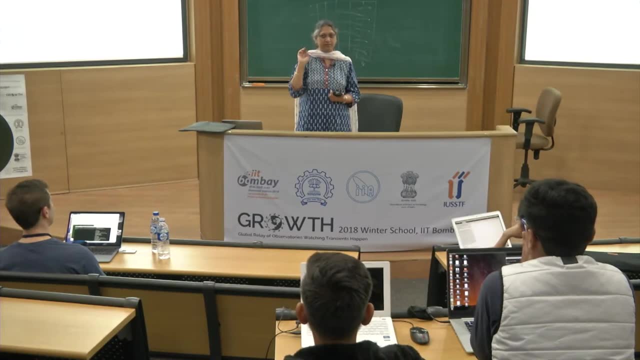 what is important in our data Signal coming from the source, right? So what will happen if you do not normalize First of all, what is meant by normalizing? Yeah, right, So why do we need to do this? 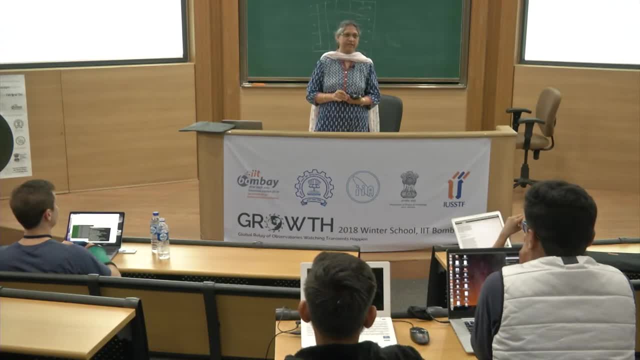 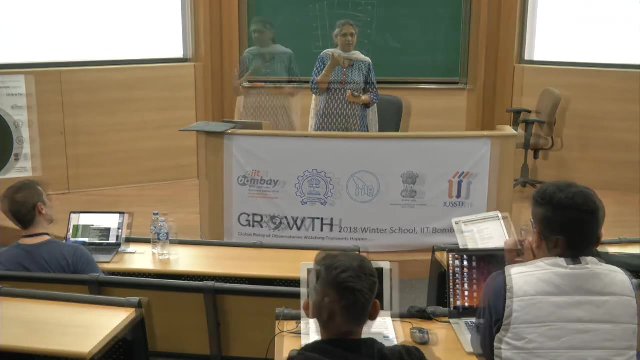 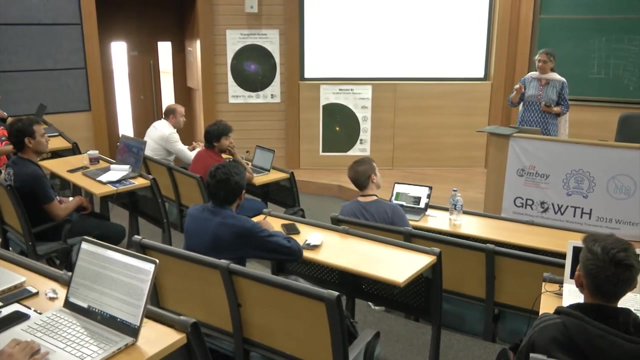 Yeah, so that the, the flux is going to be, the flux that you are getting from the source is not, or the counts that you are getting from the source is not altered by the flat field counts. right, Flat fielding. No, you normalize the flats and then you do. 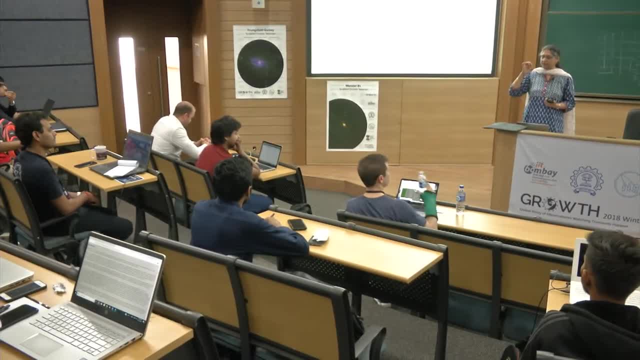 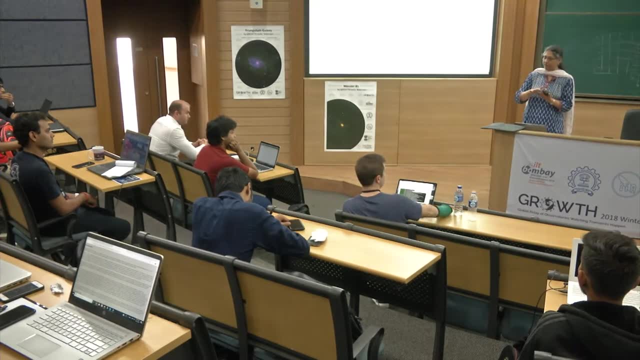 the flat field correction. So what do you do in the flat field correction is that you make the master flat. ok, You can either normalize the individual flats and then median combine them. So you can either normalize the individual flats and then median combine them. 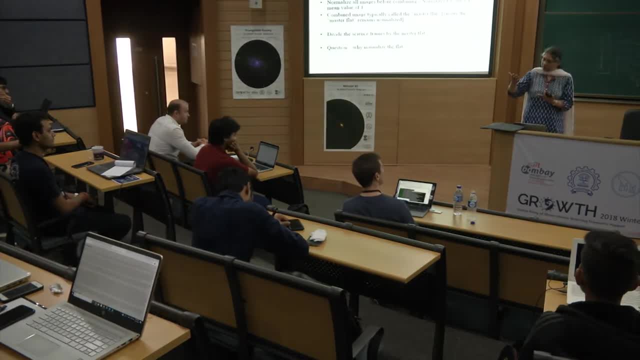 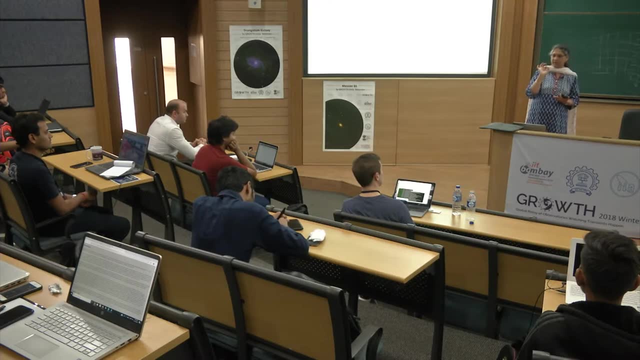 And make the master flat, or you can make a master flat and then normalize that. ok, And then how do you do the flat fielding? is you divide your science data, which is bias, subtracted by the flat field frames? ok, So, 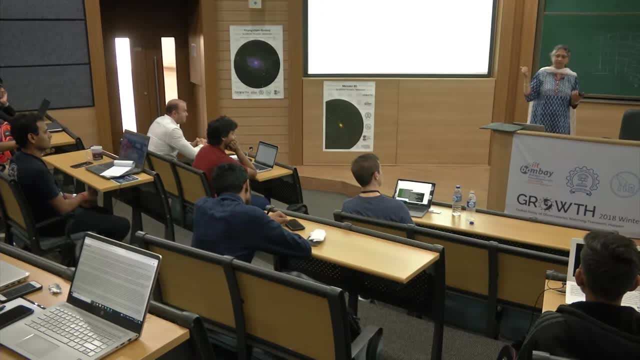 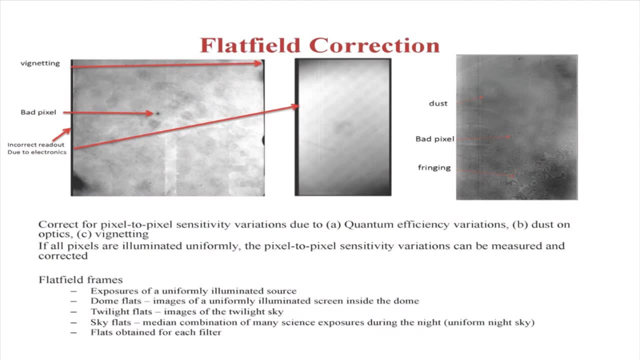 this will take care of the pixel to pixel variation. How does this take care of the pixel to pixel variation? Good, So let me just show you, for instance. let me go back to this here. ok, So there I have pointed out a bad pixel. ok, Suppose I take a row. 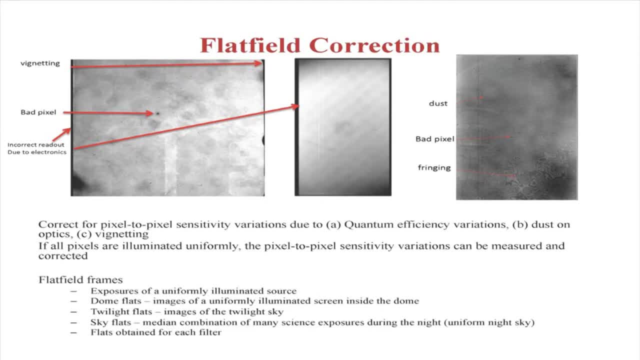 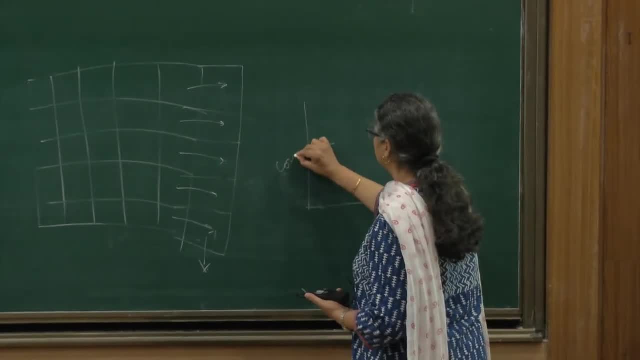 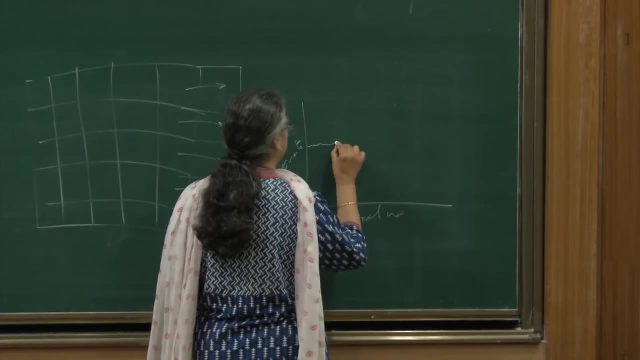 cut in a normalized flat what will happen. I have plotted in principle I should. if I take this as the counts, it is a number- it will go like this, but where the bad pixel is, you can see it as a dark spot. there We will have a dip pixel and this pixel. So 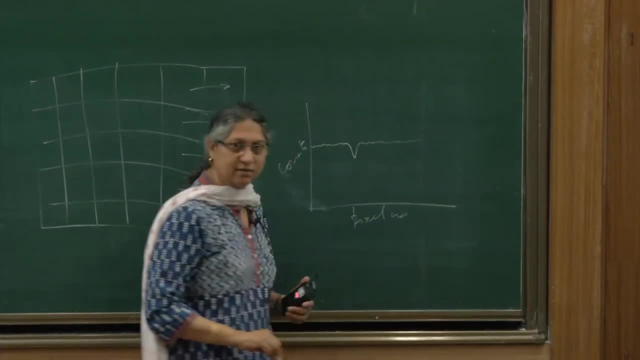 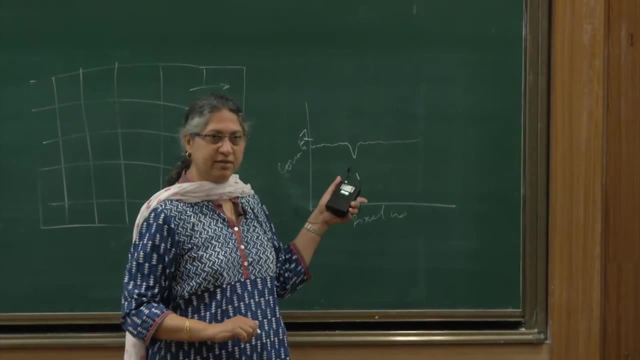 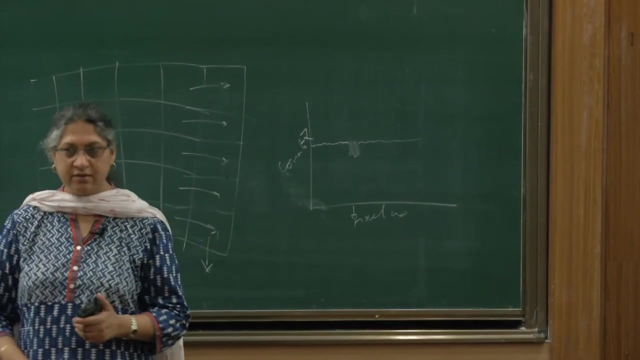 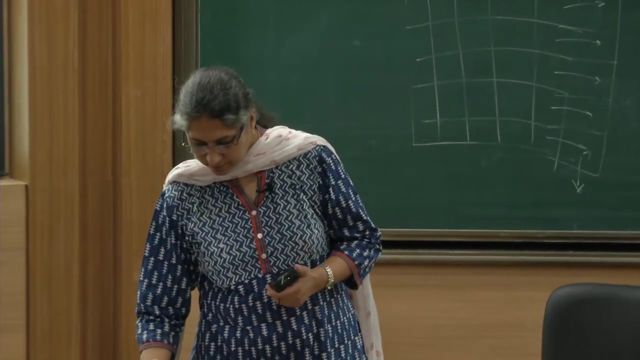 in the sensitivity and then it goes like that, right? So if this level is 1, when I divide by this along this row, this will get corrected for ok. So that is what the flat fielding does. this is how it corrects for the pixel to pixel sensitivity variations. ok. 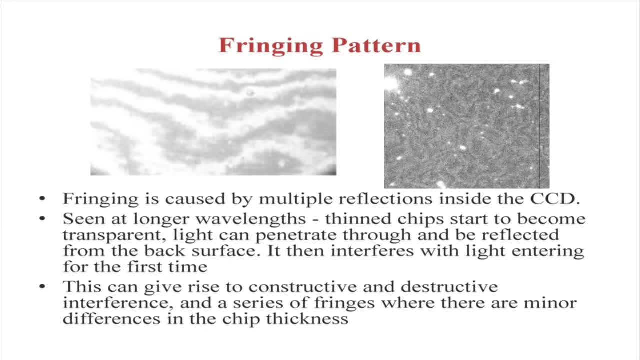 The next thing is a fringing right. how do you, why is this fringing happening? this is basically happening in what are called as a thin CCDs. You have multiple reflections in the, especially in the red region, and this can give rise to interference, which causes. 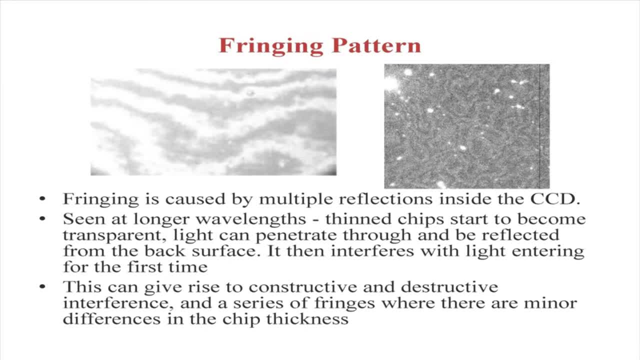 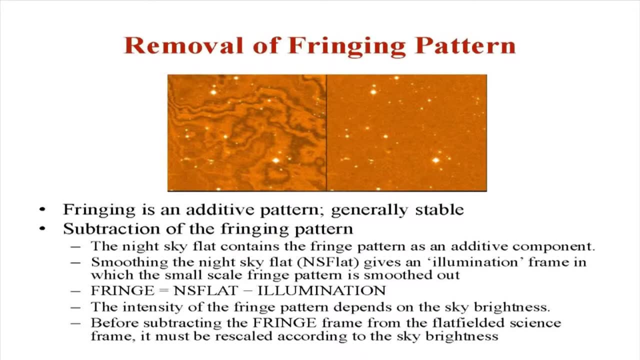 these fringes, ok, So how do you take care of the fringing? Fringing is again additive. So what you do is you take the fringes. you take the fringes, which are flat fielded images, and then you can- you can actually take the data itself. 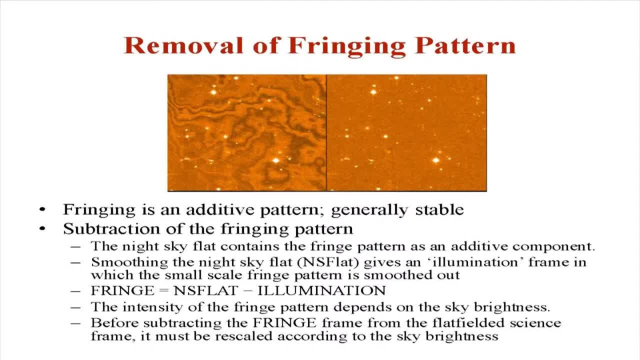 ok, Since this is, since this pattern is there in every single frame, you can use all the data for the night and then, in as long as you do not have too many bright sources in your images, this works out well. Then, when you median, combine them, you will be left with 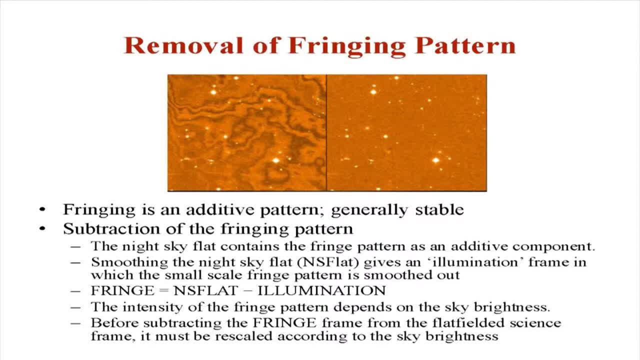 and then you can, you median, combine all your images, smooth it out. ok, So when you smooth it out, you you are kind of left with all the astronomical sources more or less smoothened out. ok, You have a sort of an image cleaned out of. 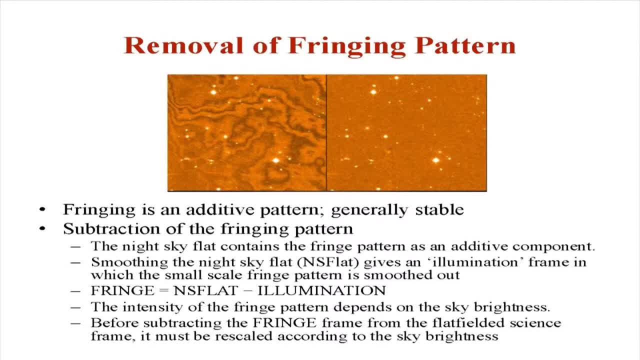 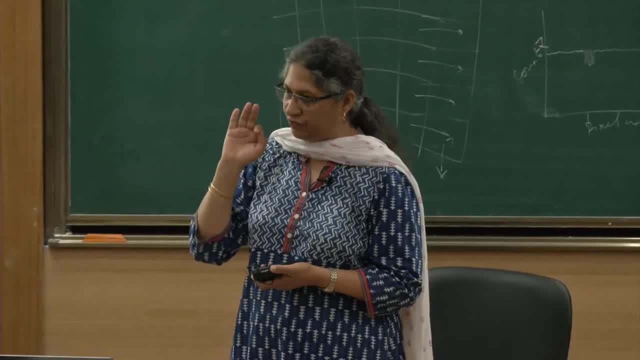 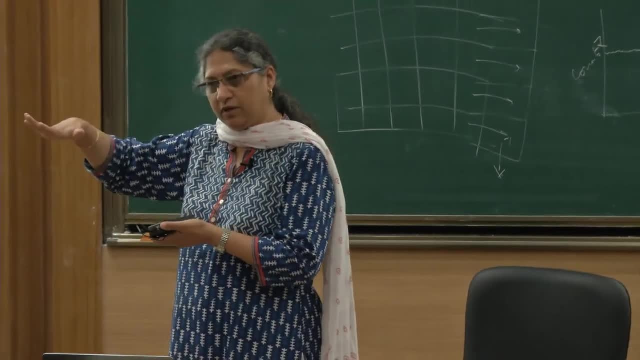 the astronomical sources. So this you can, you know, treat it as the night sky flat, for instance, So that you can take, And then the heavily smoothened night sky flat will give you this uniform background source, So which you, when you subtract it from this night sky flat, you 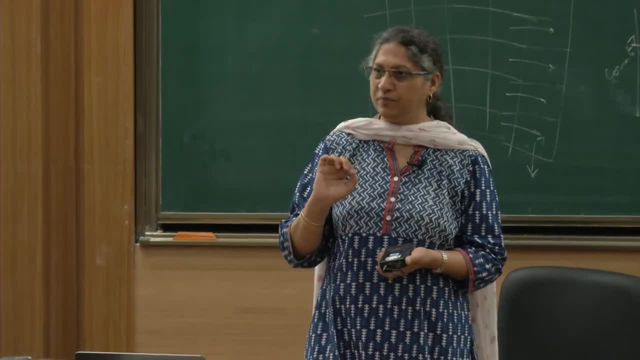 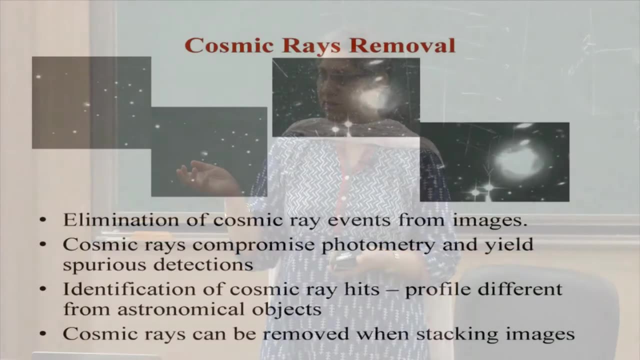 are left with only the fringe pattern. ok, So this you can subtract out from the images which have the fringing defect. The last thing that we can, we need to do is removing the cosmic ray events between, because these are not really associated with the fringes. 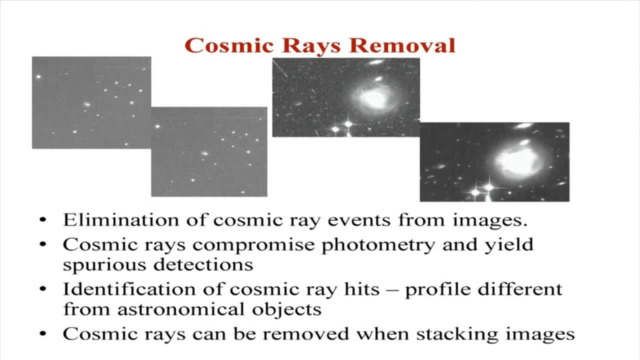 Yes, sir, with our source. here are examples. the first one is the HCT data where, fortunately, in this particular image, we did not have too many cosmic ray events affecting us, whereas the next set of images that I am showing are some HST images which I kind of picked up from. 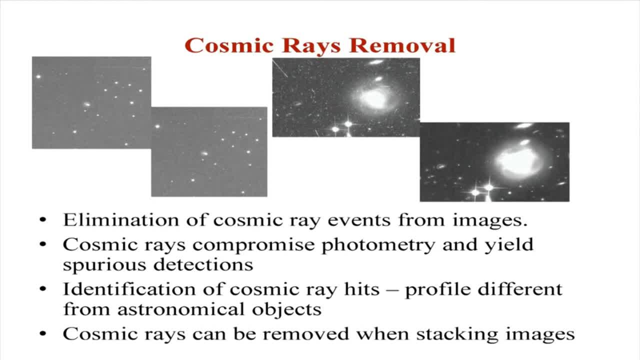 the net and there you can see. you know, you see a lot of small white spots all over right, those are the cosmic ray events and that when you remove that, you see it is a much cleaner image. We will understand more of the cosmic ray removal in the module. the basic thing is to 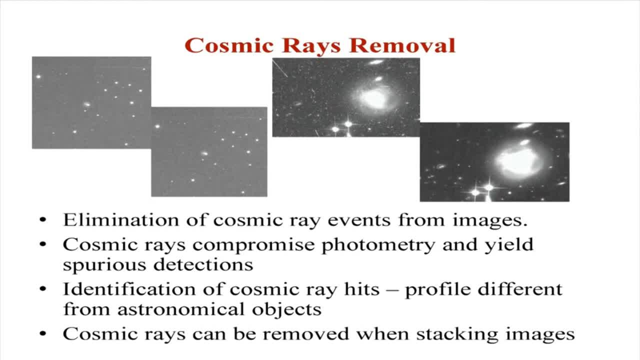 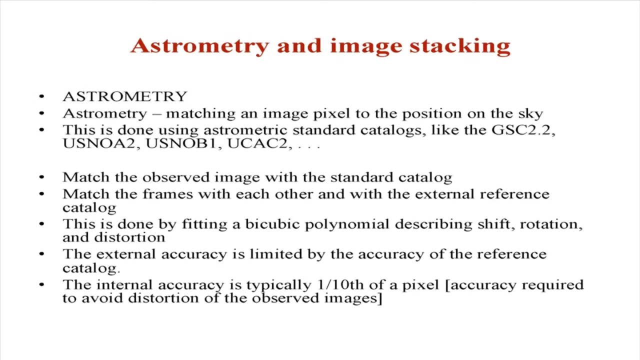 identify? how do you- I think yesterday Varun mentioned that- how you would identify, because you have these profiles which are very different from the object profile. so that is one way of identifying these sources and removing them. okay, So then astrometry, as we discussed in the beginning itself, this is nothing but matching. 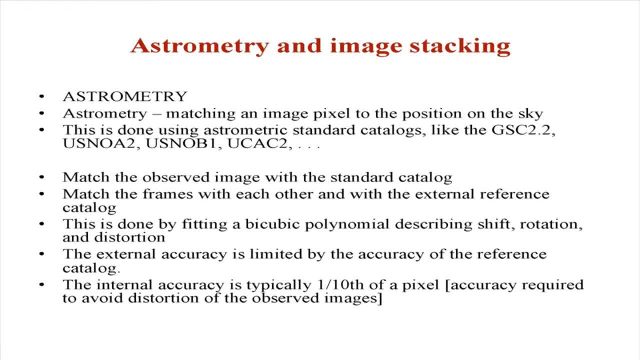 your pixel to the position on the sky. okay, So this you do by comparing with standard catalogs where the coordinates of the objects are known. So you identify your field with that and then you get these, then you are able to match them. So you can match your pixel to the sky coordinates, okay, 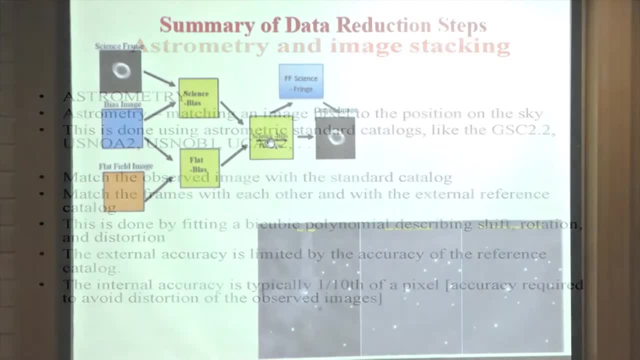 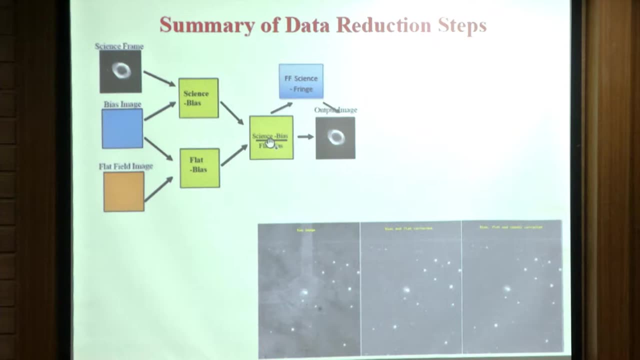 So this again will be there as a part of the module, and then you have the stacking. So, finally, this is the summary of the various steps that we need to do in image data reduction and which you can actually do now in the with the module. thank you. 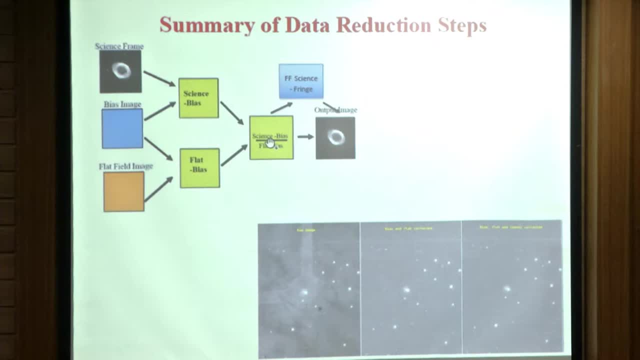 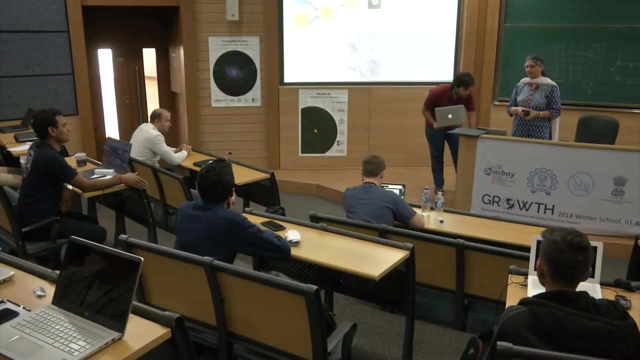 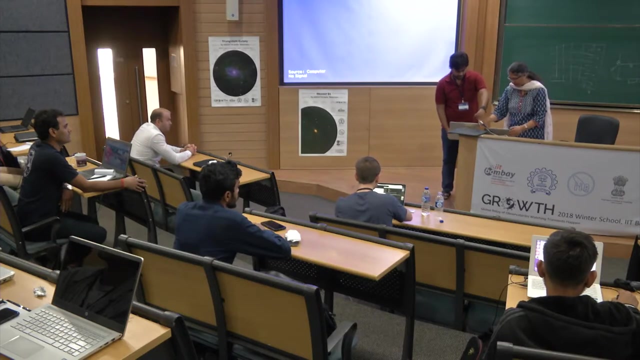 No, it is closed. yes, you, every night, every night. flats are obtained, biases are obtained, okay, and you can. if, for example, you are observing a transient source and then you know there is no flat obtained for that night, you can probably use the nearest night. 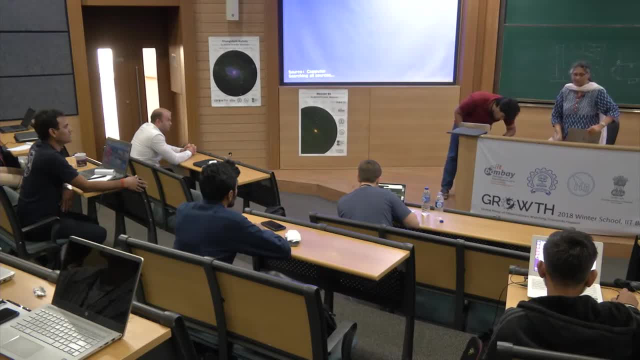 Okay, Thank you, Thank you, But in principle, the best way of doing it is that it is done that way. for instance, what we do with the 2 meter HCT is that every night and every morning, during the evening twilight and the morning twilight, flats are obtained in all filters, irrespective of what the observational 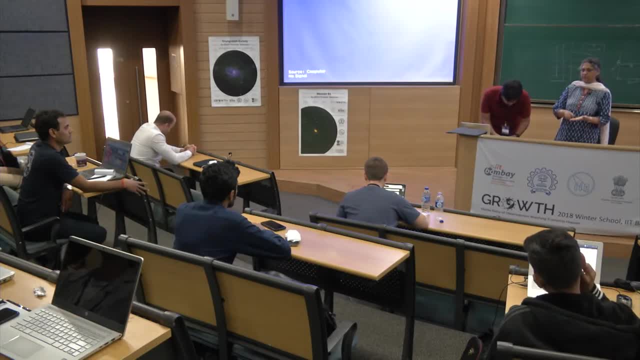 program is for that night. whether it is spectroscopy or photometry, whatever is the proposal, we do not care, but flats are obtained every night. okay, So this can be used by anybody else also. Okay, So whatever data is obtained in that night, you can also. you can do that in what? 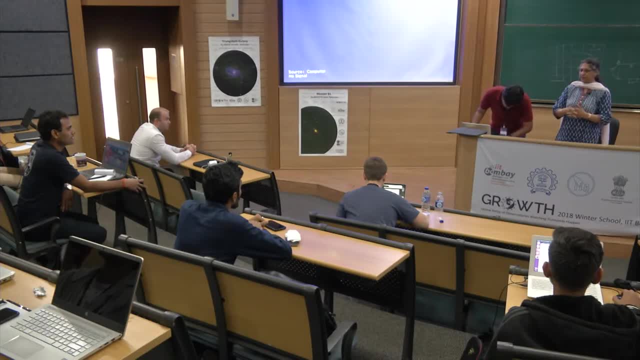 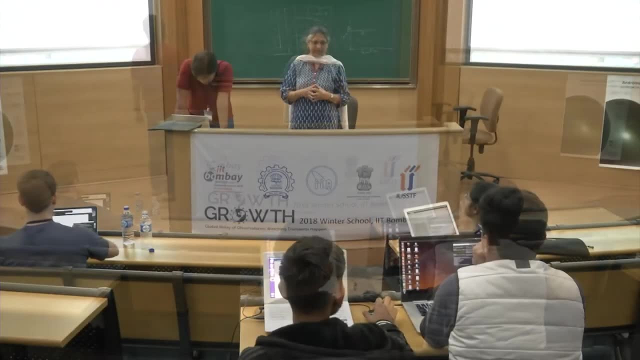 Space telescope. Space telescope: yeah, the calibration frames are obtained, but there you can use the night sky to get the flats. why the sky flats are more preferred than the dome flats? Dome flats can give rise to certain other kinds of problems. one is like, if it is not, 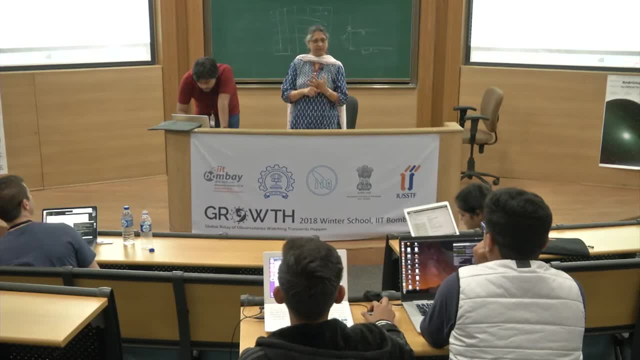 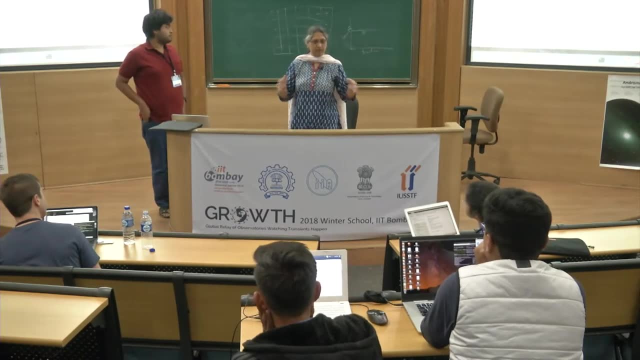 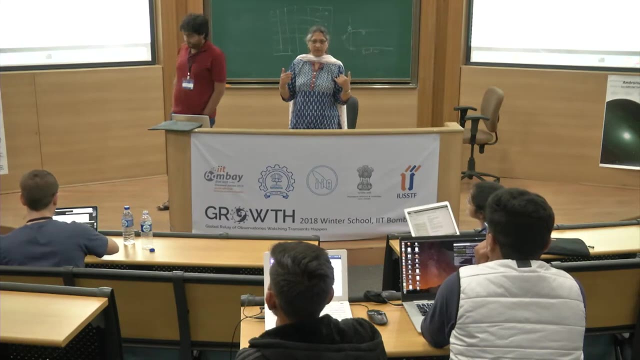 you know, properly designed Okay, Then it can have issues of not being able to illuminate the full mirror, for instance. then you do not really have a uniform source of light. And the other thing is it is always good to have more or less the same the light goes. 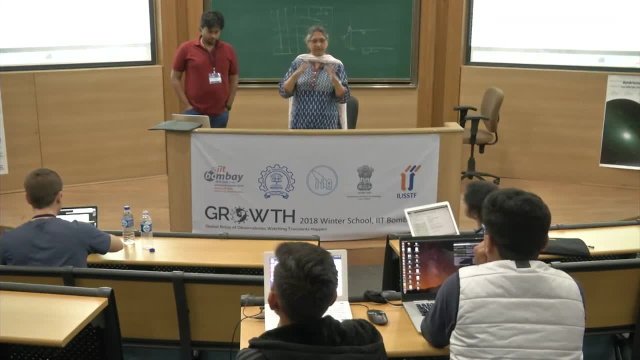 through more or less the same path as your object. okay, in which case you need to have lot of optics which will give a similar F ratio when you are observing the dome flats- Okay. And the other thing is that you are using an artificial source here, which may not really. 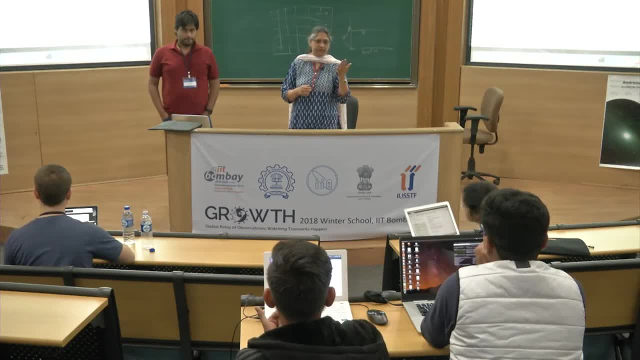 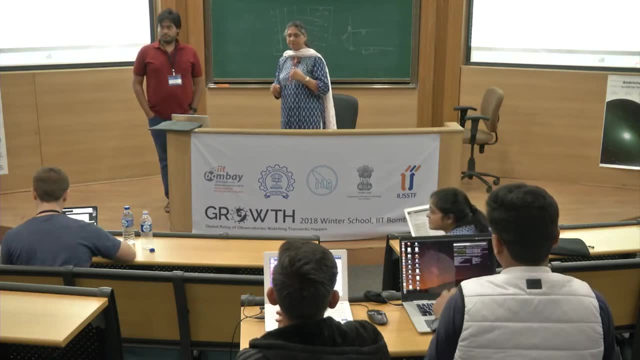 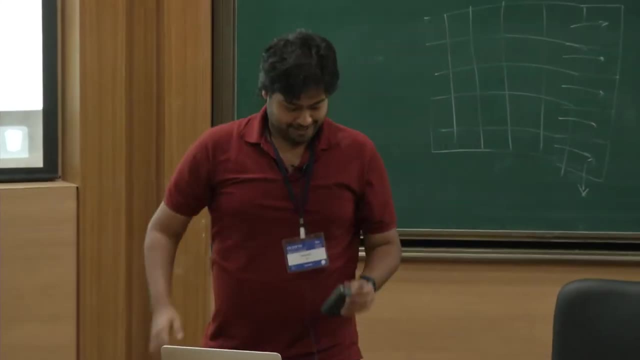 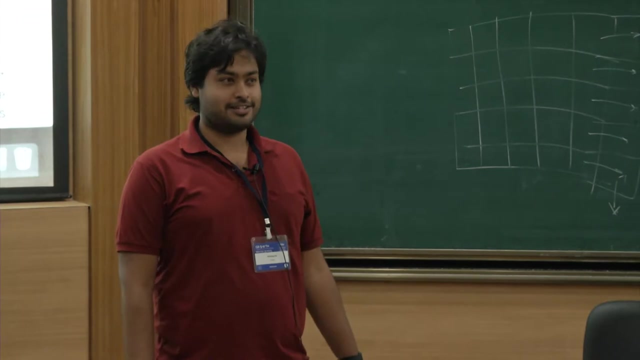 be uniform and across the wavelengths, okay, so you might have issues with that too. Discuss later. Okay, right, so first question: did everyone get a chance to download the updated version of the module that was sent out last night, Right, No problem? 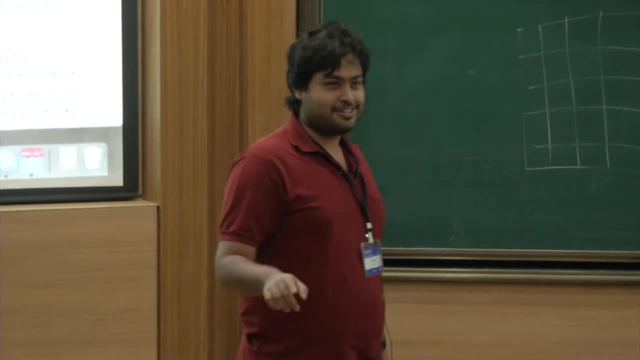 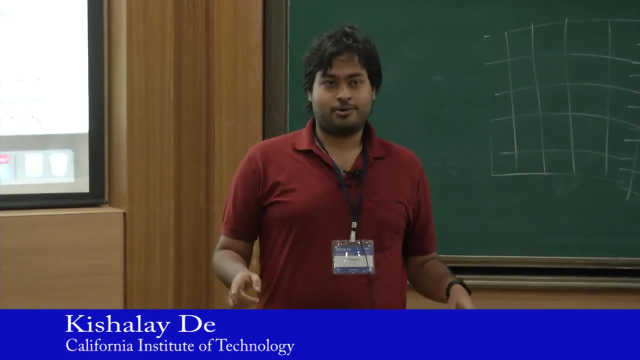 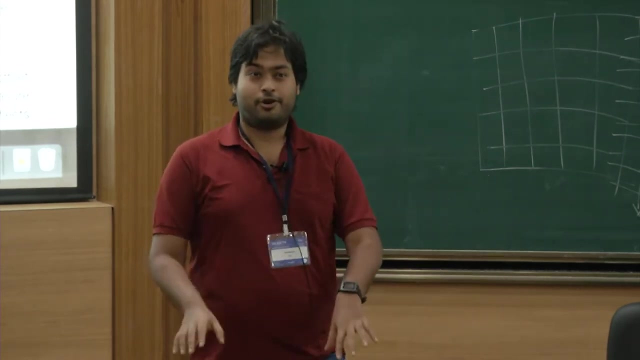 No problems with that. There was another email sent out this morning about installing: yes, right, yes. so for today's module, based on what happened yesterday, I think there was some confusion about the paths and everything, so I have decided to run everything on my laptop from the docker that you all should. 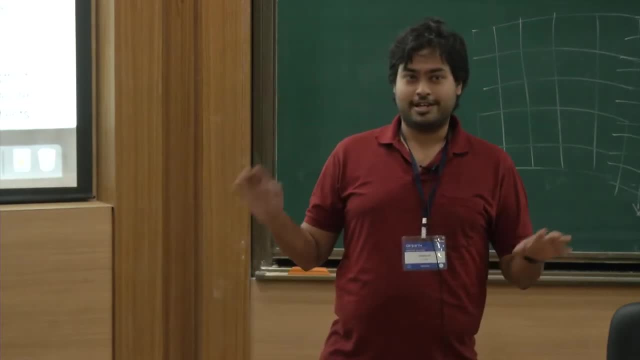 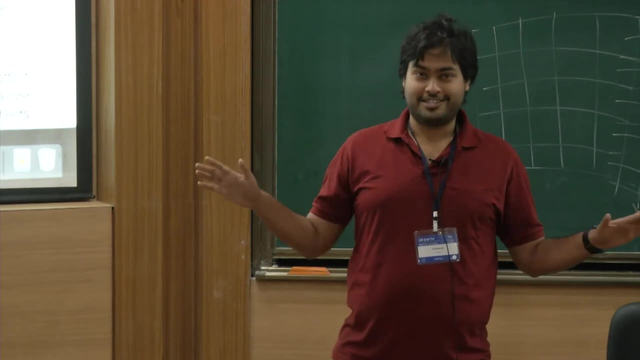 be running, So please try to use the docker that was supplied to you, because it has all the necessary software that we will be using in this module, and I will be running on the same docker, so in principle, we should have all have the same paths. 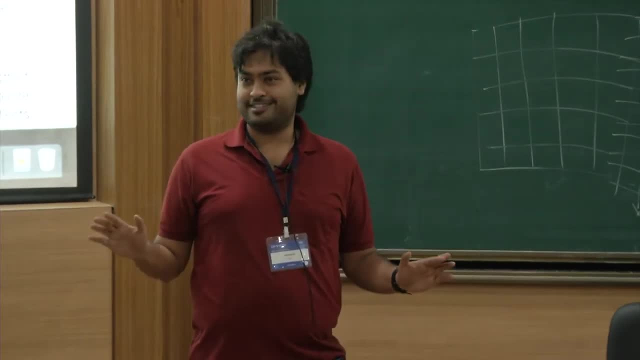 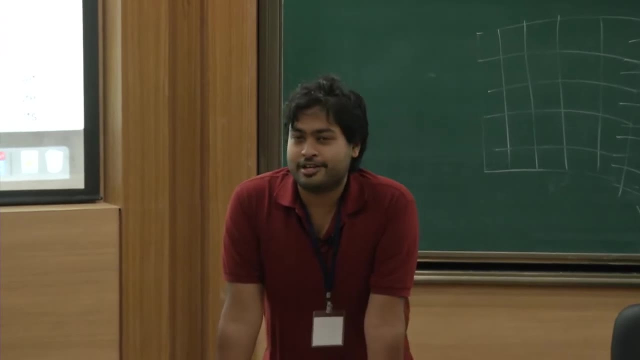 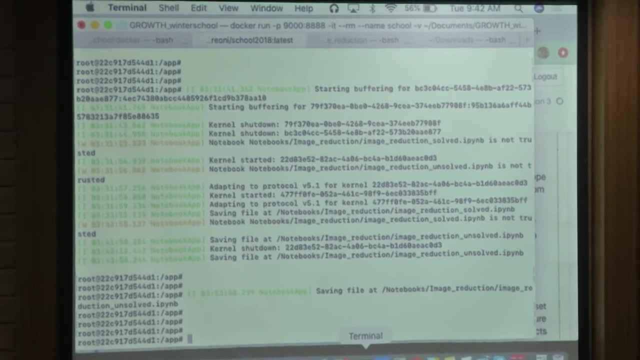 So, whatever path I said, you can set the same path and we should get the same results everyone. So just to. so I sent out an email earlier today about installing these two additional modules, so, in case you haven't had a chance to do that, just in the terminal that is running. 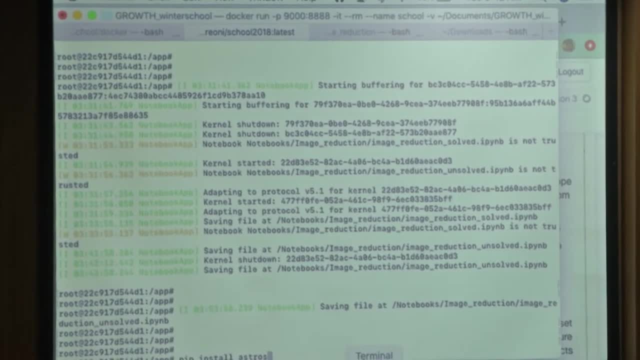 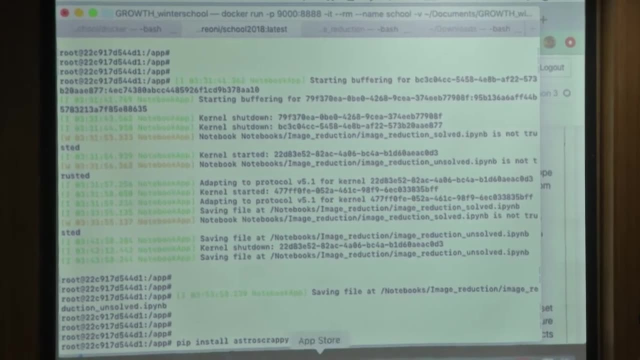 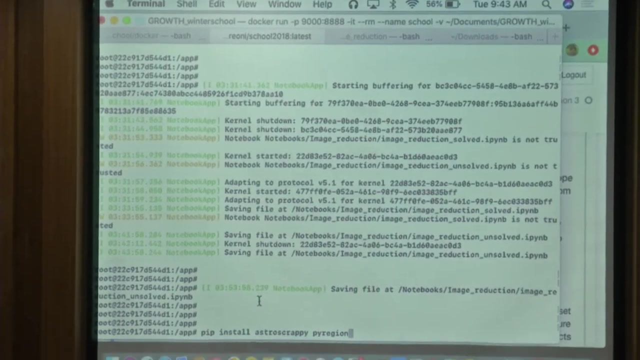 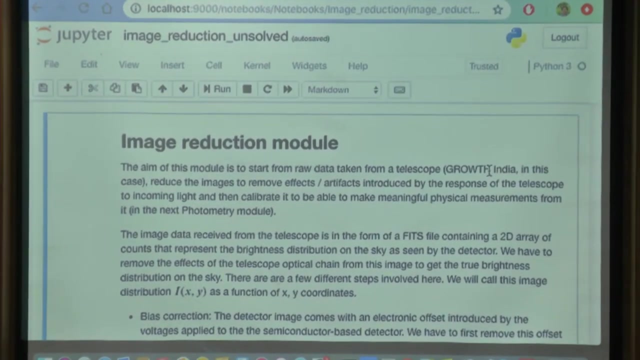 the docker just type pip, install. So these are Sorry. These are just two modules that we'll be using in this session. so it's you can just run it from the terminal and it should work. okay, right. so when you get a chance, please open. 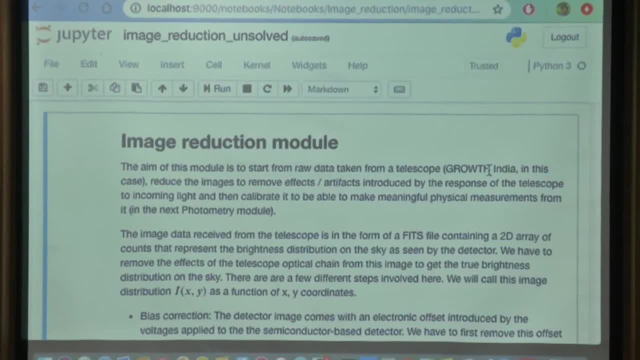 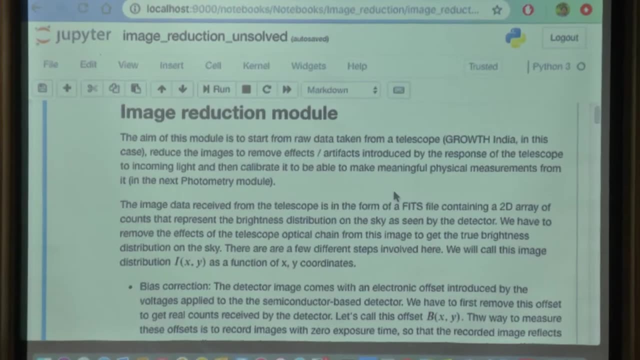 up the unsolved version of the notebook. the solved version is only for me to cheat from. you should use the unsolved version to start off with the process of image reduction. so these images, The ones that we'll be working on today, these are actually taken with the growth India telescope. 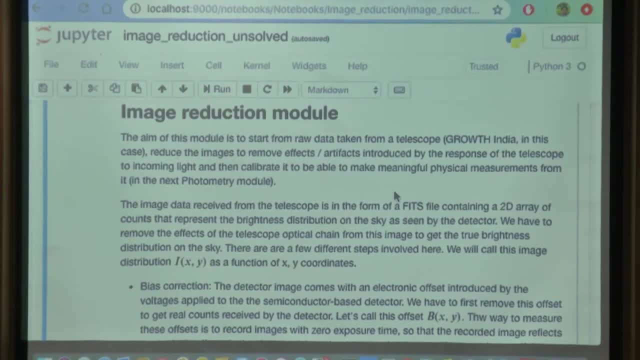 except these are not images from the last night, these were taken about a couple of weeks ago- but they will demonstrate the general process of image reduction and in this case, we're actually looking at a field that contains an interesting variable style. so- and you'll be working with this- the light curve of this variable style in the future light curve analysis. 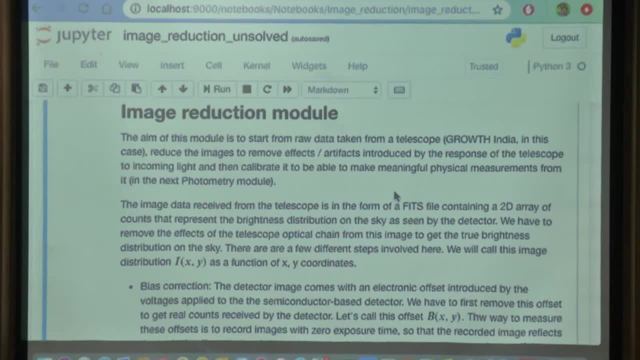 module. so just so you know where all that photometry comes from, we'll actually be reducing this data to show you how you get from a raw image- Okay, That comes from the telescope- to a reduced image where you can extract photometry from. 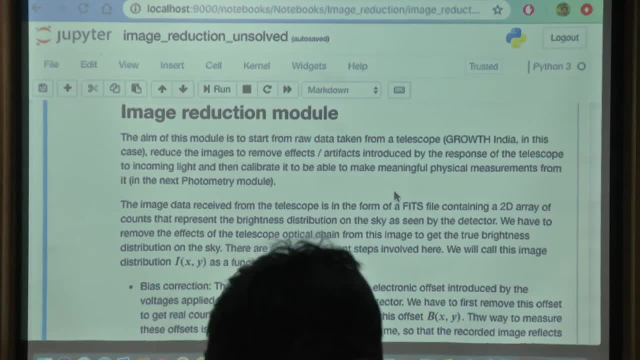 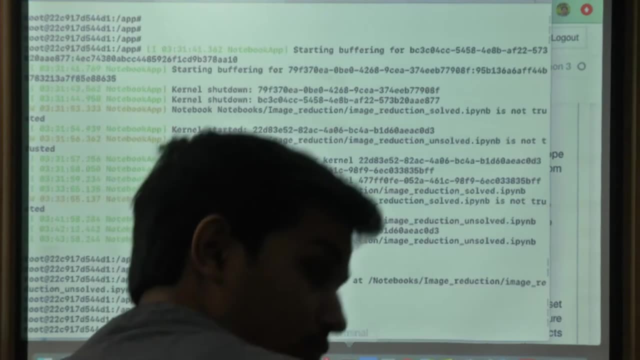 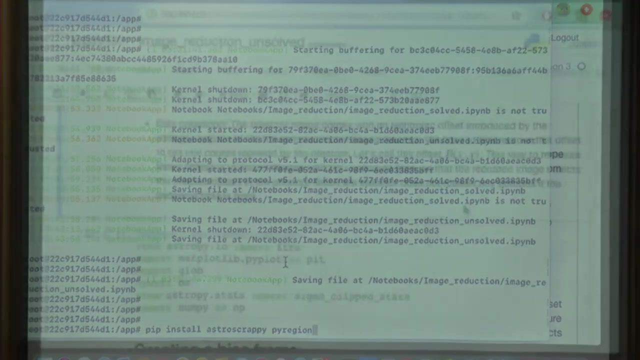 which is the subject of the next module. so I'll just wait a couple of minutes, in case you haven't had a chance to download the notebook or run this command. so just run this command and you should be able to install the modules that will be needing. so perfect, so the first. 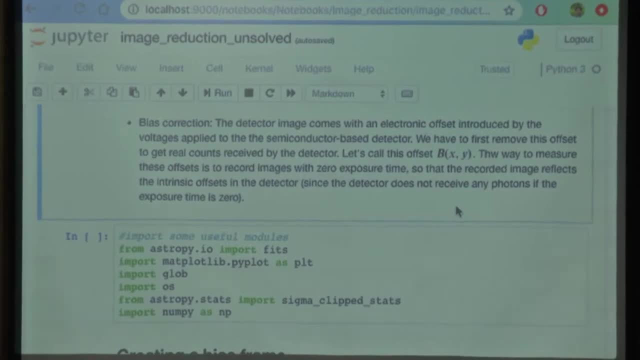 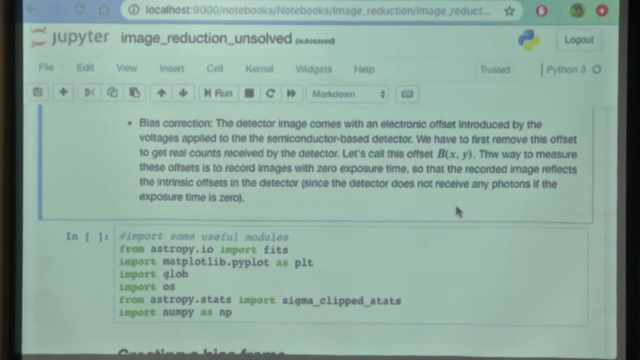 thing that we'll do is, as Anupama has already mentioned, is to create what is known as a master bias frame. So the idea is you take exposures with a telescope with zero exposure time to subtract off the offsets that are introduced by the detector, which are: which is not, ah, which does? 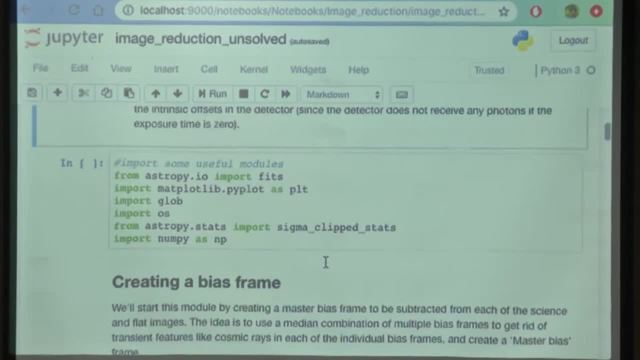 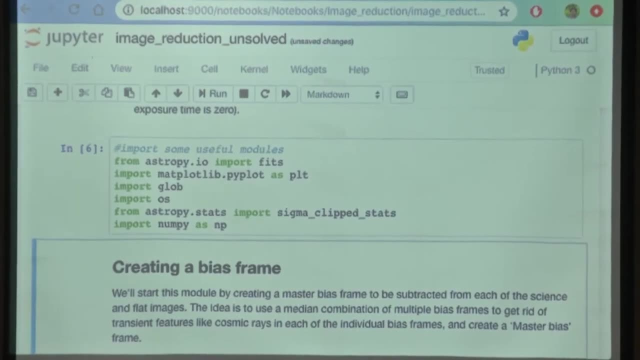 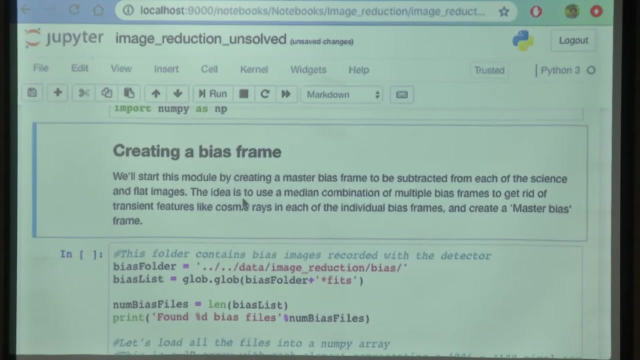 not reflect the true brightness distribution on the sky. so we start with just importing a few modules, So this should just work smoothly. ah, we're just importing some modules for plotting and for doing some statistics on the images. ah, Okay, Okay, Okay. 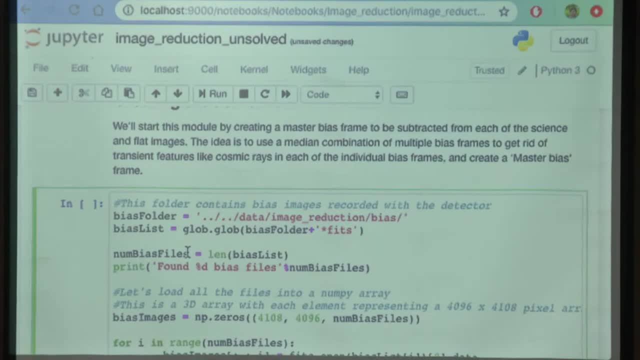 So if you move on, ah, to the next cell, so just make sure your path is set to this. this is exactly the path that should be there in the docker. so if you set this path, it should work. ah right, so once you've done that, what I'm doing here is just I've- I've sorted all. 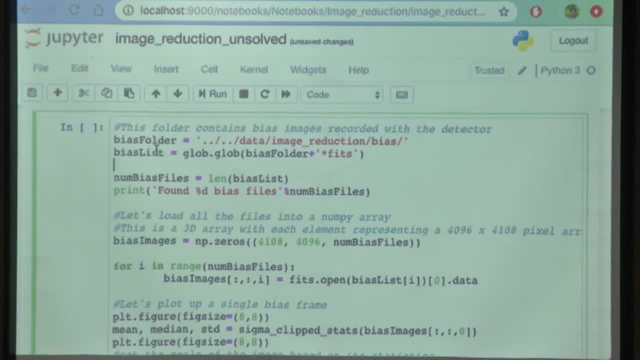 the calibration files into folders. so I'm just reading the files that are there inside inside that folder and then loading them up into this numpy array. So this is a three dimensional numpy array with the images stored in, ah, the the multiple bias images stored in as different elements in the array. so, um, this is so if you run. 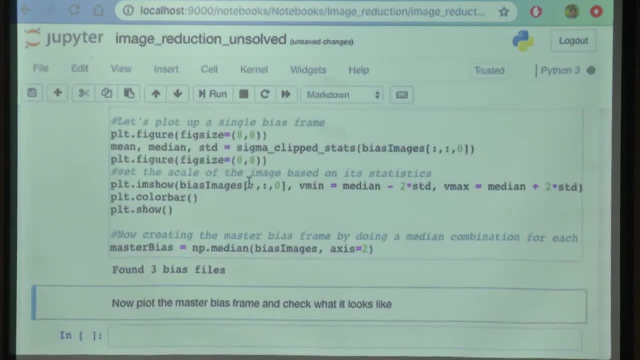 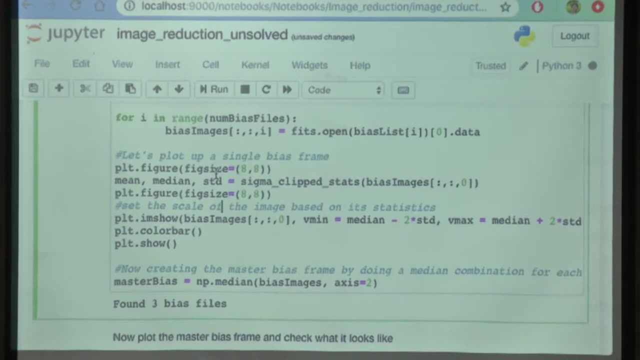 this: it should say there should be three bias files that are there in the folder, and then it will: ah, once these files are loaded, I'm also plotting up one image, ah, one bias image that was there in that folder, just to show you what a typical bias frame from growth. 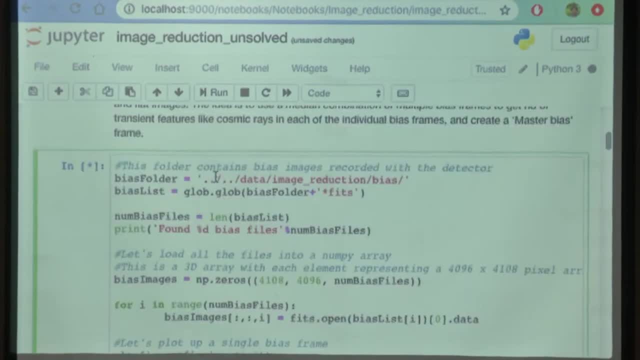 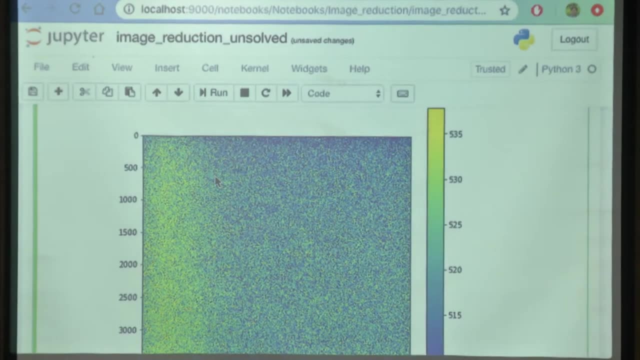 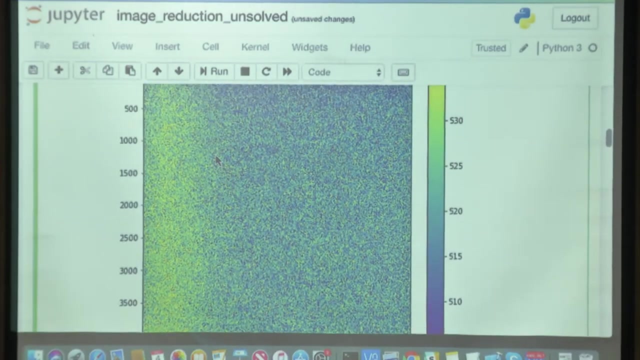 India. looks like this can take a bit, but should come up. Yes, Okay, Okay. So this is the path. Yes, Yes, Look the path, Okay, Ah, So does everyone have this single bias frame plotted up? 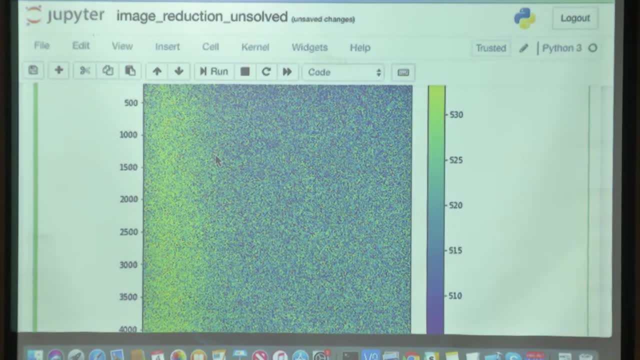 Does it look okay? Okay, Ah, Right. So I just wanted to notice the general pattern on this bias frame. So, as you can see the offsets, they vary with the position in the detector. So the left hand side of the detector has a larger offset. 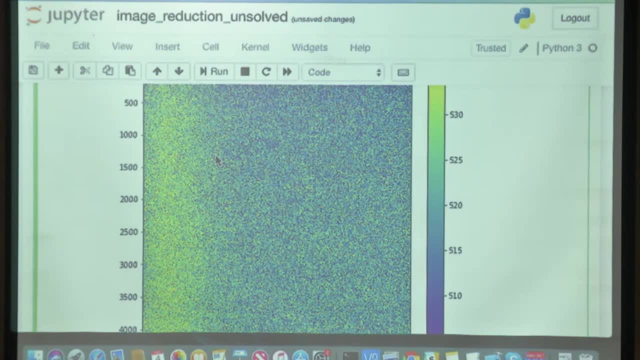 So the bias values are larger over there, whereas the right hand side has lower bias value. So we have to subtract this offset off from the real images. So just keep this pattern in mind. We'll see it later in the actual images. 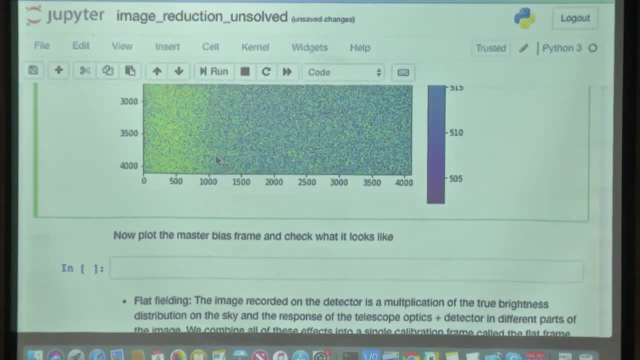 Um, Right, So the next one is just an exercise for you. We did create a master bias frame, So if you see, ah, this array called master bias right here, Can you try to just plot this master bias using. well, basically the same, pretty much. 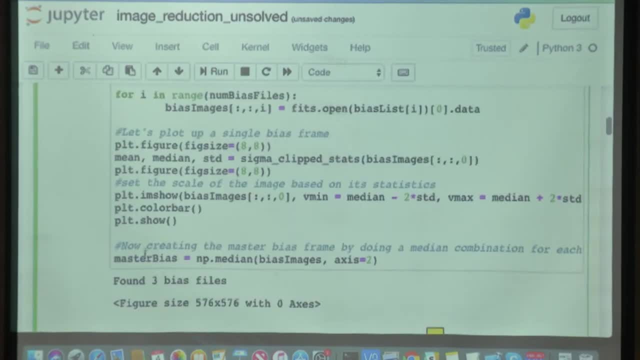 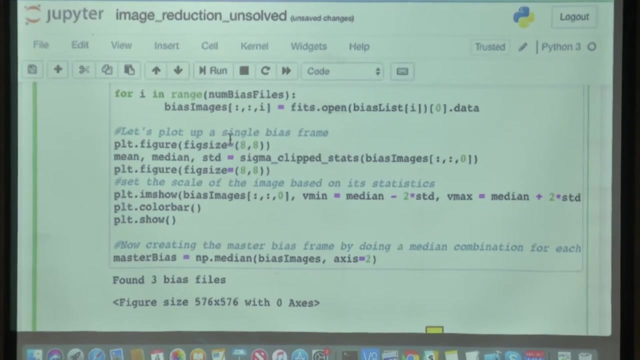 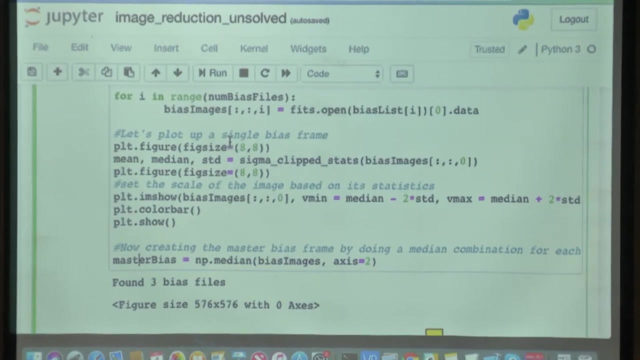 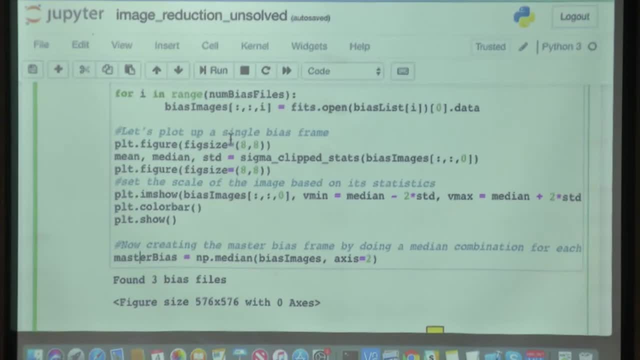 Also, just so you know this, what this command here is doing is that so we have all the bias images in one array, which is a three dimensional array, and what you are doing is we are asking numpy to stack along the images- Right images, So that what you get effectively at the end of it is an image which is median. 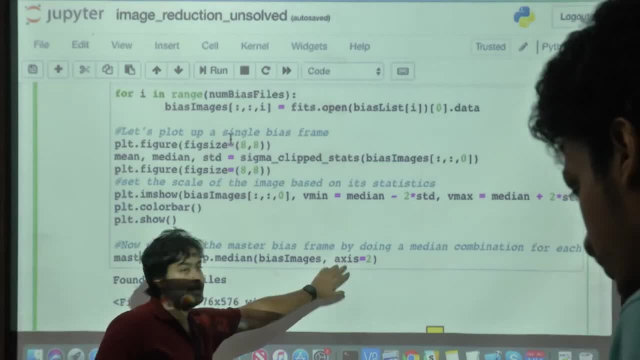 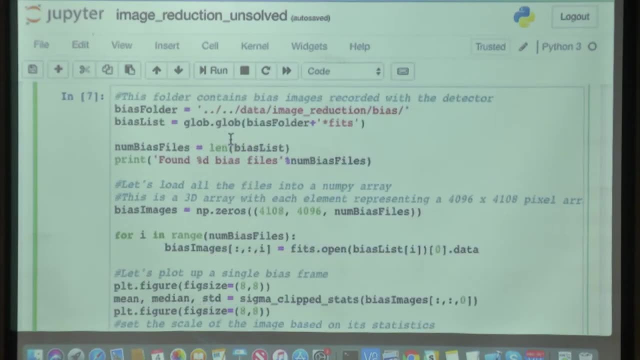 combined from all of the individual bias images, which is why this parameter axis, equals to it, stacks along this specific axis that we asked for. ok, So how many of you were able to plot the master bias? ok, perfect, ah, ok. How many of you are having trouble plot plotting? 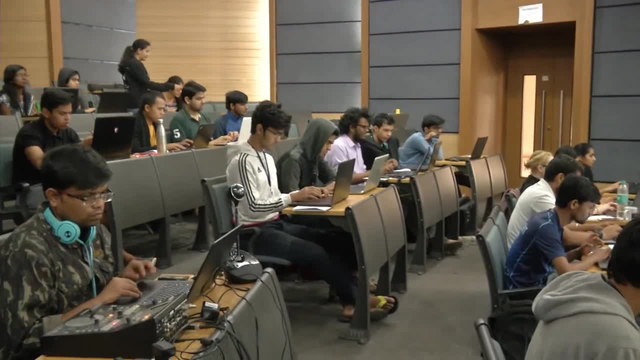 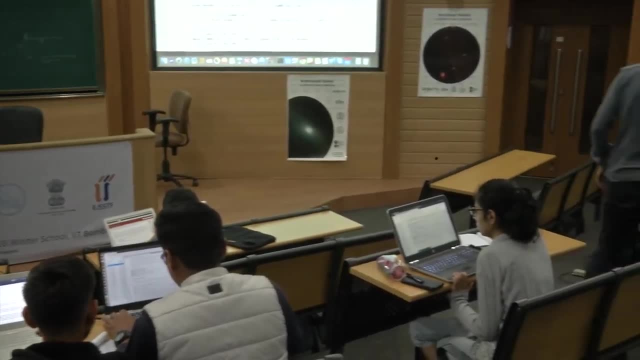 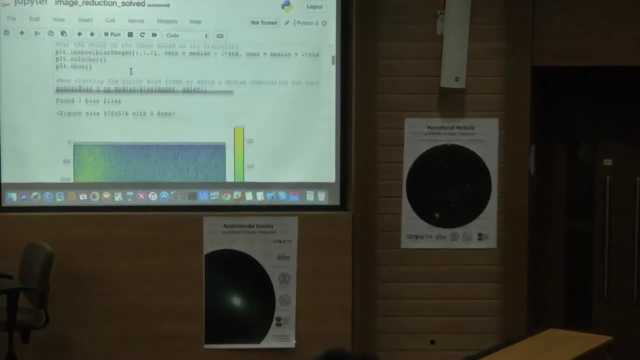 the single bias. Any major issues yet with plotting the single bias? Ok, I think I am going to move on, So let me just show you what the master bias looks like. I will just. yeah, I already made the master bias, yes. So if you look at this command, 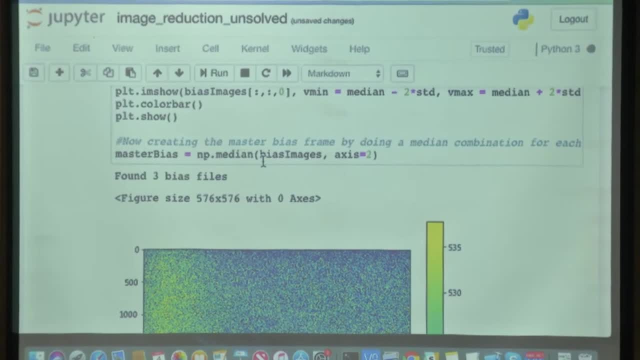 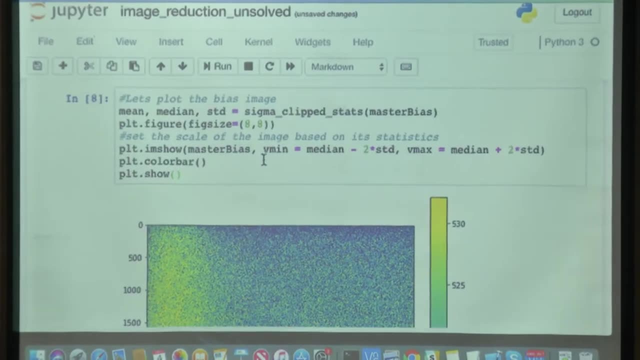 this is what this is doing. I did a median combination over all the bias images, So you just have to plot this. yes, yeah, ok. So this is what the master bias looks like. as you see, it is pretty much has the same structure as we saw in the single file. 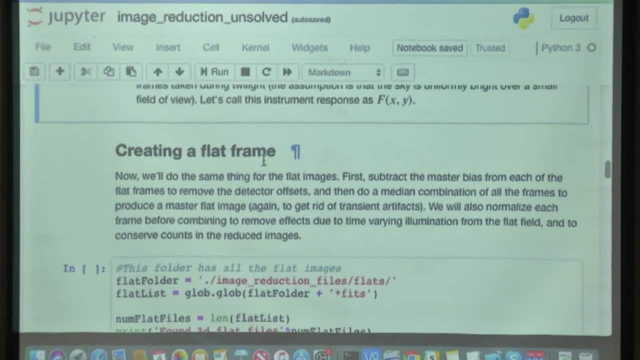 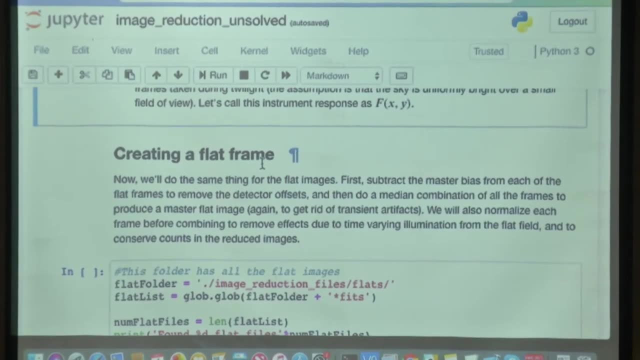 Ok, So right, the next part comes. that comes is the flat fielding. So, as you already heard, flat fielding is about removing the pixel to pixel sensitivity variations to make sure that the image of the sky that you are getting does not reflect the sensitivity of the telescope. 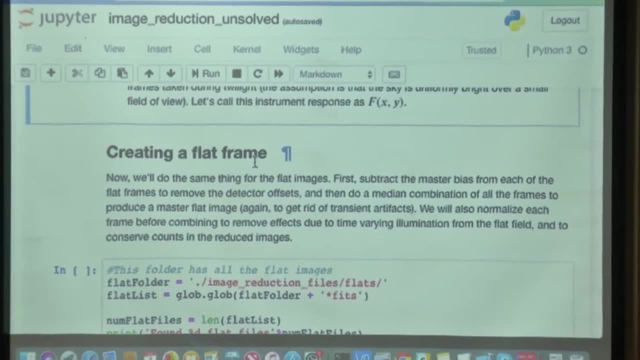 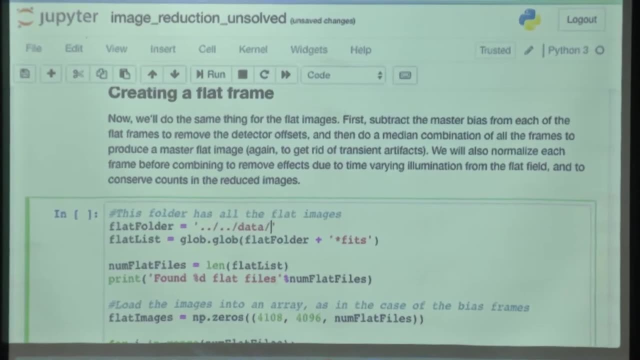 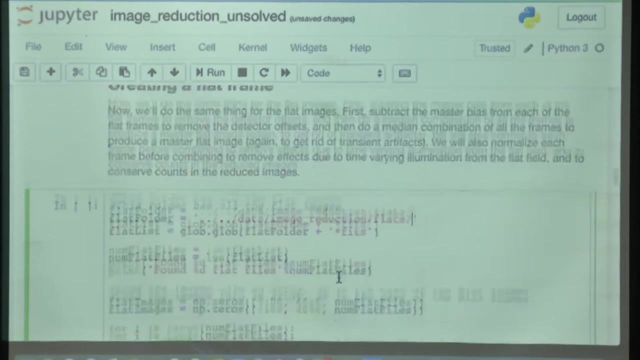 and the detector combined in the image. So, as before, I will change this path. the path in this case should be: So just copy over this path. ok, So as before. it is exactly the same path, except it is a different folder. it is instead. 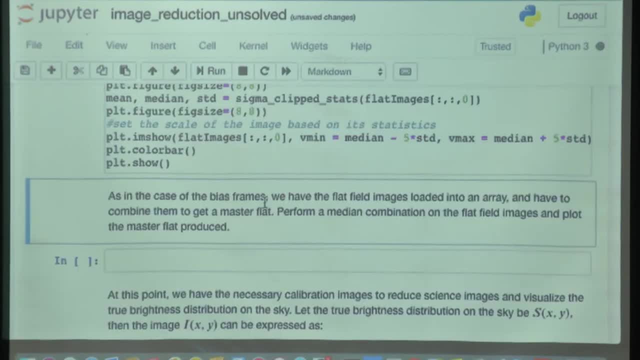 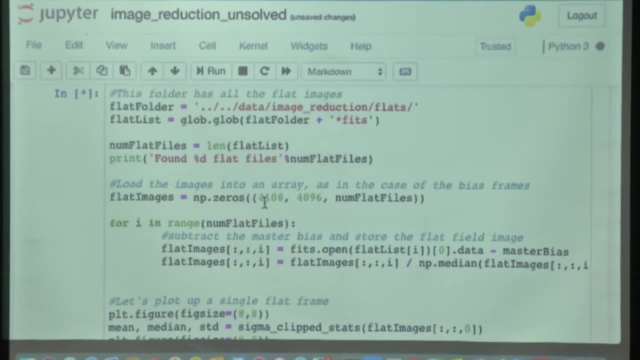 of bias. it is in flats now, So if I run this, it should show up what a single flat frame looks like. So just to walk you through what is going on here, I am again loading up all the flats that were there in this folder and then I am subtracting off. first the master. 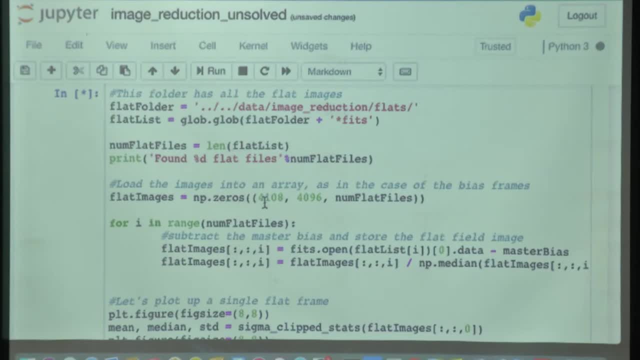 bias. So the flat itself also has the master bias offset inside it and you want to remove that before we do the flat combination. So I am taking one image, which is the flat field, subtracting the master bias and then normalizing it. So ok. So again, I am taking one each flat field image which 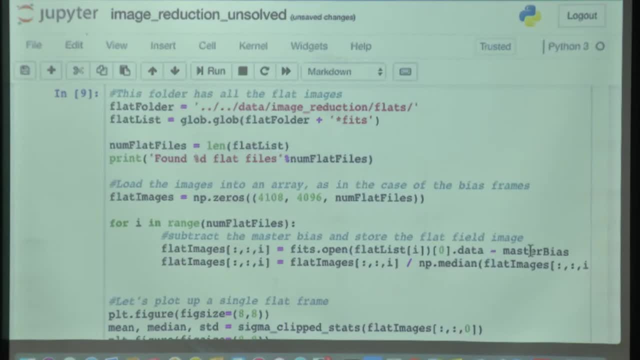 is in this subtracting of the master bias and then normalizing the flat by its own median, So that, irrespective of what the actual counts in the image were, everything is now normalized to the median counts in the image. Any questions about that? Why this is doing that normalization? 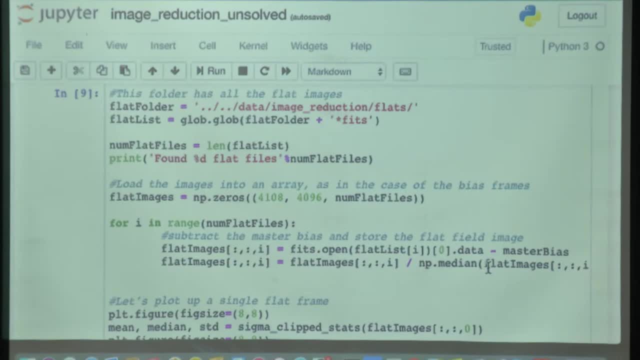 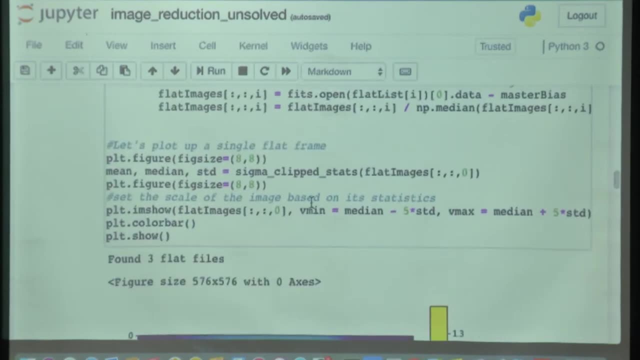 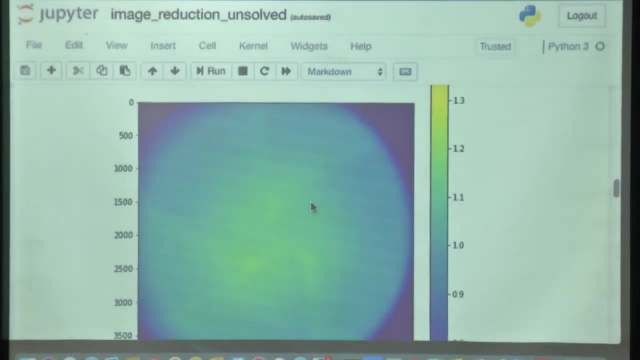 I am just subtracting, I am just dividing the entire image by its own median, and then I just plotted up. I basically use the same command as I did for the master bias. In this case I am just plotting the flat frame. So this is what a single flat frame looks like. 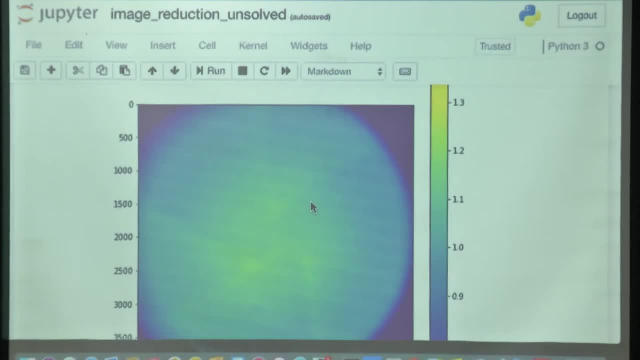 Did. how many of you got to this step? Ok, Perfect, Ok, So just take a note of the count. So you see all of the counts in the image, the color bar. they are normalized to 1. So its everything is normalized respect to some 1 value. Ok, Any major issues in running this yet? 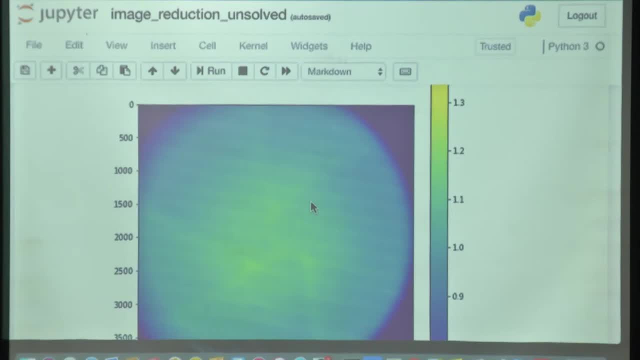 Ok, So It is again because the median is always more robust to outliers. So imagine: if you have a cosmic ray somewhere in the image, then a mean will always be affected by that cosmic ray. It might just produce a weird value for the mean, whereas the median 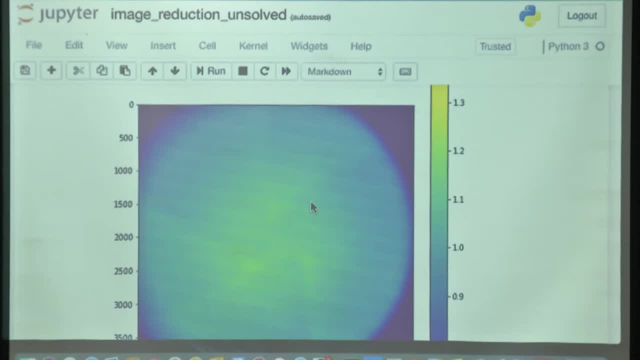 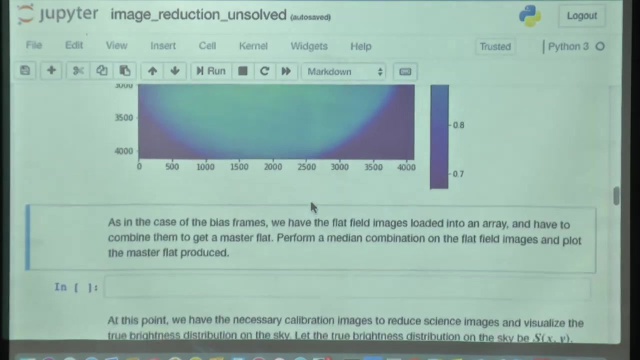 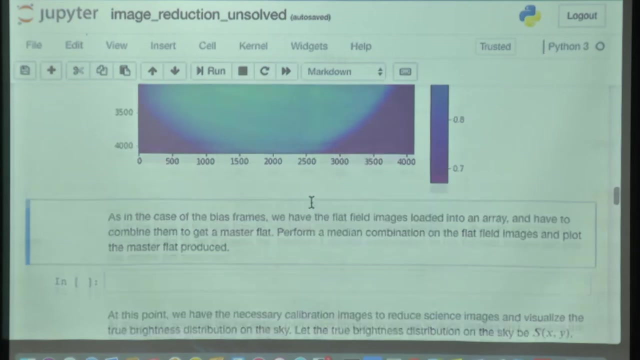 is much more robust to outliers. Sorry, what? Ok, Ok, Right, So the next exercise is to just do exactly the same what we did in the master bias frame Plot, the master flat frame. So in this case I have left it as an exercise. 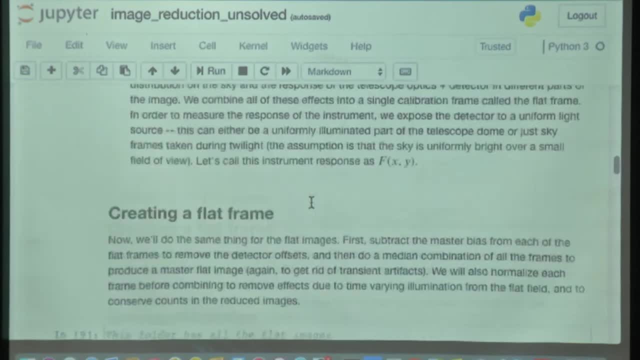 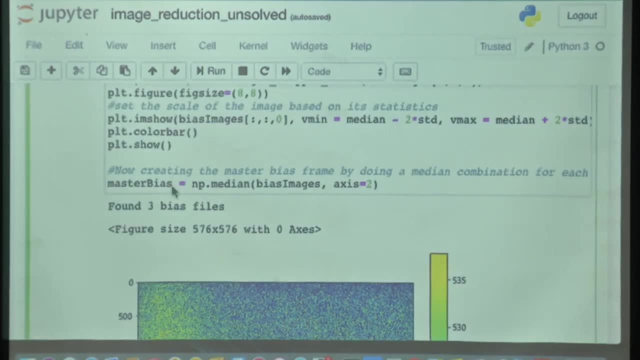 to actually produce the master flat frame. So what you want to do here is you want to go back to this command here which does this master bias equals to this median over this set of images, and you want to repeat that to create a master flat frame. 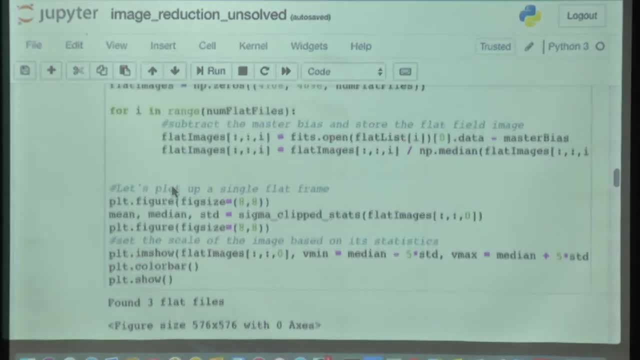 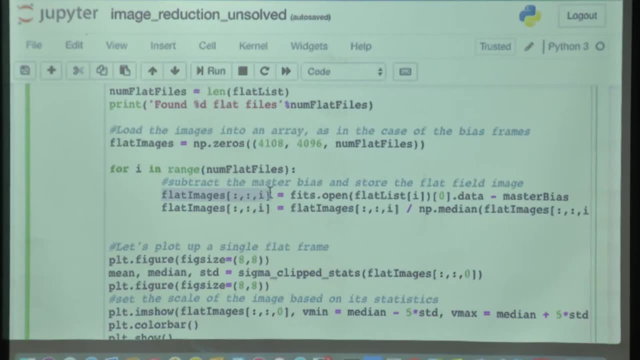 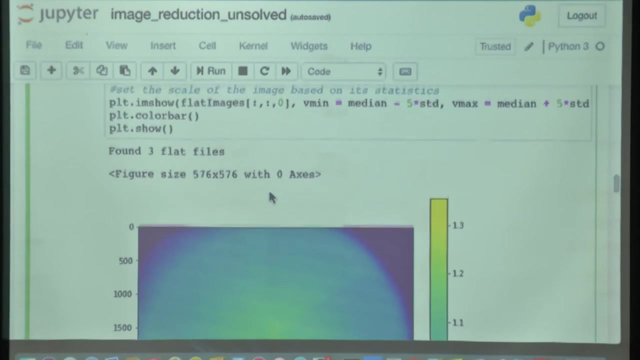 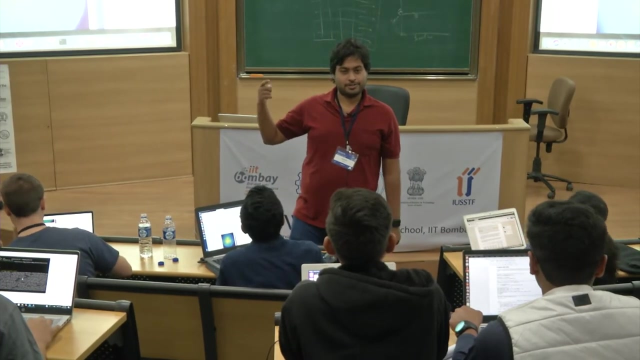 Yes, So just note that all the flat images are stored in this array, So just make sure that you are running a median combination over these images for the flat frames. Yes, that is. that is a bad column. that is just one that Manupama mentioned about. 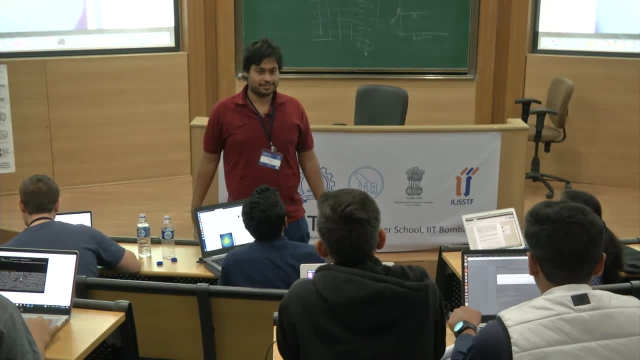 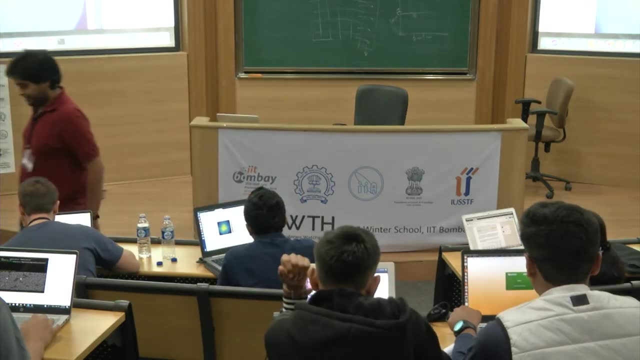 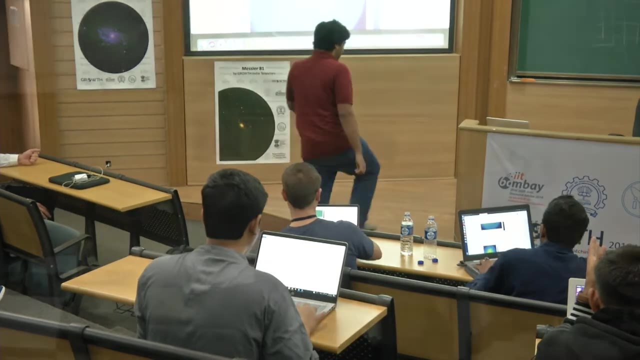 where you can have electrons accumulating for no reason, says the defect in the detector. So all detectors have some level of defects. you just seeing that? Yes, Yes, So, okay, So let me. So some people are worried because they are seeing a single line in the image somewhere. 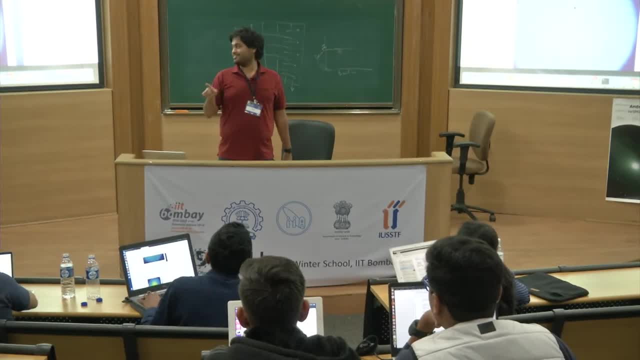 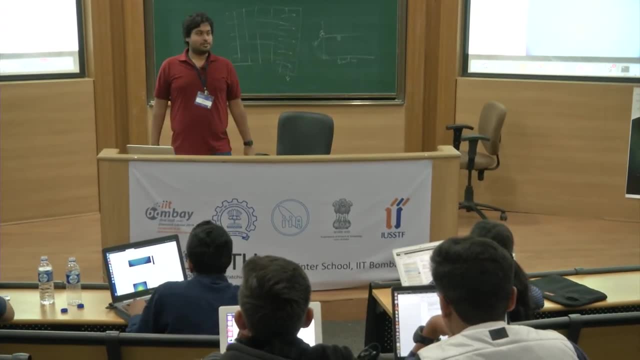 that is a bad column. that is a known- at least I think it is a known- defect in the detector. So it is one of the defects that Anupama mentioned, which is which can happen because of electrons accumulating at some specific location. So those are bad columns and in a real image reduction you 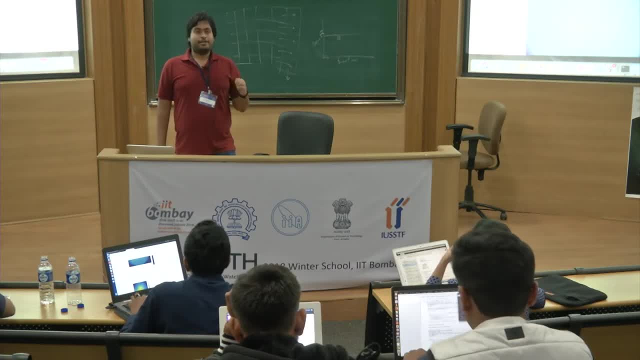 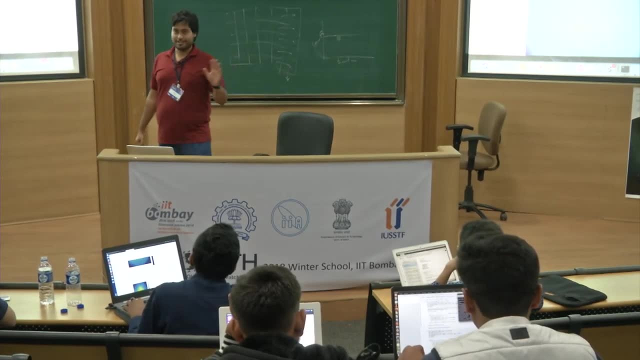 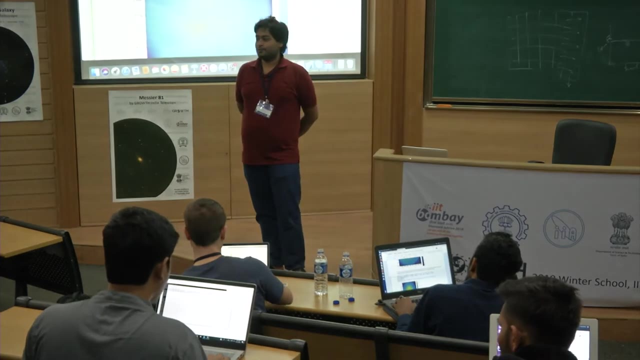 would actually account for them. you would have a. you would typically previously know where the bad columns are. So you can not observe your sources on top of that bad column. you do not want to do that, Not always. sometimes those bad columns are just too bad. you cannot remove them, you just want. 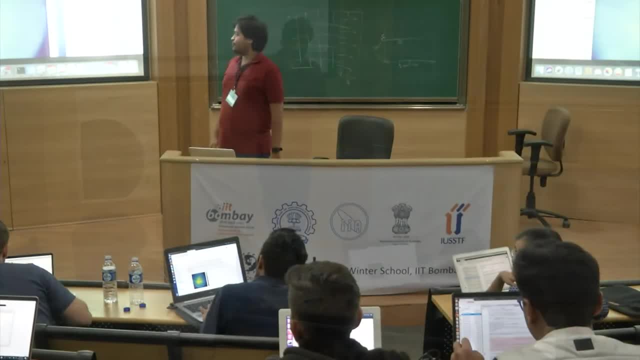 to keep your sources of interest away from that bad column. Yes, Okay, So I am going to go ahead and produce this thing. Okay, So I am going to go ahead and produce this thing. So I am going to go ahead and produce this thing. So I am going to go ahead and produce this thing. So let us whatever it should. 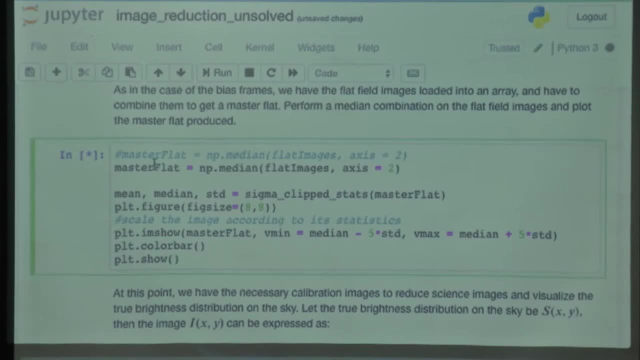 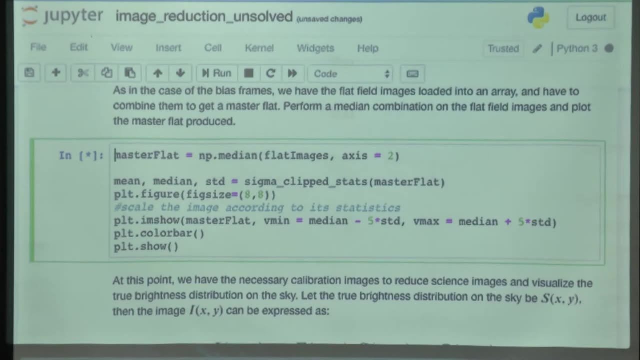 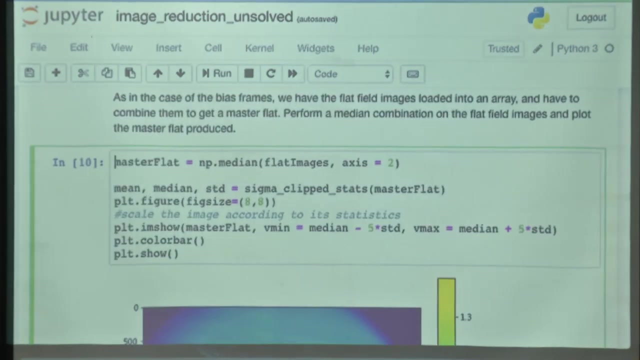 be medium, Okay, 3.. Yeah, I can, I have. it is the docker. I do not know why it is Yes. So this is. so if you run this command, which what I am doing here is again taking the flat images. 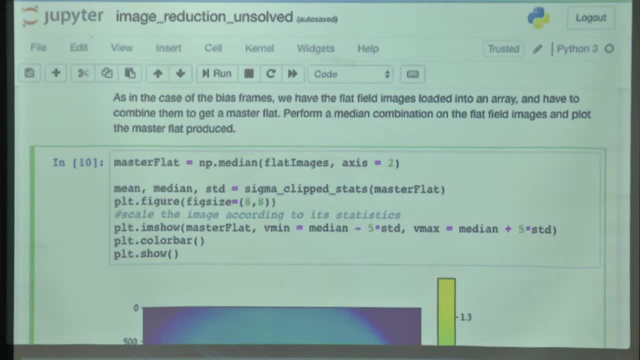 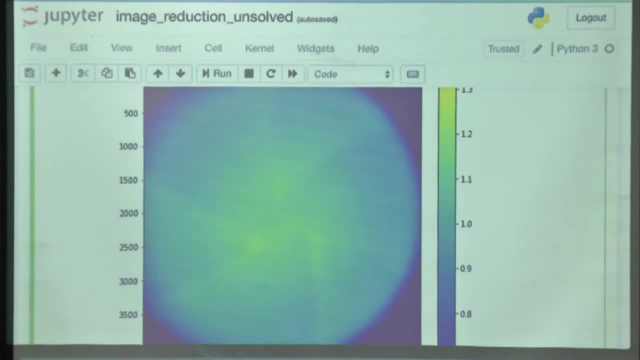 And median, combining it along one axis and plotting it up, So you should see something that looks like a flat field, that looks like this. It is because of the. this is matplotlib. it shows up at some scale, shows up at some not. Yes, Okay, How many people got to this step? How many people 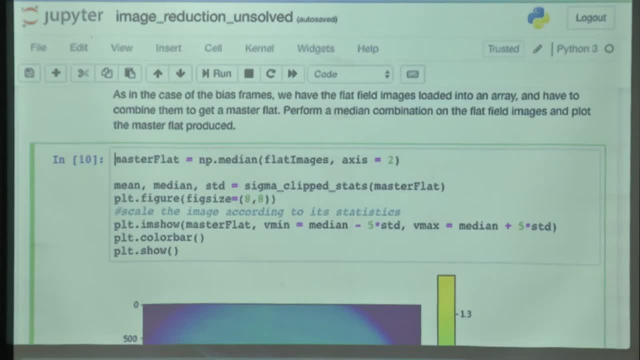 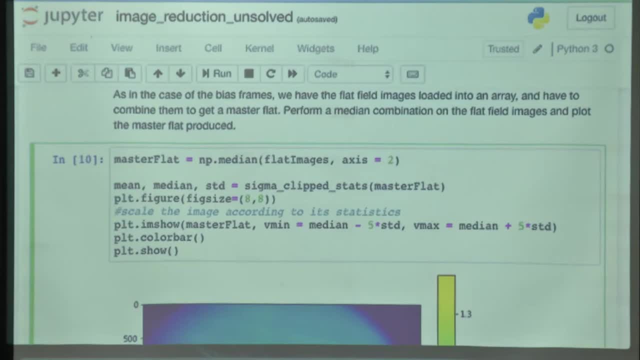 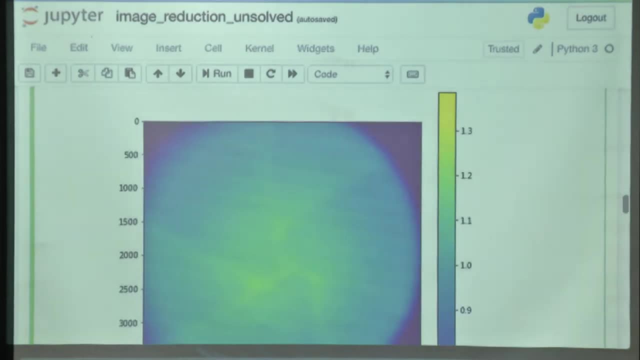 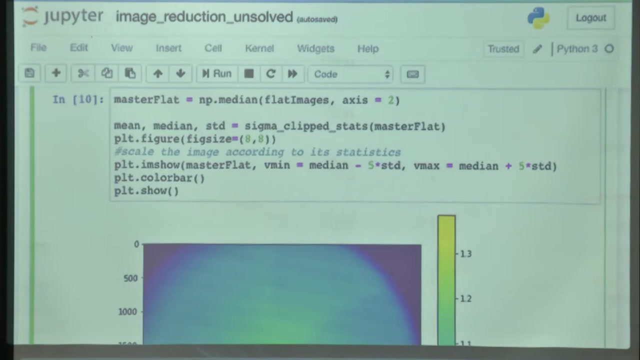 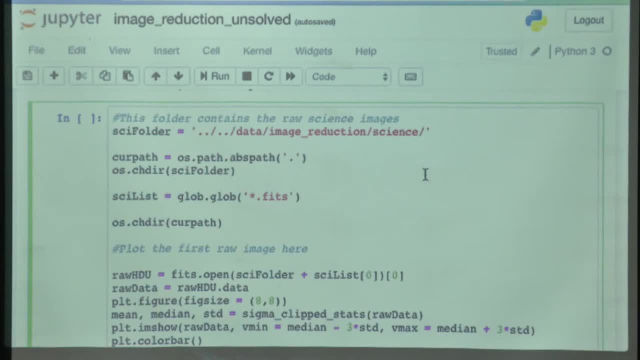 function is that I am automatically take it and have finished it if it is not produced and have finished it before. good, so what I am doing here again is: so this folder now has all the signs images that we want to process. good, so what I am doing here again is: so this folder now has all the signs images that we want to process. 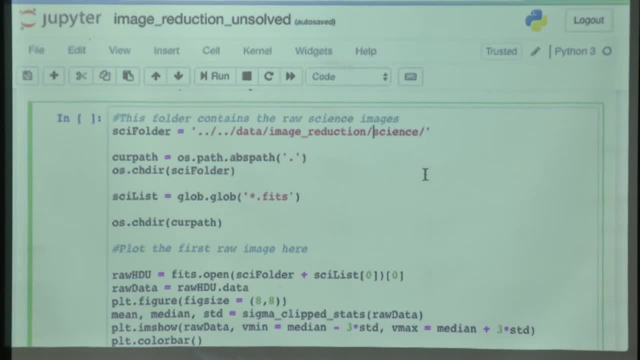 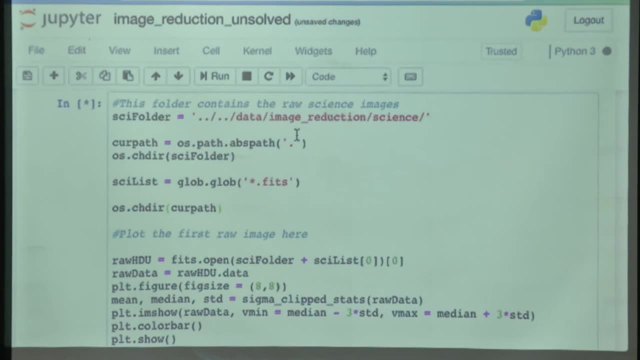 and what I am doing here is just continuously plating one of the signs images to show you what it looks like. this is a raw science frame. It has all the bad effects that were introduced by the telescope and the detector, but you should just have a look at it just to see what a raw image looks like. 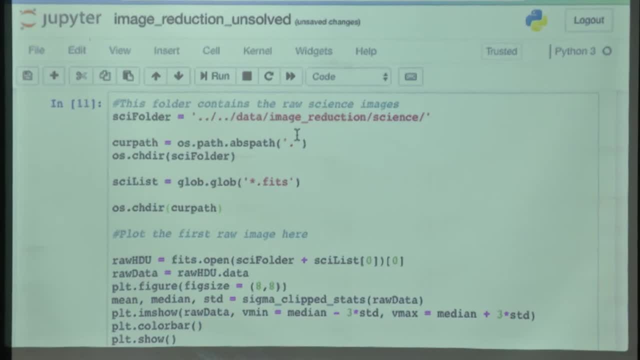 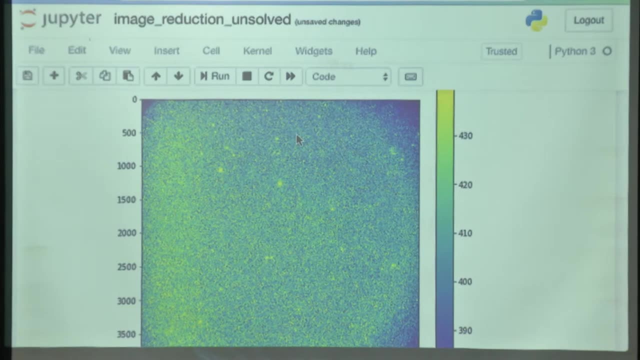 like So you can have a look at. it is just to see what a raw image looks like. Faced with all the different effects, they do seem enough and frames it's one. it's just one image. yes, So this is one raw image from the growth India telescope. 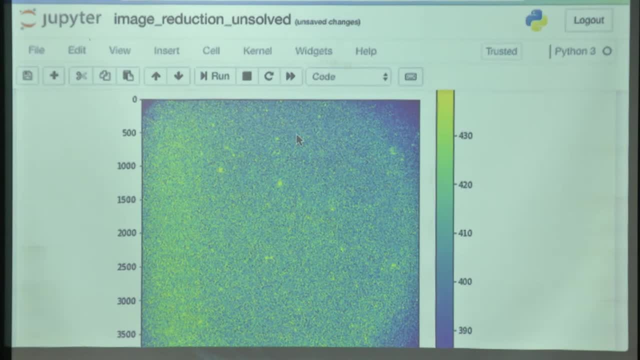 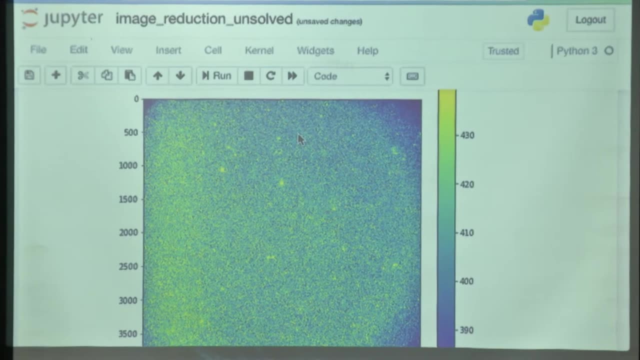 and, as you can see, the pattern that you should be looking for is this. you see this, this trend of increasing counts on this side. this is the bias that is introduced on top of the science frame, and you want to subtract this bias and divide it by the flat field to get what the 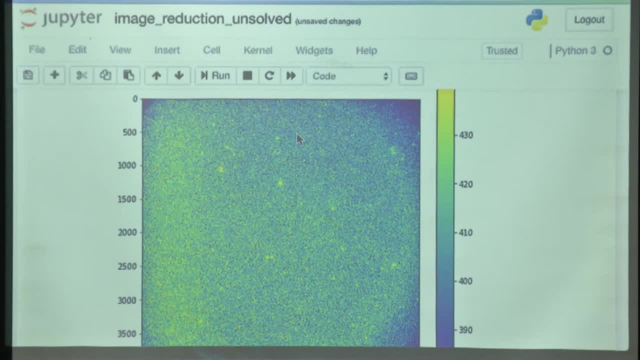 true brightness distribution on the sky is like: yes, yes, it should be approximately the same for the same detector, at least over some period of time. yes, it's a detector property. yes, different detectors have different patterns, possibly, yes, yes, okay, everybody able to plot this science frame, the raw science frame? raise your hand. if you were able to plot the science frame, anybody. 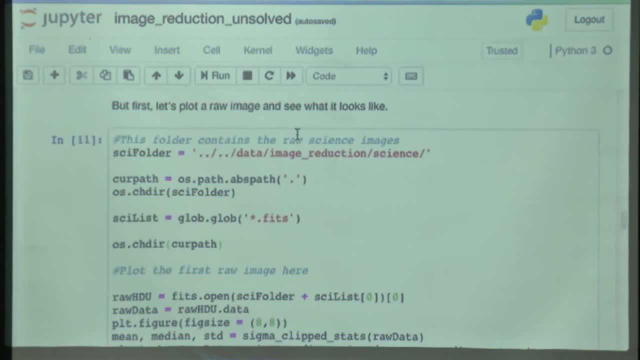 having major issues. I also, by the way, I will pull up this part just so that, in case you want to do that. So I will pull up this part just so that, in case you want to do that, look at the path. this is if you are using the docker. this should be the paths that you will. 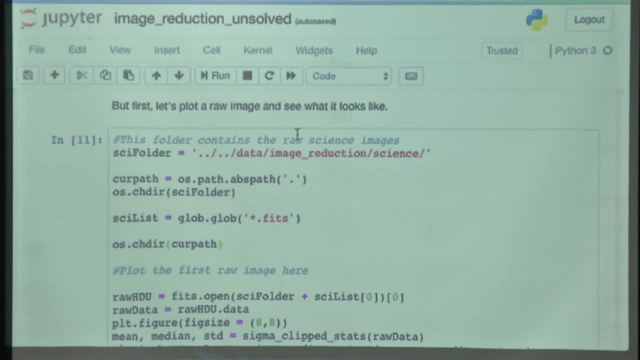 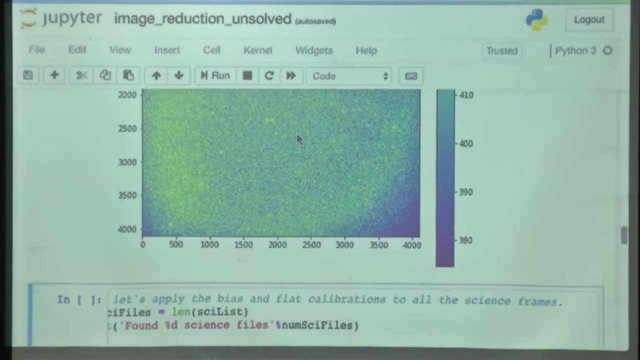 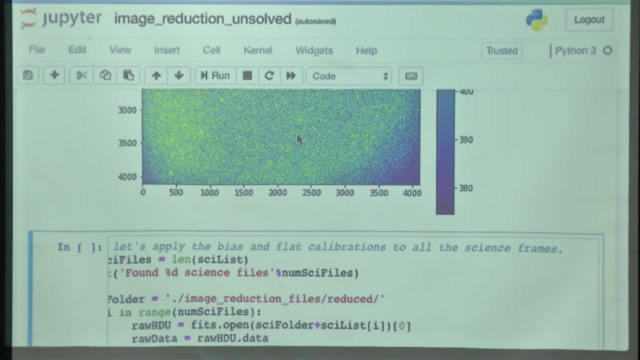 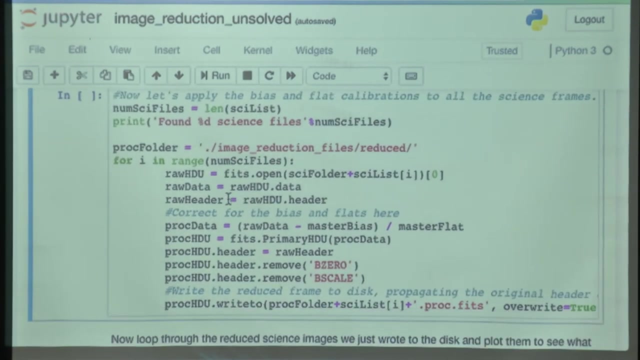 find the science frames in okay, questions issues, problems, okay. So if there are no major problems, I will go on to the next step, which is actually applying the calibrations that we have to these science images. So okay. so what I am doing here is I am looping over all of the science frames that 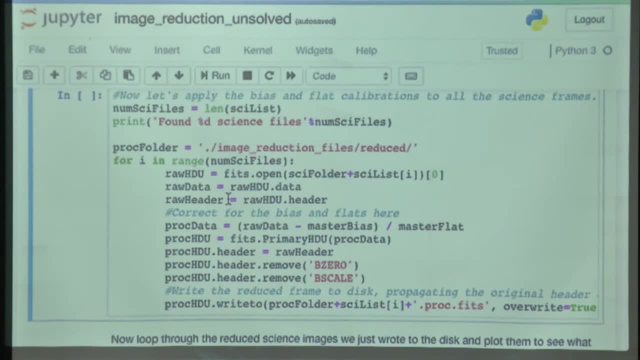 we just listed from the previous cell, and so this is the raw frame. I am reading the raw frame. this is the data. this is the header. this is the data. this is the header. and then I am producing a new array, which is the process data. where I am, what I am doing is I am subtracting the master bias. 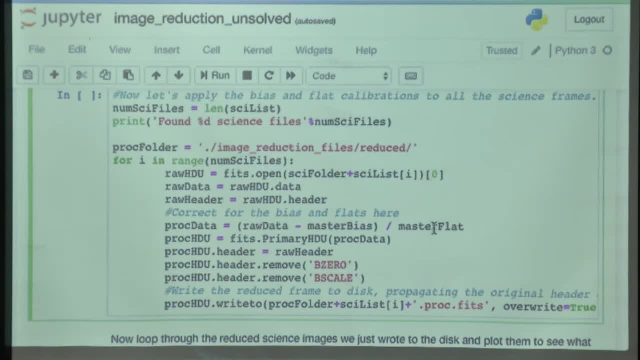 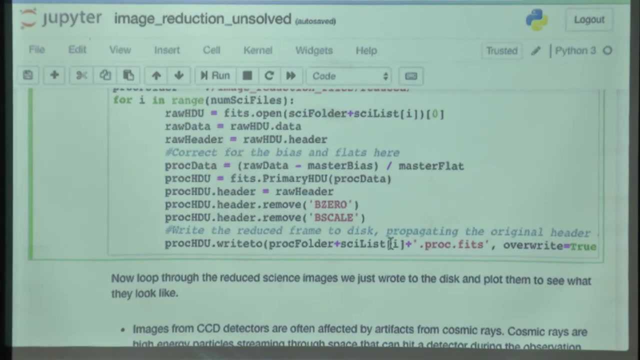 raw data minus master bias and dividing it by the master flat. this is exactly solving the arithmetic equation that we saw few minutes ago. I am subtracting the master bias, dividing it by the master flat, and then I am writing it to a file which is called basically the same name as the science file, with a probably outfits which just mean it's. 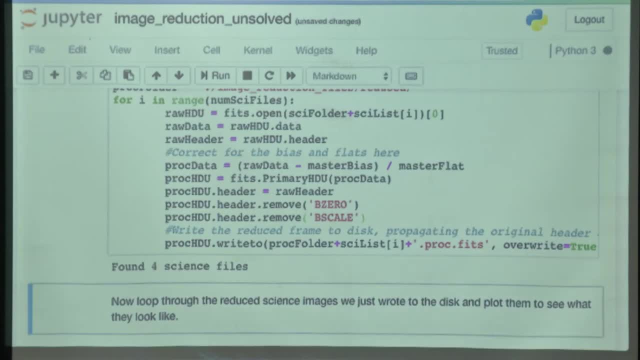 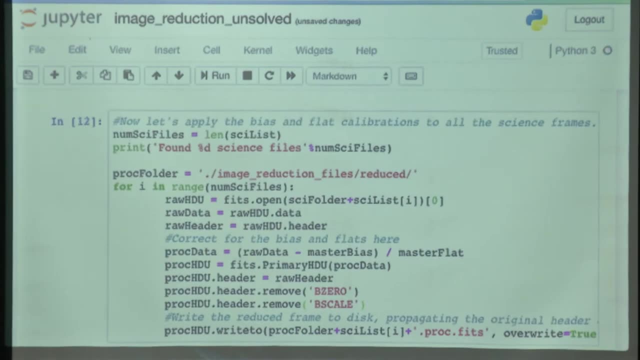 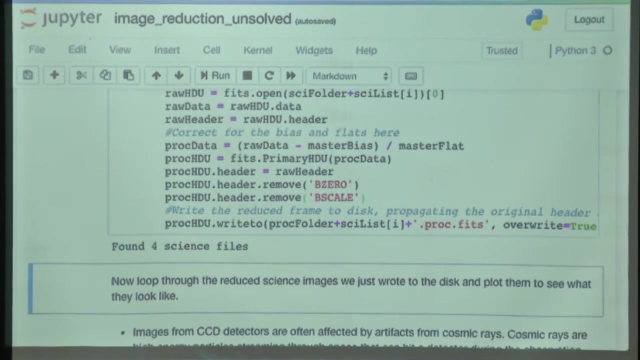 a processed file, So let me run this cell. yes, okay, so everybody able to run this cell. raise your hand if you are able to run this cell. okay. how many were able to run this cell so far? oh, yes, it should just be a. it's not really plotting anything yet, so it's just writing. 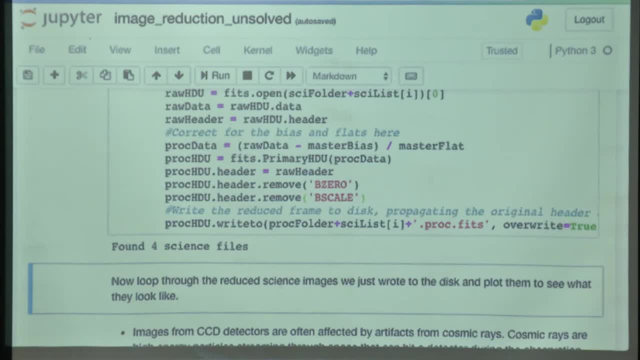 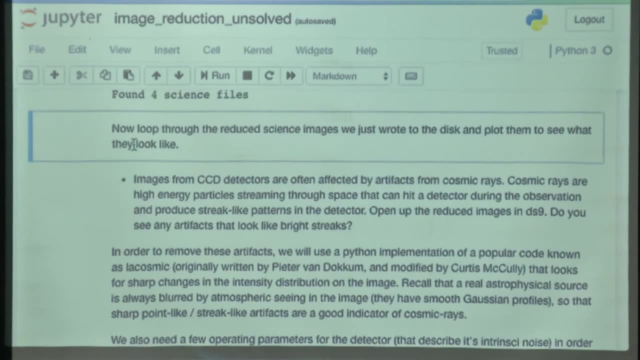 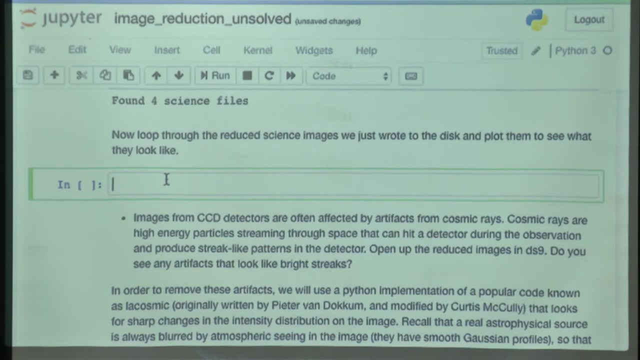 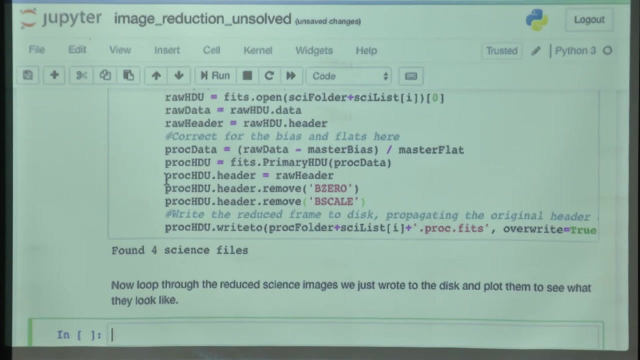 the files to the disk. is it just a moment? it means here that this is just a moment. sorry, what, what? oh, it should just be. dot proc, dot fits is just saving the file, as with the same name, with a suffix to it which says dot proc, dot fits means it's processed. 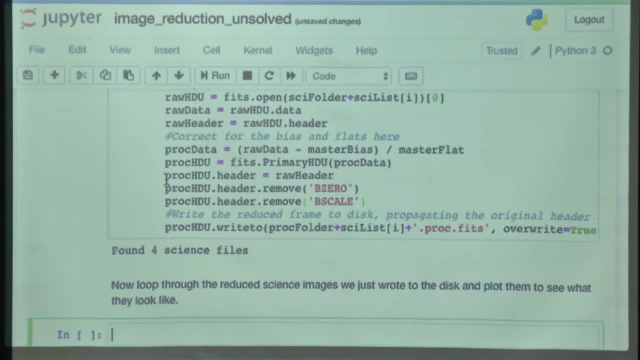 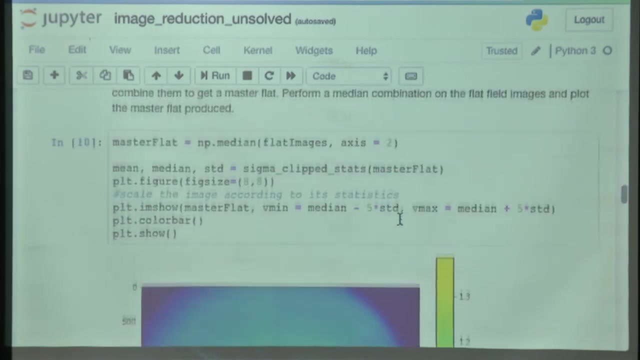 it's exactly this name. so it's the folder plus the name of the file, plus proc. dot fits axis. so we have. what we've done is we have loaded all of the flat frames into a three-dimensional lumpi array. so imagine it's like a stack of. so there's one image, another image, another image. 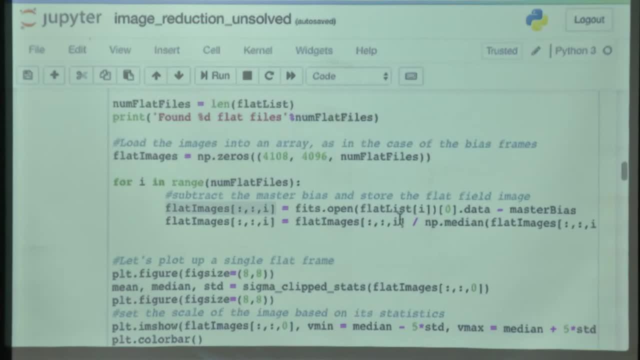 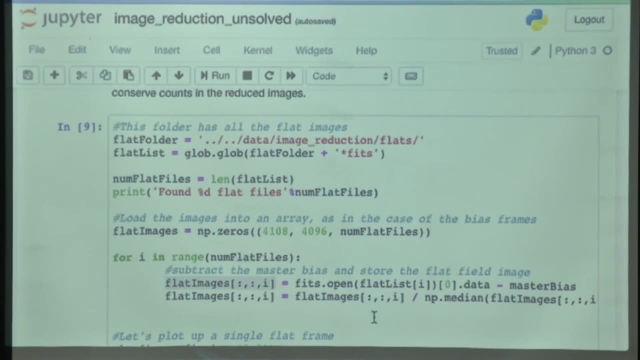 what you want to. so if you want to median- there are so many axis you want to- you can medial, and if you can att median along this axis, you can medial along this axis. you can median along this axis. what you want is a median along the image dimensions. so axis equals to 2 says median along. 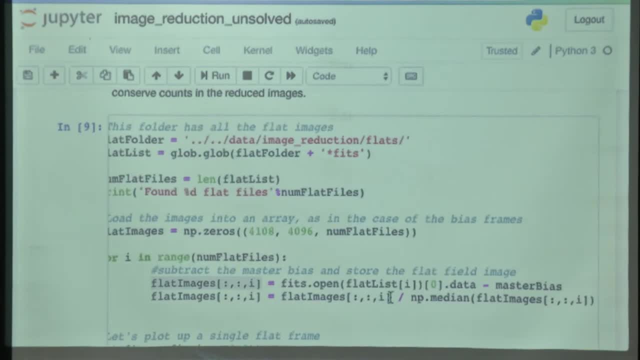 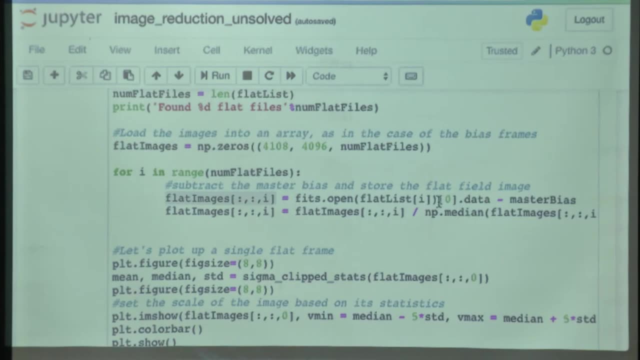 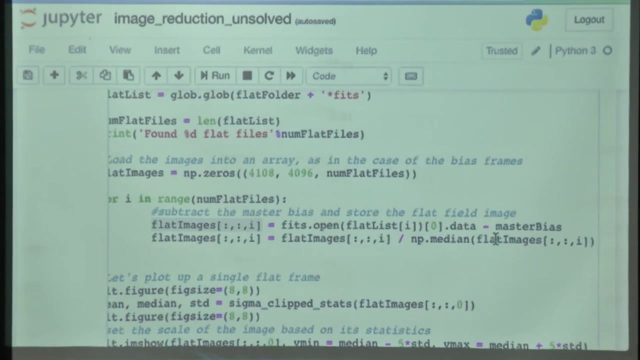 the image directions so that what you get effectively is a. that's because of the way I loaded the frame, so if you see, if you see this, so this says that I will get this view expression I. This says that for each layer in the array you are loading in the data into that specific 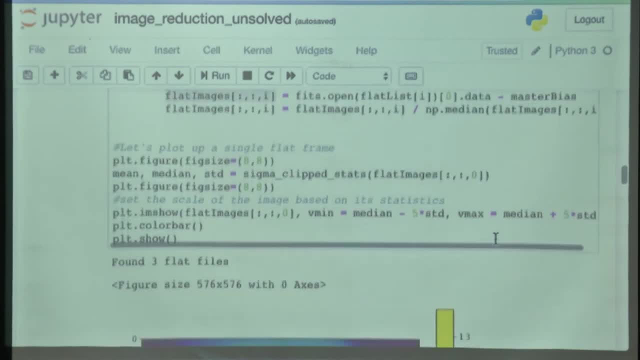 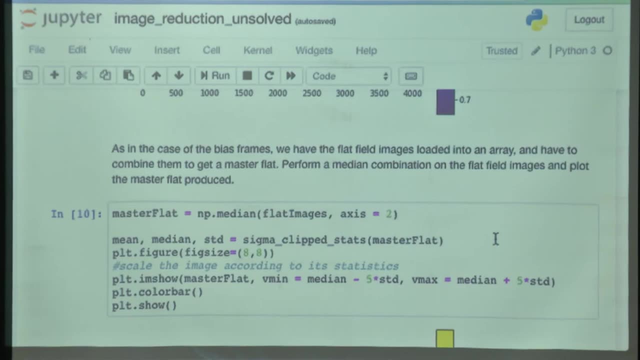 layer and I want to median along that layer so that what you get is a median combination along that axis. That is what axis equals to doing, because I think by default, NumPy will not median along the correct direction. You have to specify that you want to access along this, okay. 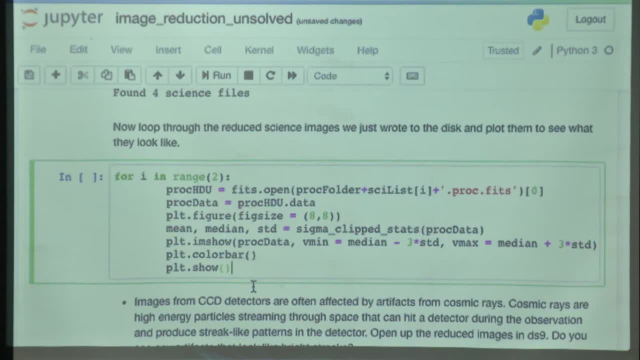 So what I am doing here is I filled in the next cell after that one and I am just plotting two of the reduced science files. So it should look something like this: You should first open the data, load it with AstroPy in an array and then plot it. 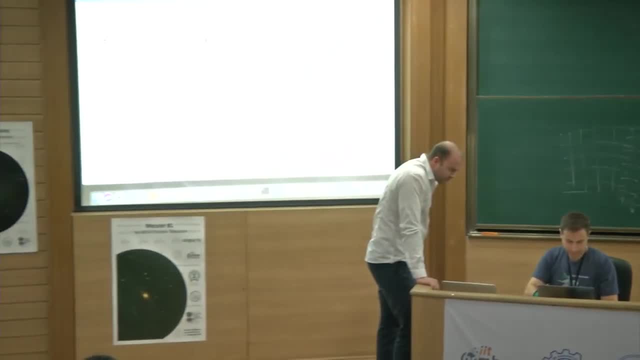 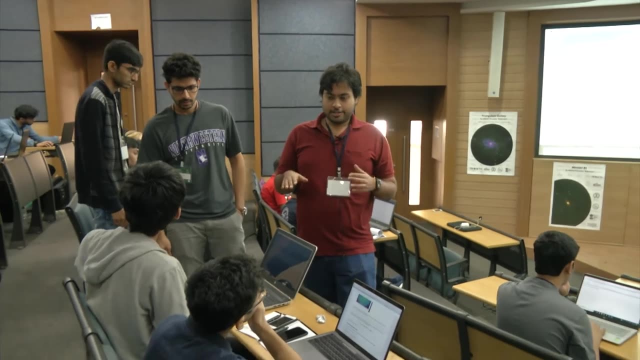 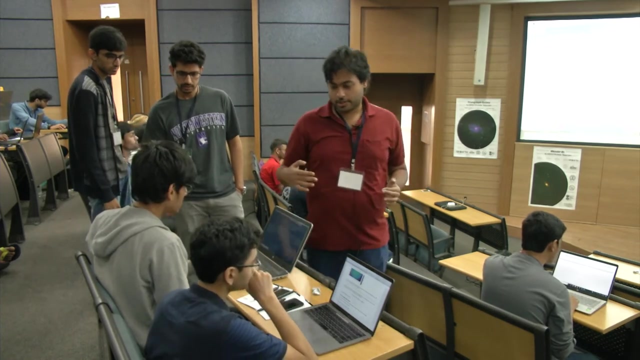 Yes, yes, it is an electronic offset in the detector that is always there. yes, No, flat is the variation in the sensitivity of the pixels, So each pixel may not be this- have the same sensitivity to incoming light. and we want- and that is because that is why it multiplies onto the science image, whereas the bias is. 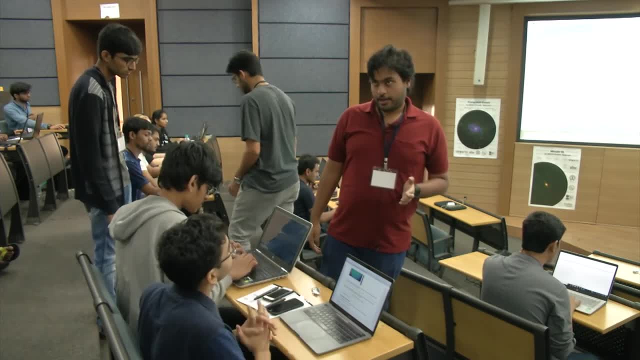 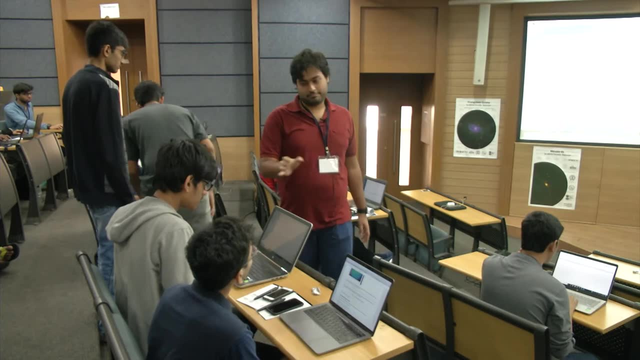 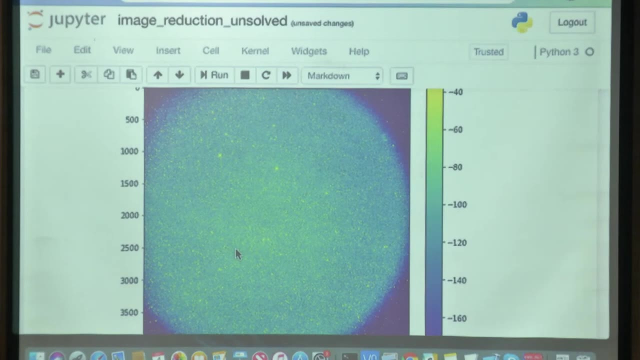 an offset that you want to remove. Usually the natural background light is not as much of a problem in the optical, In the near infrared, things are different, but in the optical it is not really something you should be worried about. yes, Alright, So it does. 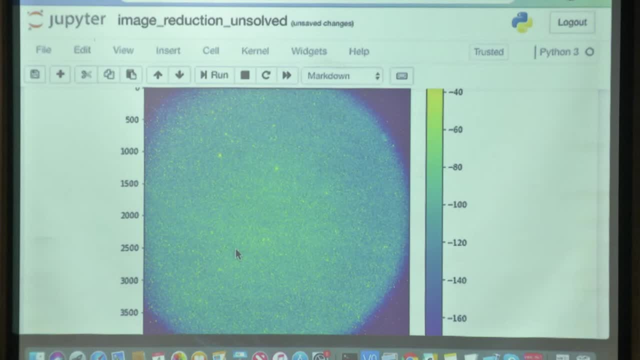 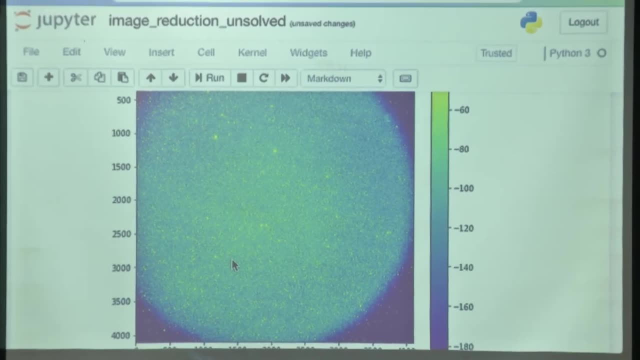 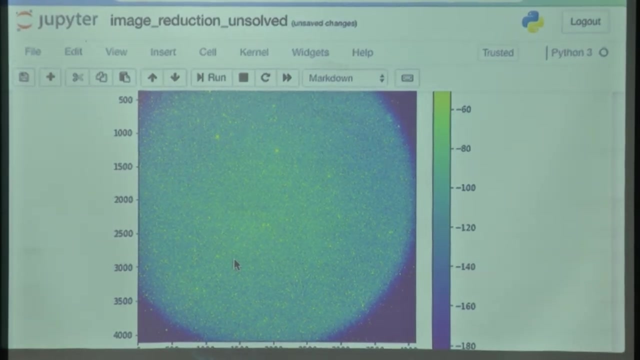 So this is what the reduced image should look like. How many of you were able to run some version of this to get an image that looks like this? Okay, I see one hand. okay, So the thing that you should notice is that the offset variation across the image is now. 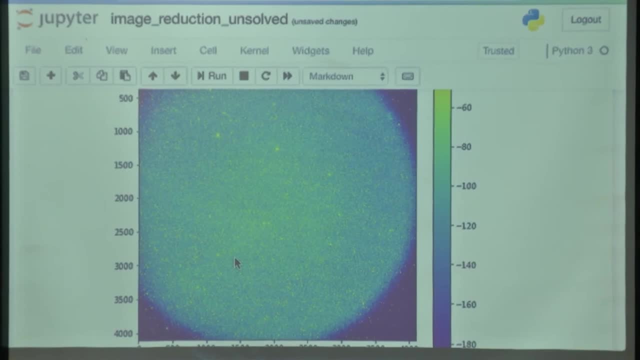 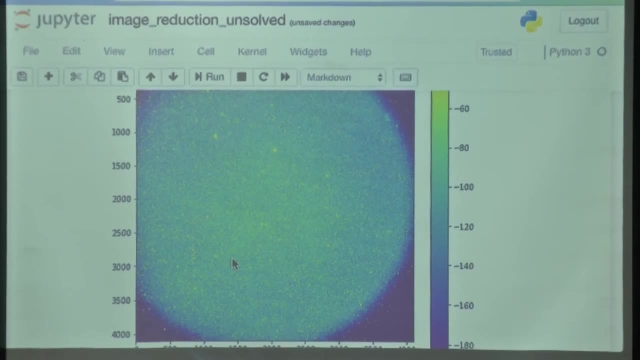 not there. It is more or less plain. the edges of the image are still dark and that is because of vignetting, Where it is just that the telescope optics does not allow light to get into this part of the image because it is such a wide field. 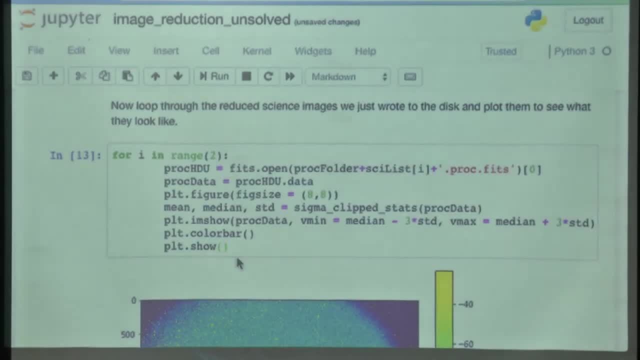 Okay, so just so you know, this is pretty much all there is to image reduction. This is what the true image of the sky actually looks like. The subsequent steps, depending on how much we time, how much time we have, the subsequent steps are just refining on this image to remove more and more artifacts from the image. but 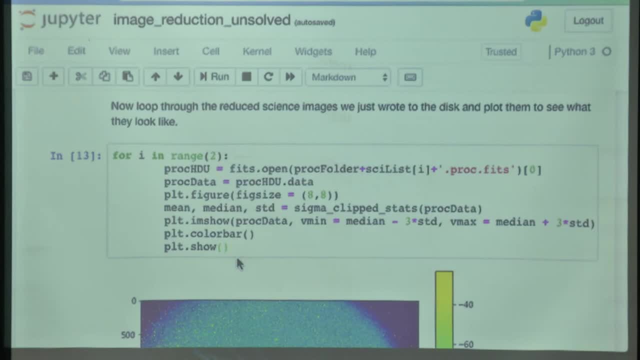 in principle, Yes. All you need to get science data out of This is a reduced image, a true image of the sky that does not have any of the artifacts that were introduced either by the detector or the telescope. I have not stacked anything yet. 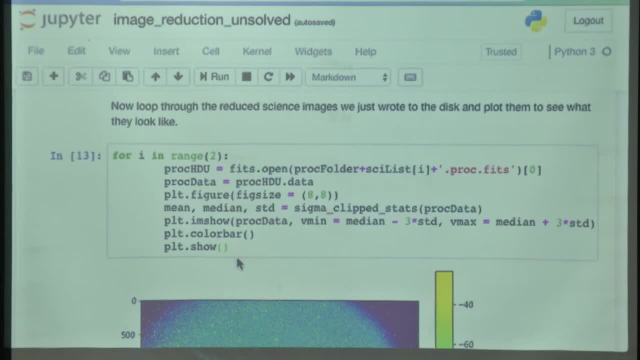 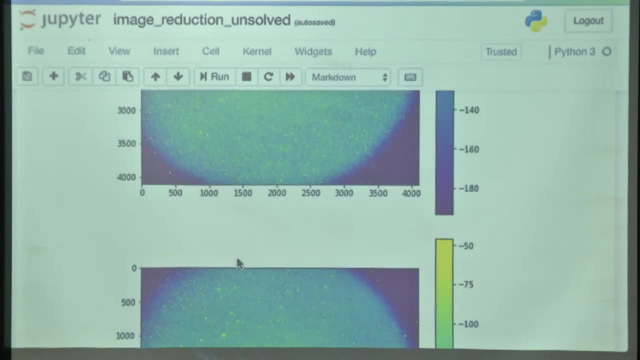 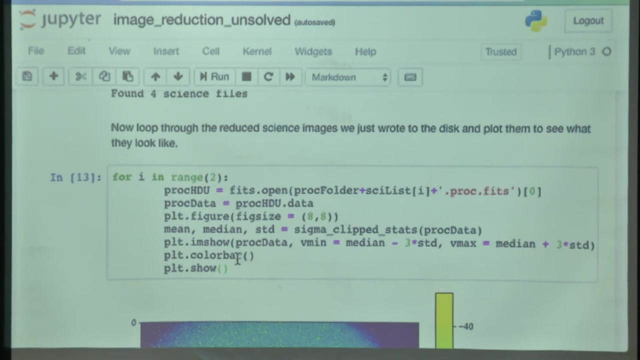 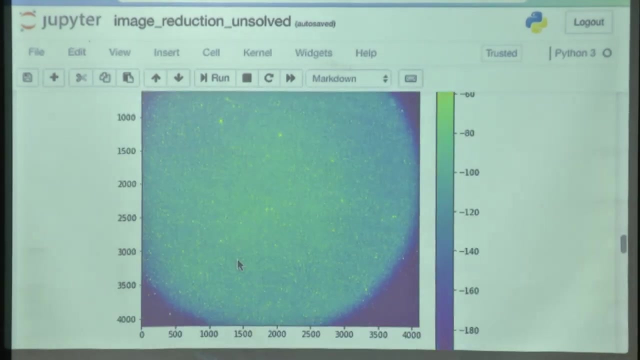 These are individual science images. Oh, so there are two. I just plotted two of these images. oh yes, So this is what I am. So I am Plotting the file that was written to disk and then I am plotting it. Okay, so so far we actually have reduced images. but the next thing that I had in my module 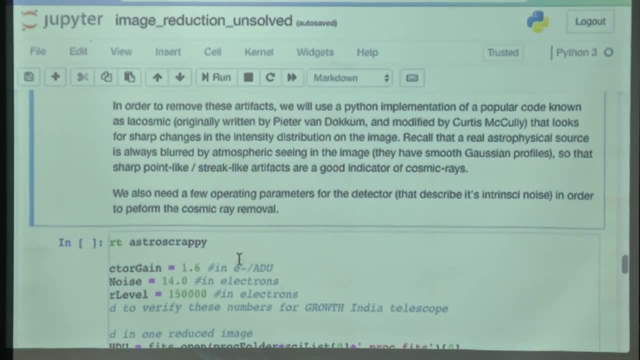 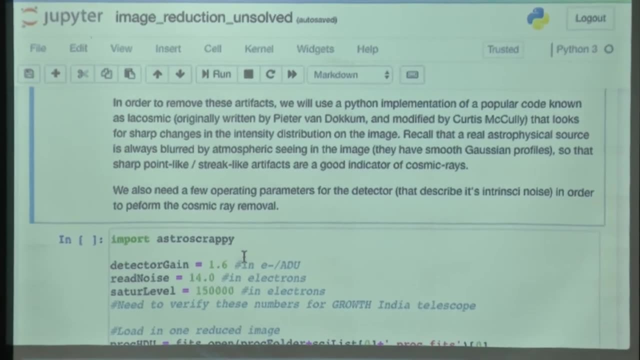 which is probably going to be the last thing that we do is let us see. So the next part of the module is to remove cosmic rays from the image, where the idea is that during, in the duration of the exposure that you had, there were probably some cosmic 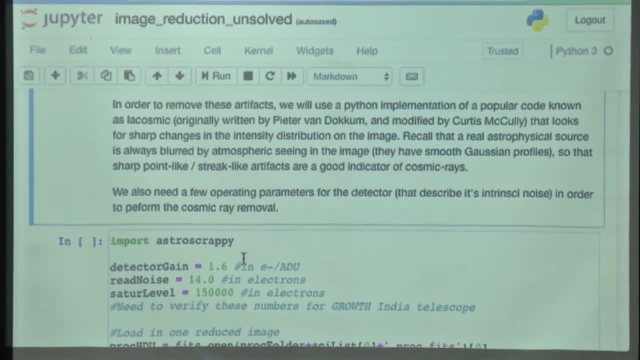 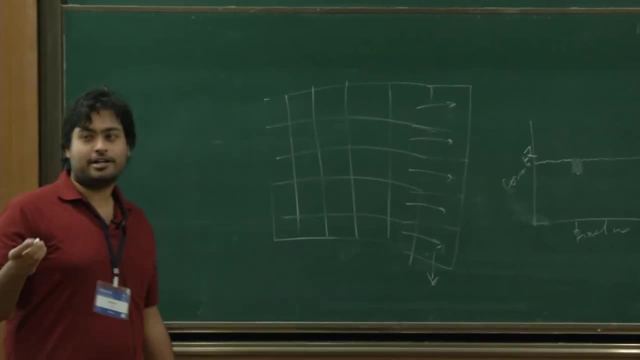 rays that hit the image And the way to identify them is to look for very sudden variations in intensity in the image. So imagine you have, so a normal star, a normal. if you look at a normal star, then a star always has a shape which is reflects the PSF, the point spread function of the image. 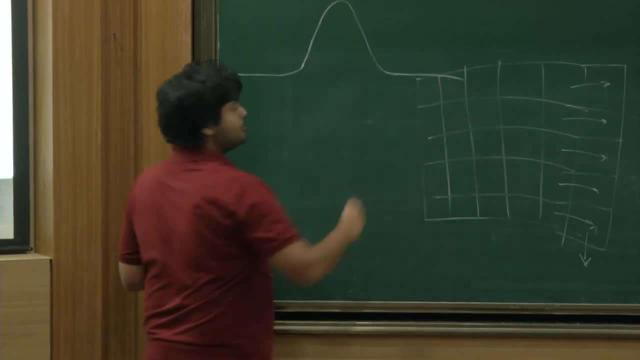 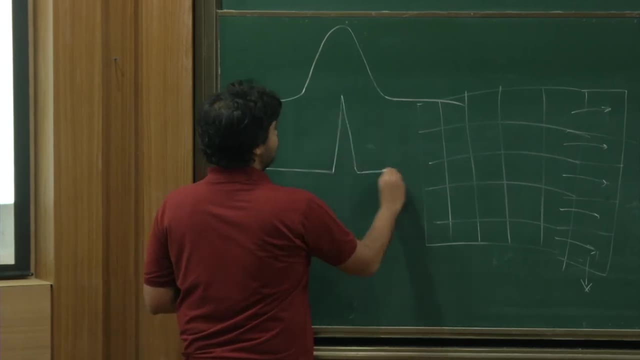 So you would get a smooth variation that looks like this: if you take a cut across the star, A cosmic ray looks very different. A cosmic ray would typically look something like this: It's a sudden delta function that just hit the detector And 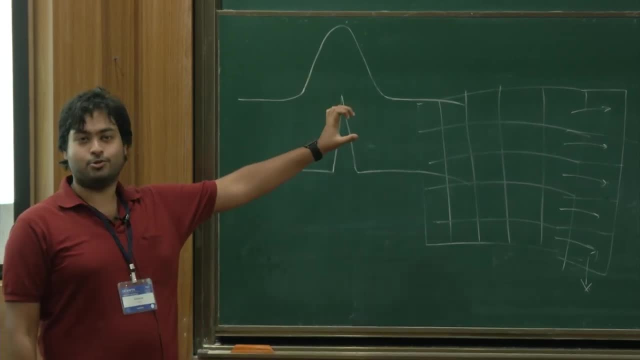 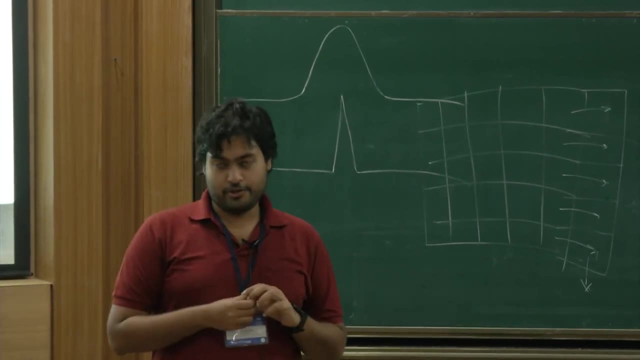 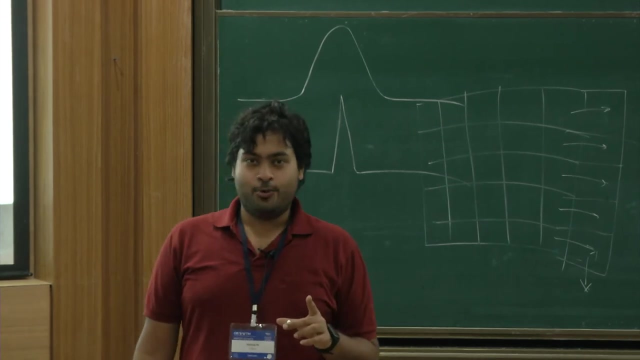 It's. It's this change, it's this difference in the shape that allows you to identify what are cosmics and what are real stars and out there. there are actually quite a few implementations of these algorithms that deal with cosmic ray rejection, and I wanted to use one of these. 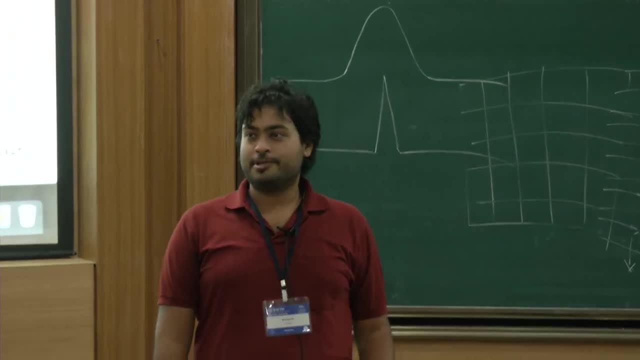 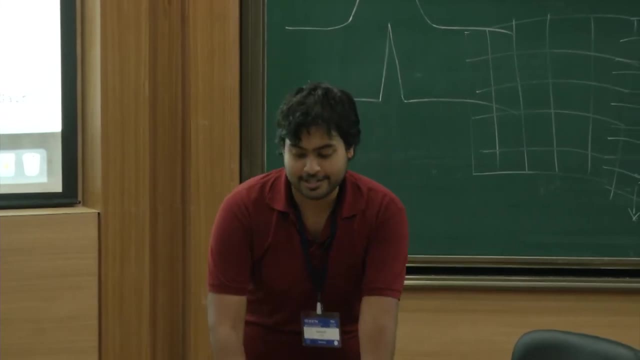 which is called. So this is a fairly popular cosmic ray removal algorithm. It's based on LA cosmic, which is which is a routine to detect cosmic rays, and this is a That we just installed before the start of the session. this is a python implementation. 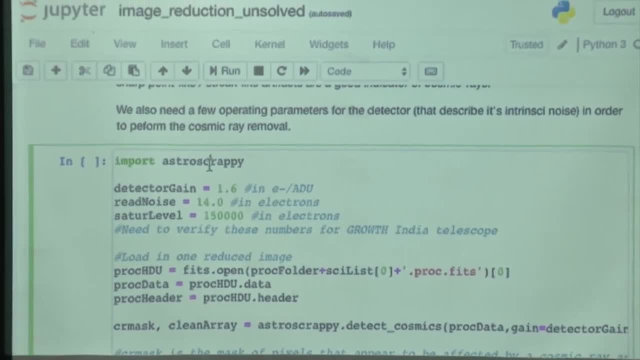 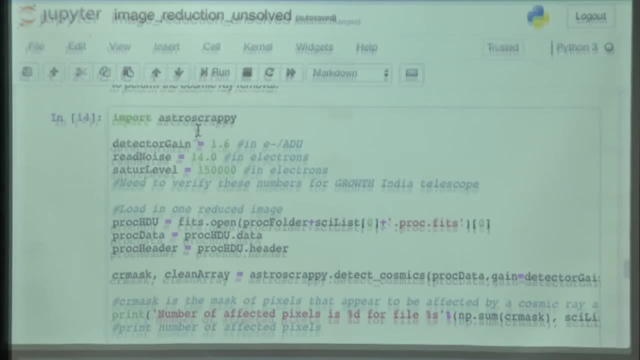 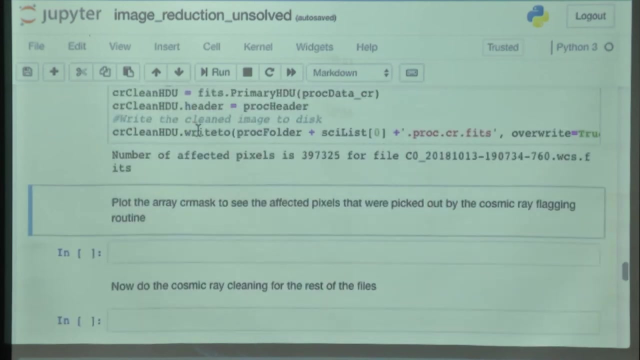 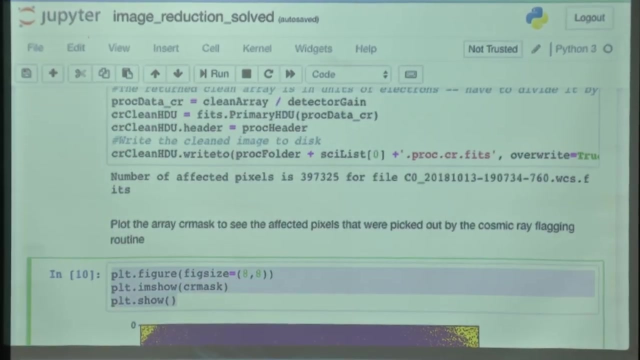 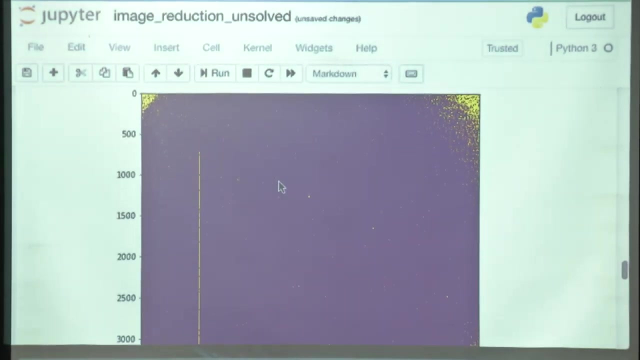 of this same module, which is LA cosmic. So let's see, So if I run this cell, Okay, so I just wanted to show what a typical cosmic ray mask look, looks like. so So, even if you haven't been able to run it yet, but I think you should just take a look- 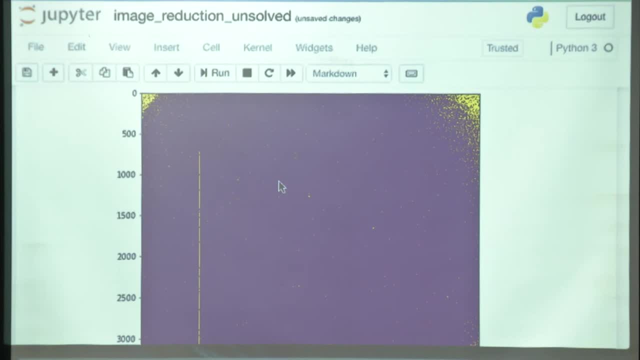 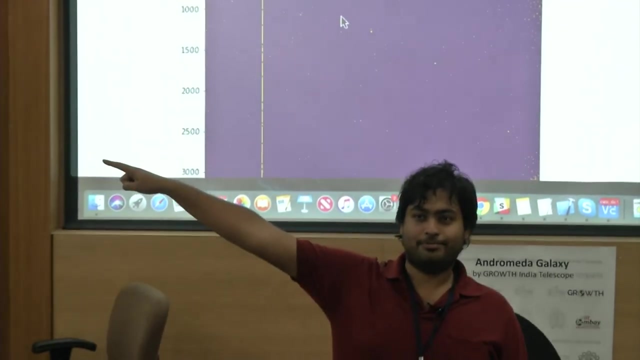 at what a typical cosmic ray mask looks like. so what you have here is basically the same image, but what this algorithm did is to detect things that look like this, and it created a dot wherever it found those things. Yes, Okay, how many people that got to this step? okay, there were, okay. so I think I'll end with 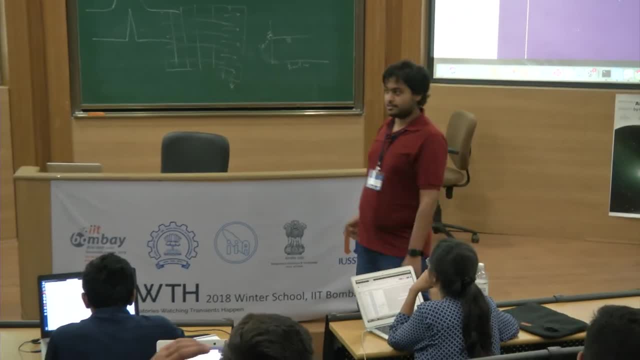 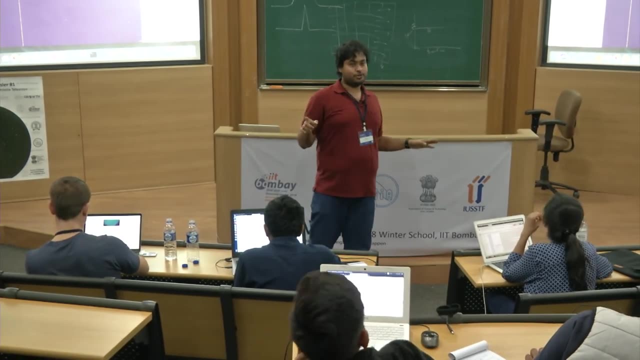 astrometry, I think. yes, five more minutes, yes, so I okay. so, even so, we can talk offline if you are not able to get to this step. but I just wanted to show what astrometry is about, because that's another important part of reducing an image. 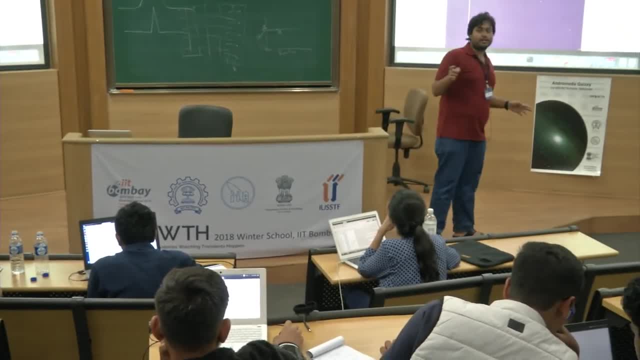 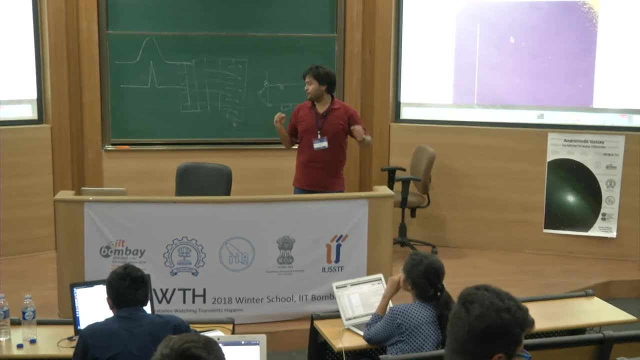 So, as Anupama said, astrometry is all about figuring out where the image is on the sky And Effectively. Effectively, what it turns out being is matching patterns of stars. so imagine you have the idea is that suppose you have stars in your image that looks that are randomly positioned. 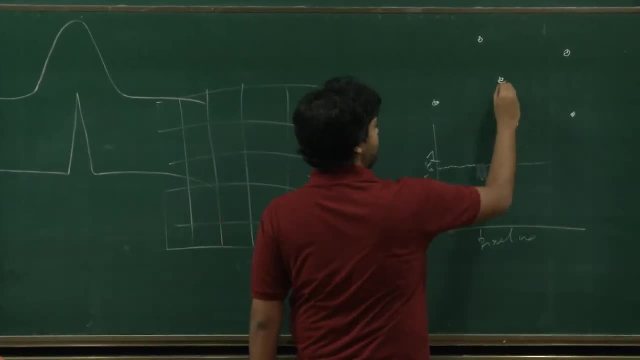 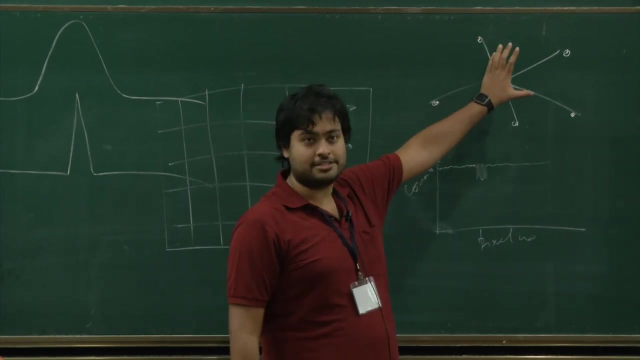 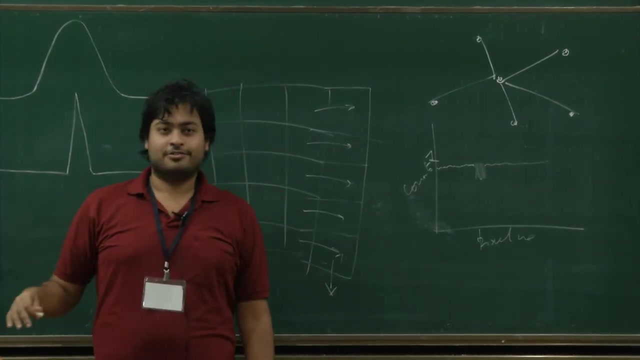 like this and you ask the question: what if I join these lines along stars? and then you want to match these, these pairs of stars, to a catalog of known positions. so imagine you have a separate known catalog of known positions. this could be so. we live in the era of big. 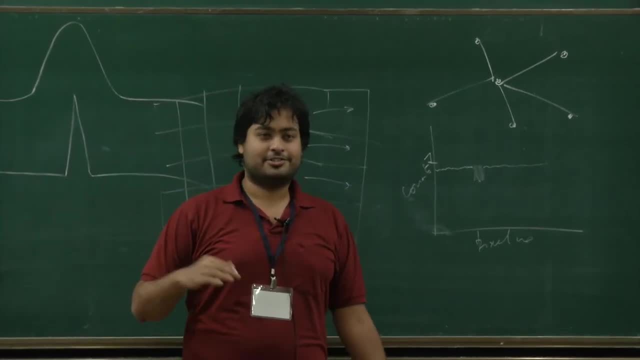 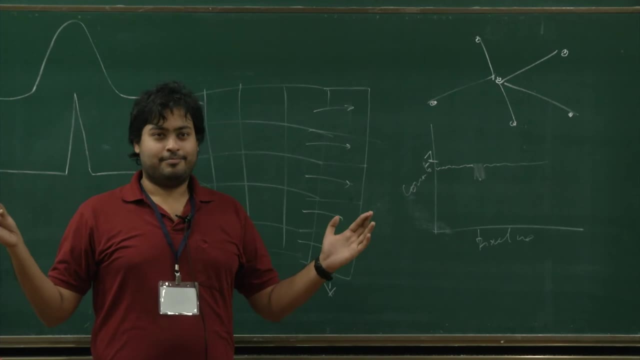 surveys, It's very likely that the position that you're observing has already been observed by some other survey. so you take that catalog. so this, this other catalog, will also have the same stars because it's the same part of the sky. so the idea is that this other catalog also. 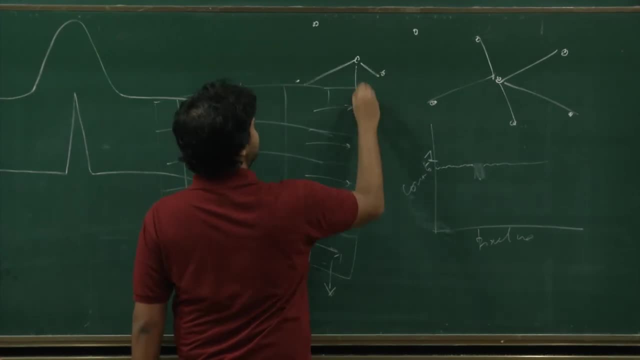 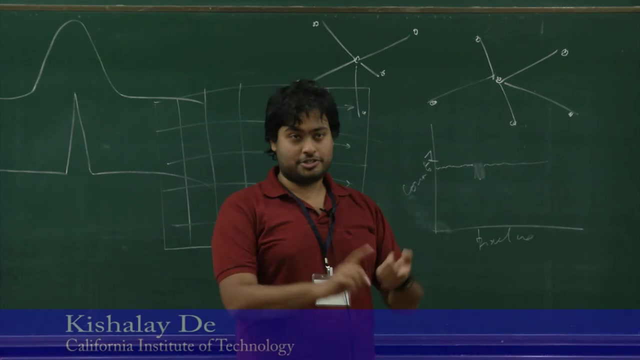 has the same pattern on the sky and you ask the question: does this pattern that I see in the catalog match this pattern that I see in the image and, if it does, you actually know what is the position of the image, what is the orientation of the image and what is the? 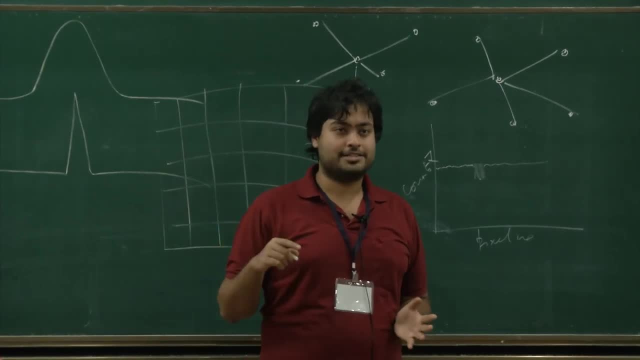 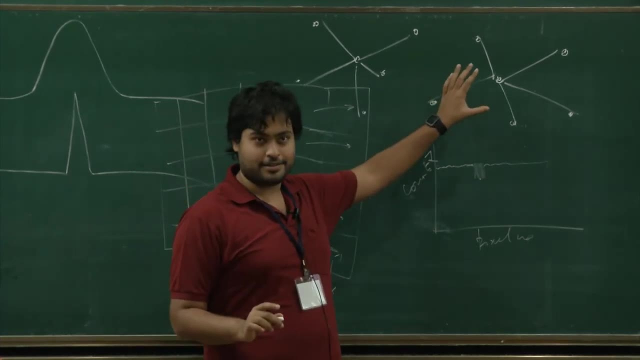 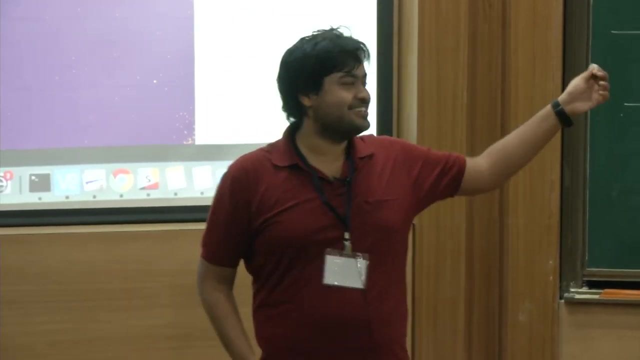 scale of the image In terms of you know how many pixels corresponds to how many arc seconds on the sky, and that's, that's all that is there is to astrometry and basically all astrometry software solves this problem. ah, yes, I mean they use more complicated. I mean these, this is just lines, but it can. 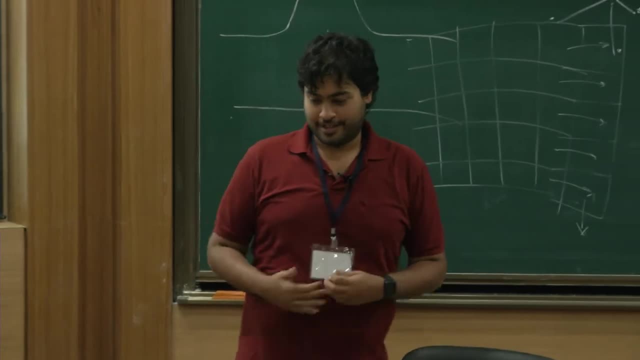 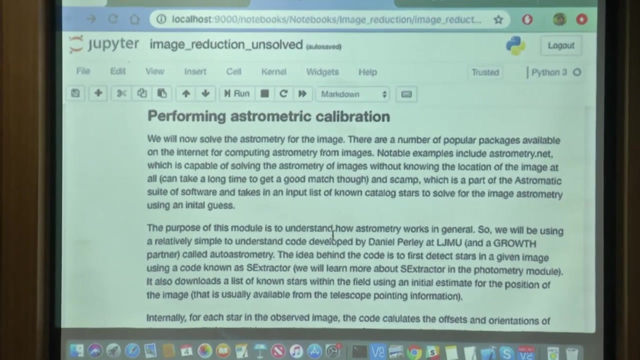 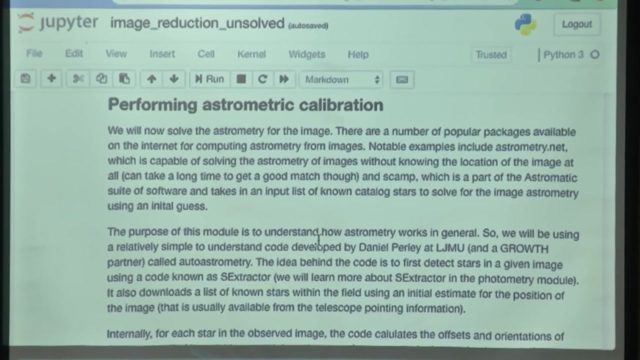 be quadrilaterals, triangles, with anything. ah, let me show you so what I'm doing in this module. I'm using a code that was written by Dan Purley at Liverpool, which is a fairly simple to understand code, which is? it effectively solves this problem, which is to match stars. 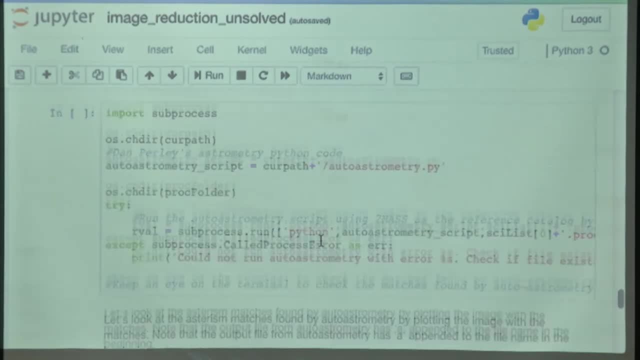 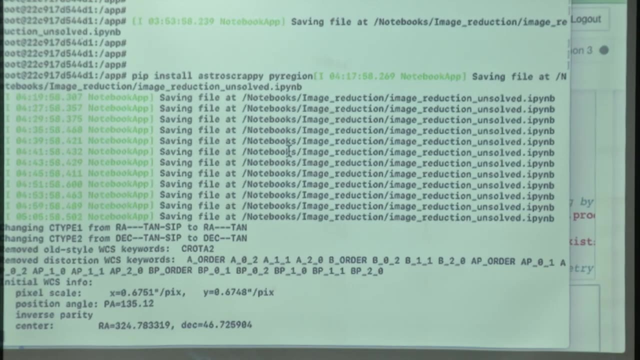 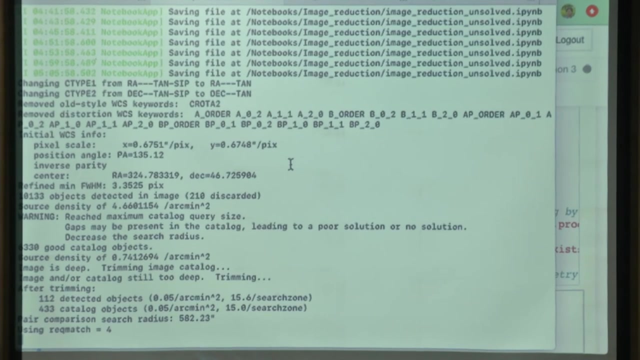 in the image to stars in the sky, and let me just try showing what this looks like. ok, so. so if you keep an eye on your terminal while you're running this, you will see that it's it detected few objects in the image and it it's matching it to a catalog of known images. 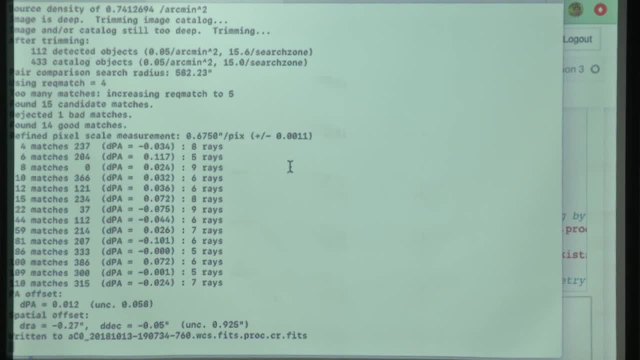 in this case It's matching it to the two mass catalog, which is whole sky, near infrared. and what it did was it it found so many matches between the stars in the image and stars in the catalog to figure out what is the position and orientation of the image with respect to the catalog. and 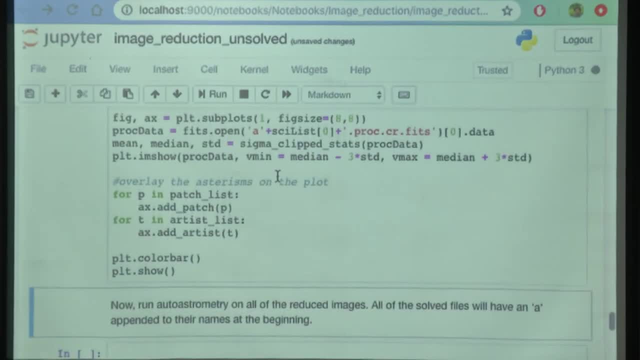 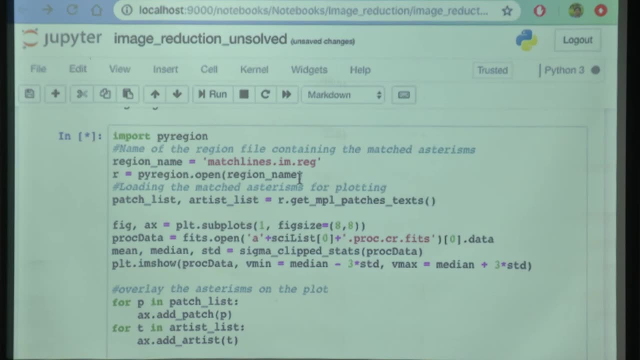 just to show you what matches it found. this is the. just give me a moment, So what? so what this code also produces is a list of matches, which is list of shapes that it found while trying to solve this problem right here, and once it loads up, ok. 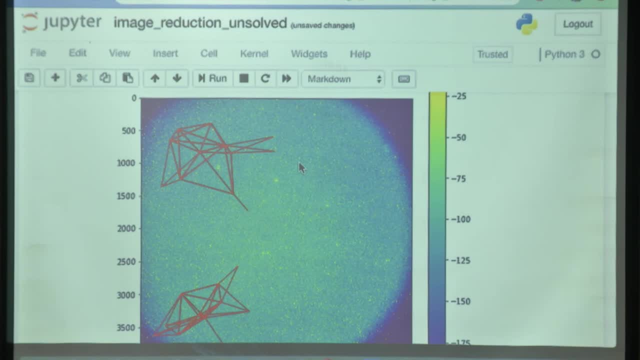 so these are the matches that it's found in the image. so what it did was that it asked to mass give me the positions of the stars. that is that you know about, and these are the positions of the stars in my image. can you match any shapes? could be triangles, straight. 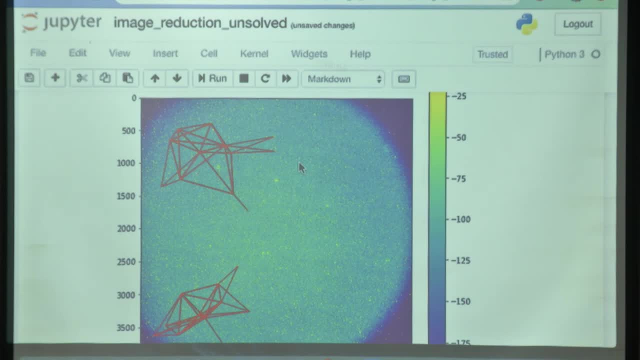 lines, quadrilaterals, really anything, and does this look like any of the matches that you see in the catalog? And these are the good matches that it found? so you see, there are this. so this pattern is called an asterism. it's- this is a name. it's asterism where you effectively match. 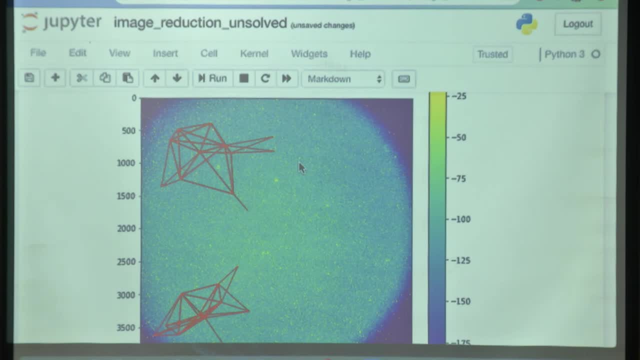 patterns in the image to a pattern in the catalog, and these are the good matches that it found. So once you have this kind of a, an identified pattern on the sky, you immediately know what is the position of the image, because you know the position of these stars, you know how big.